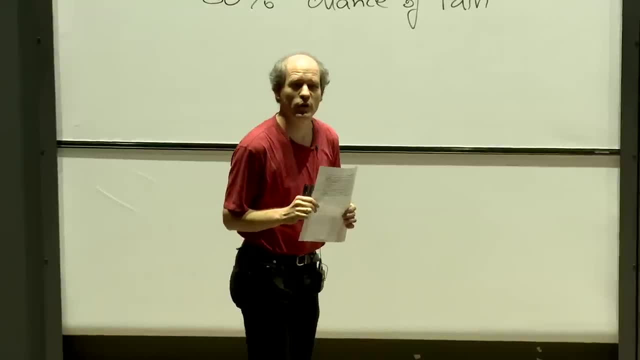 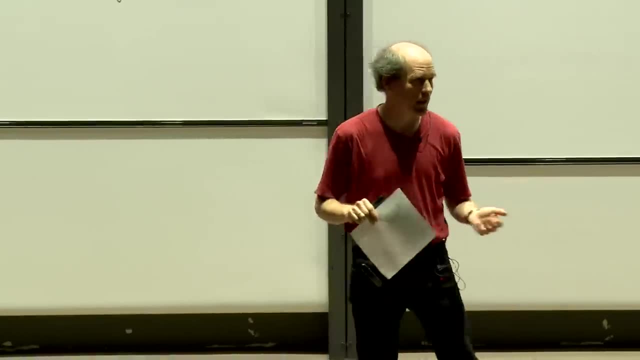 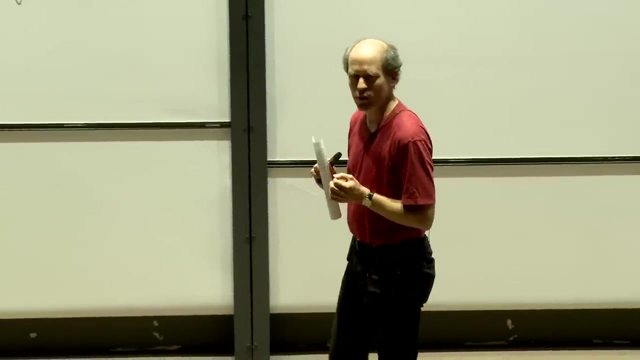 it to rain for 80% of those days. That's an explanation that's useful to interpret the weather forecast and to behave accordingly. Get your umbrella out and don't get wet Now. mathematically speaking, that's not a very good explanation, though, is it? 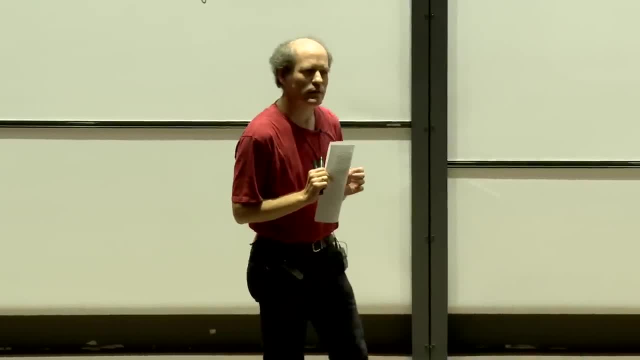 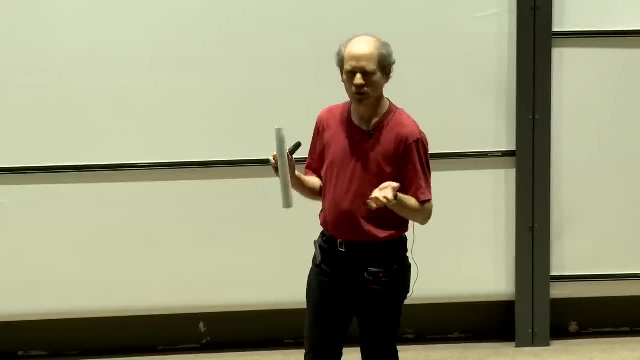 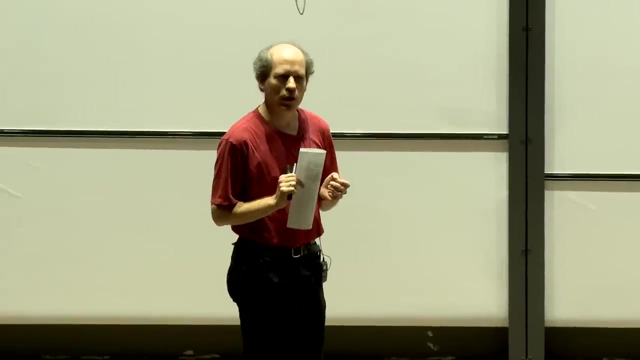 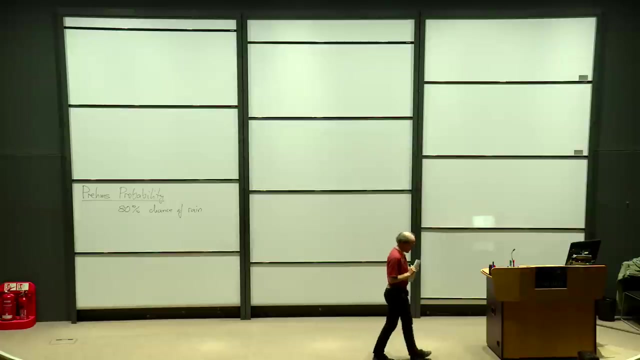 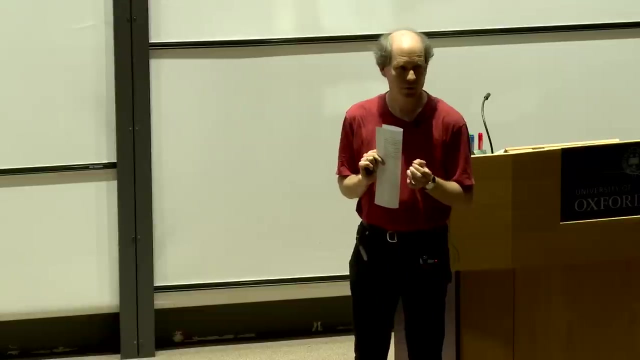 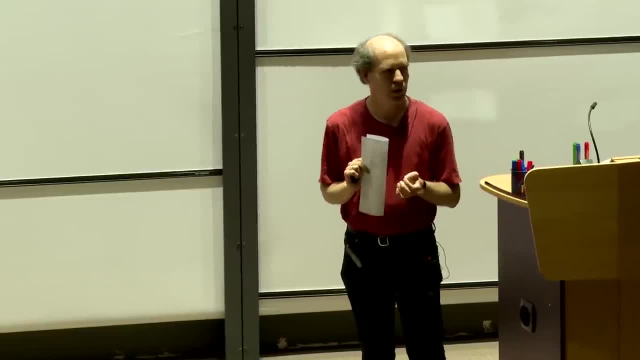 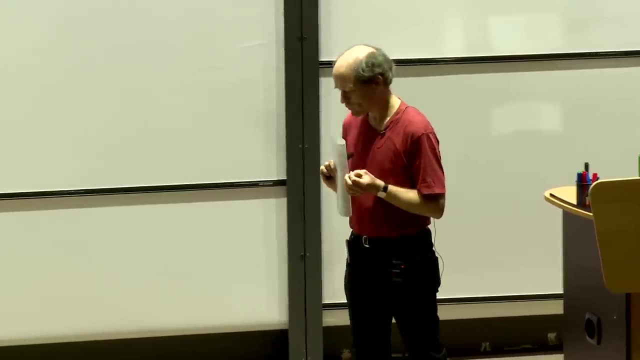 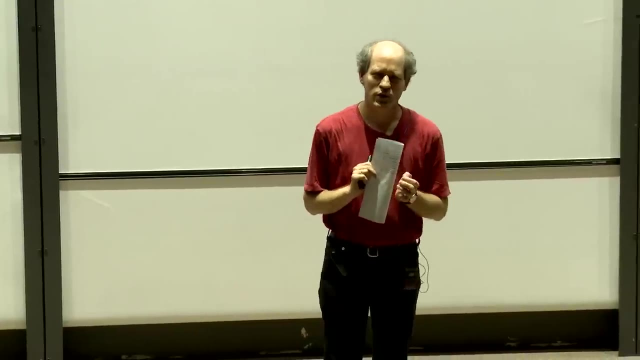 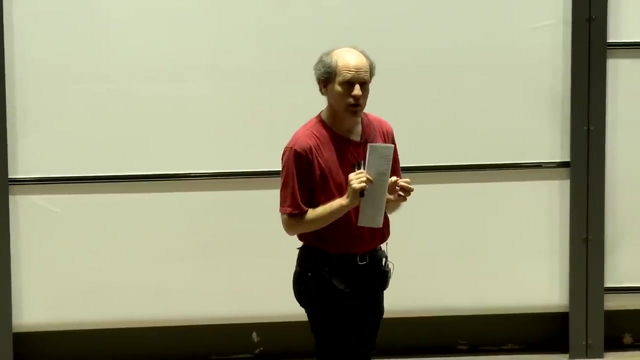 things that we don't fully understand or fully observe may appear to be random, and it may be useful to use probabilistic modeling. there's an 80% chance of rain. how can the Met Office make such a statement? is there evidence? is there data that they've collected? yes, there is. they've got lots of weather. 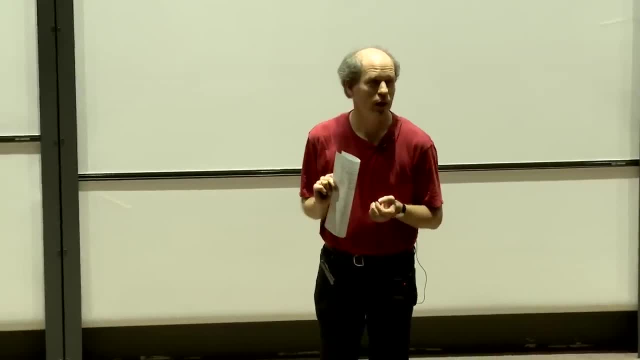 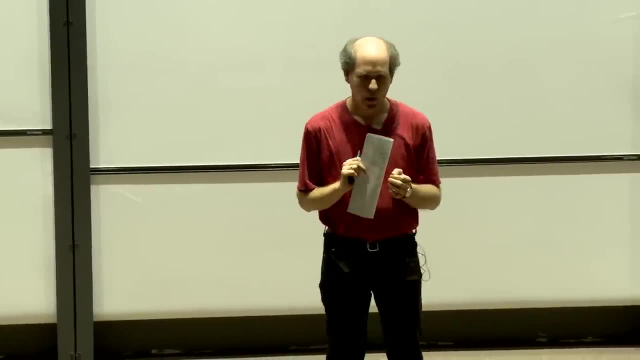 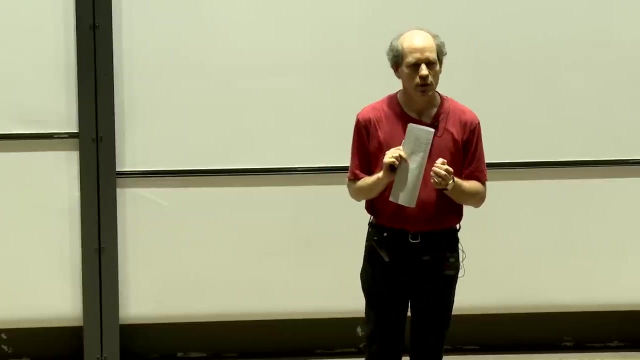 stations all over the country, they have devices on planes, they have weather balloons that they launch and they get a lot of data and they analyze the data. these are statistical questions. right, they can predict the future based on the past. it's a rather sophisticated statistical application because there 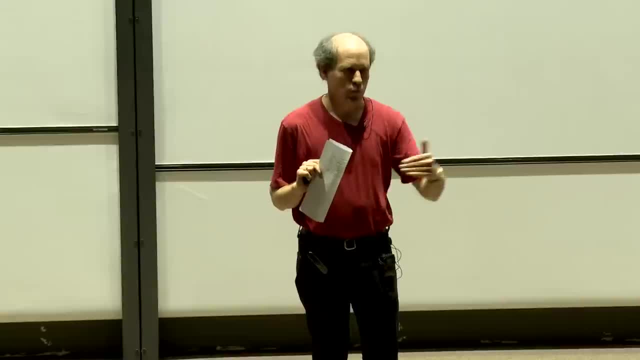 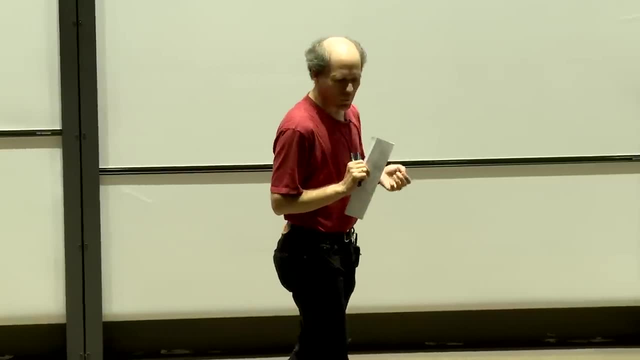 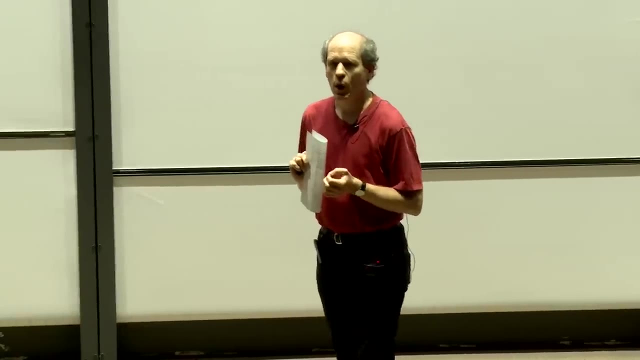 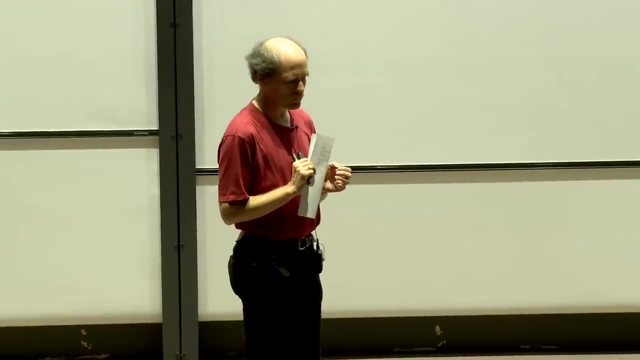 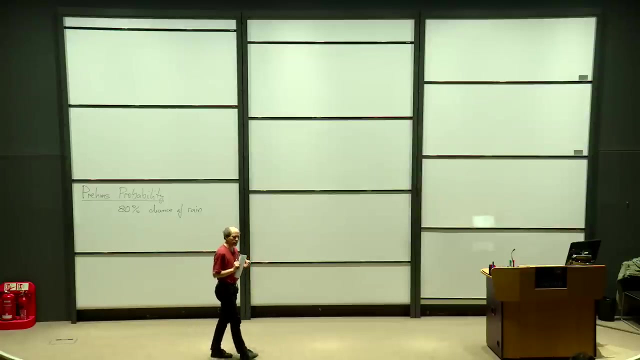 is a lot of data involved and also because predicting is harder than just describing, and about the future in particular. well, you have to have to use some modeling, probabilistic modeling, in order to to make sense of the situation that you want to predict. now, this particular situation about weather prediction is of 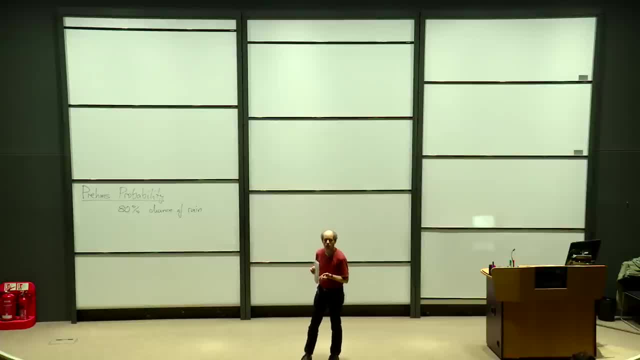 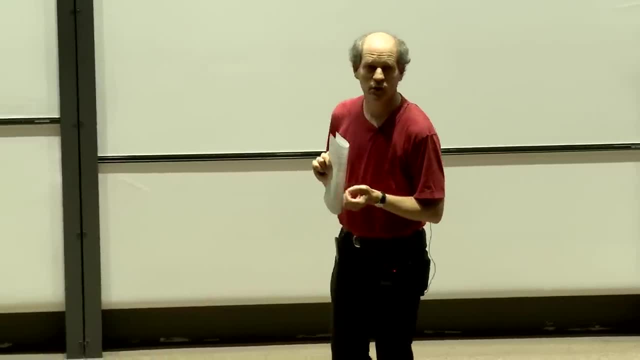 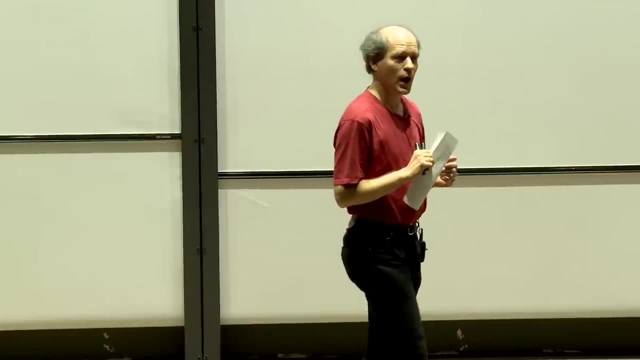 course, only one of many applications in the real world where probability is and features- and it it's really- across a whole range of different settings. some very elementary, like tossing a coin, rolling dice and a well shuffled hand of cards gives gives rise to some some interesting probability questions. others: 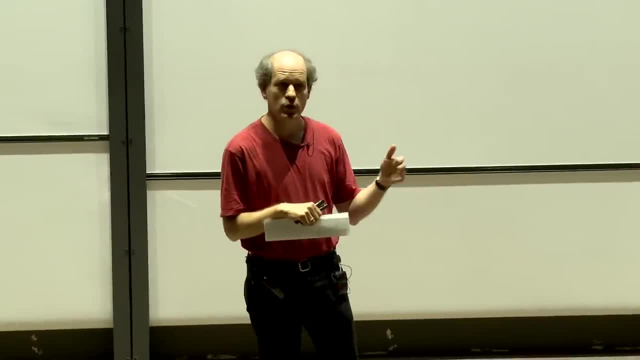 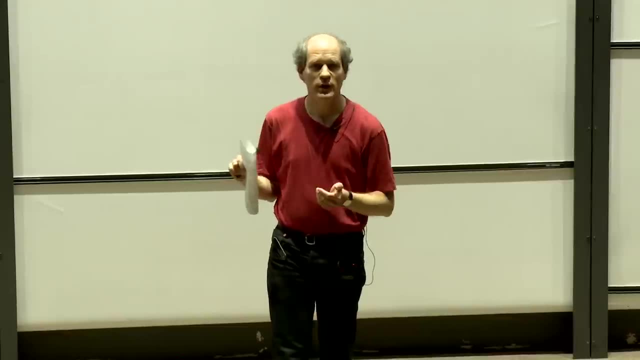 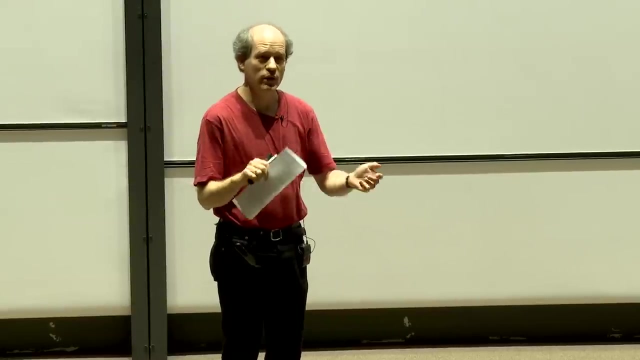 are much more sophisticated, and weather is one of them, but there's also financial markets or genetics in in many ways that are from how are all the species related? how? how does the genetic evolution happen, in terms of DNA that gets passed on and that changes, and both on a big scale between species, but also on a small? 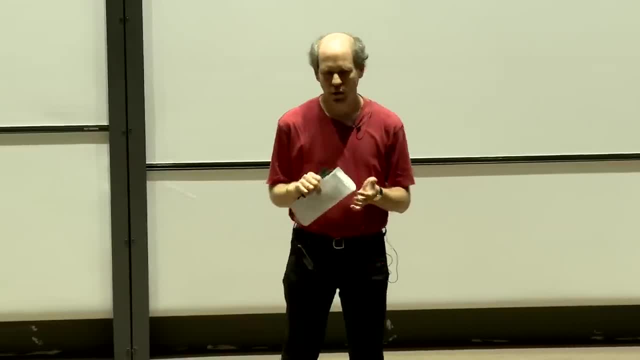 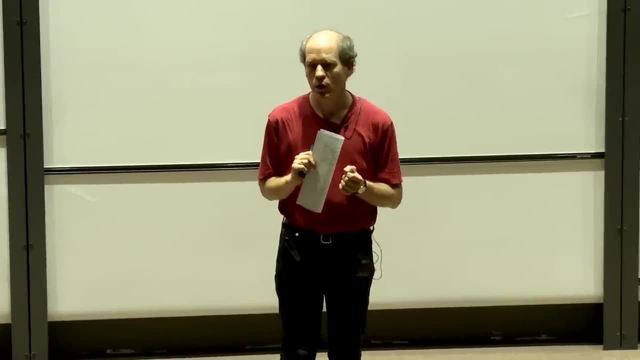 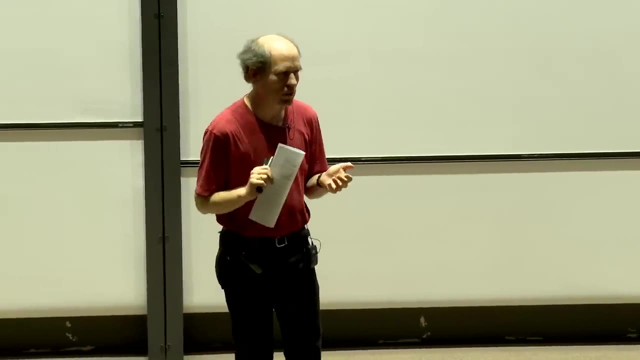 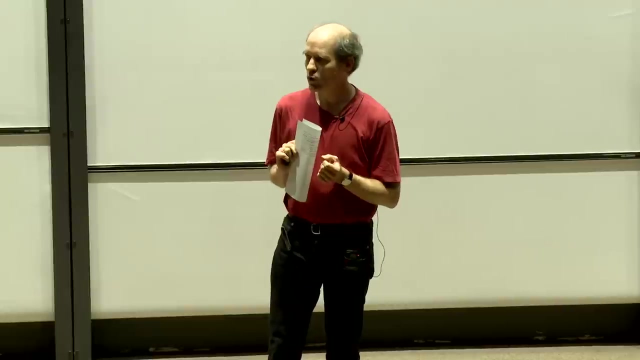 scale from your parents to yourselves. so there is a lot of randomness involved in that process and there is scope for probabilistic modeling in each of those areas. it's some of it genuinely random, others maybe not so genuinely random, but we can still perceive it as random and make useful random models that that help us. 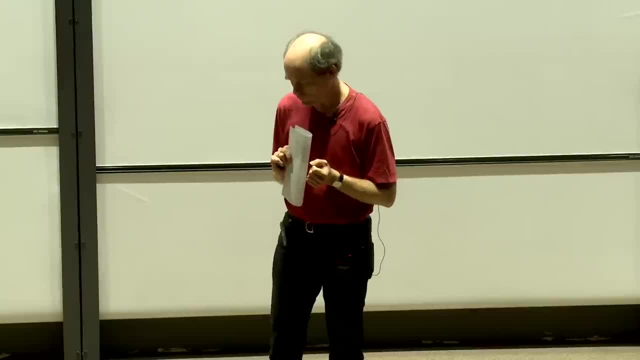 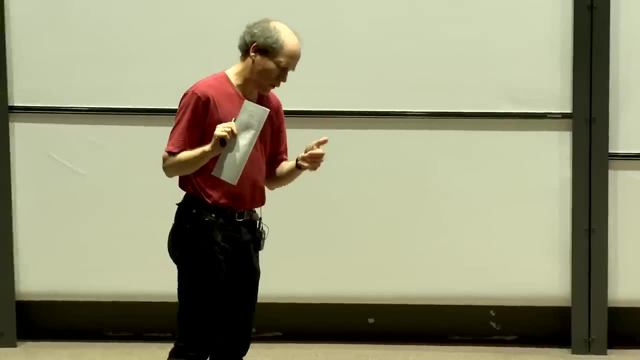 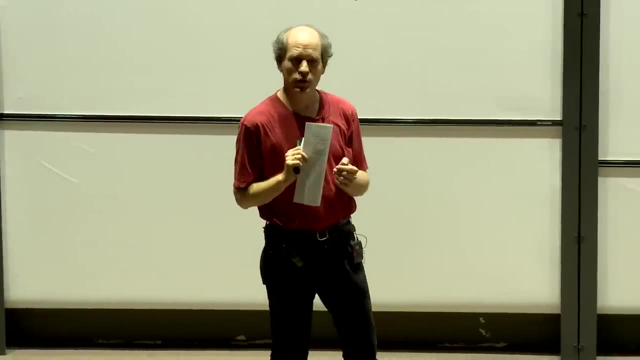 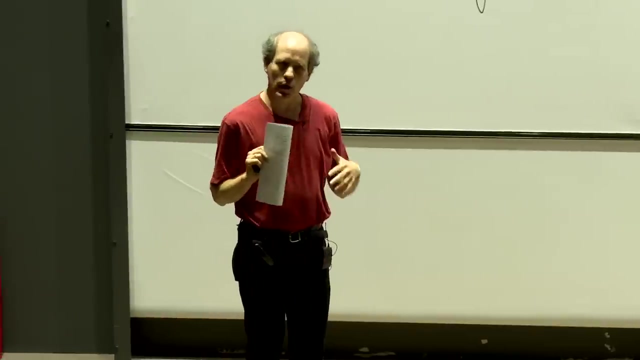 take decisions ultimately. now I'm a mathematician and you're studying, probably, probability in the context of mathematics or computer science or both- some of you with with philosophy and others with with statistics as well. but we are going to have to start at the beginning and really focus on the mathematical side of 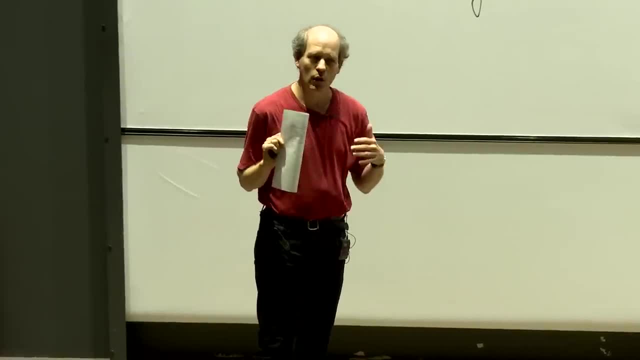 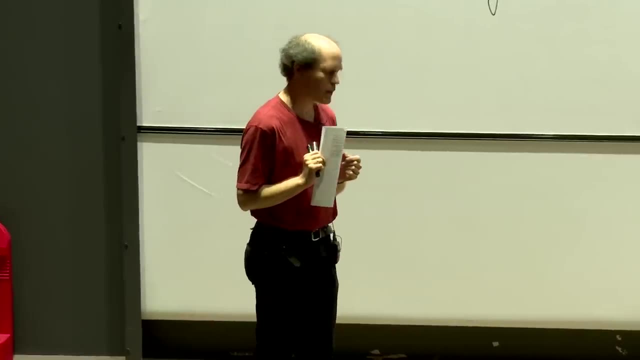 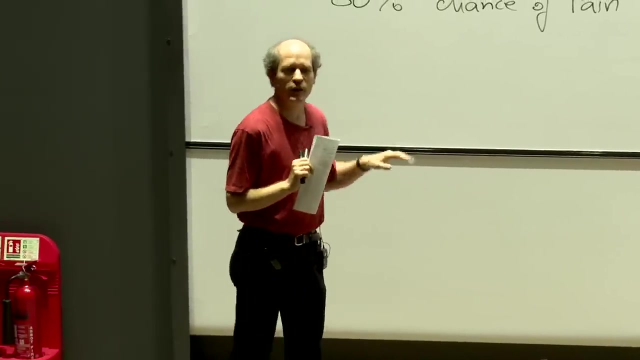 things. we want to answer the first questions. I asked: how can we make mathematically precise statements about probability? and that is what what this course is about. so we are going to introduce models in a way that is a little less fluffy than this eighty percent chance of rain, and we are going 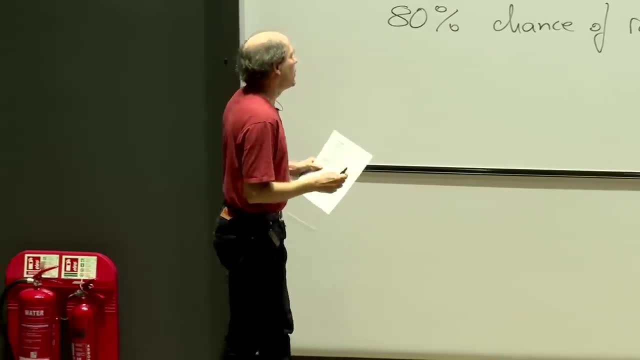 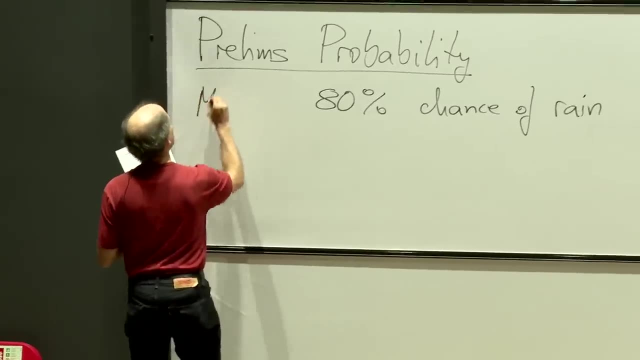 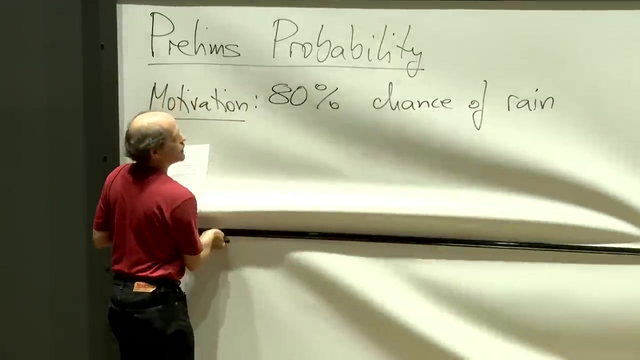 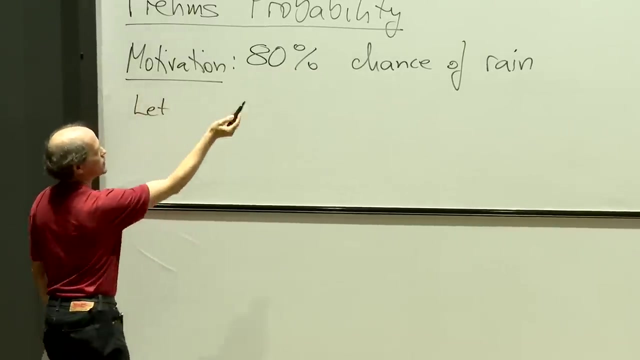 to to write things bit differently as a consequence. so so what? what I want to do here is maybe call this motivation and then and say: what I prefer is something like: well, I mean, this is- I put this in the context of Friday this week, and but what we, what? 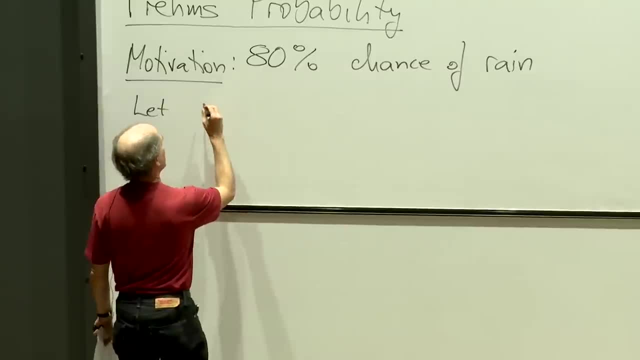 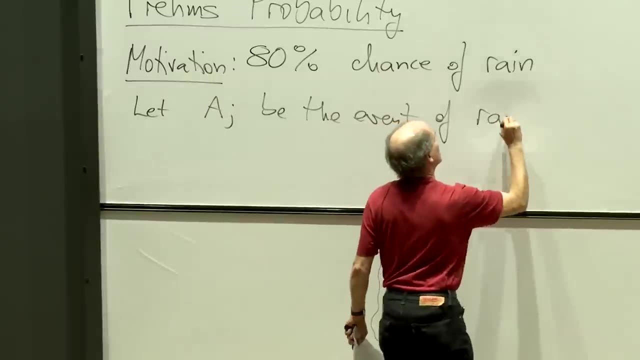 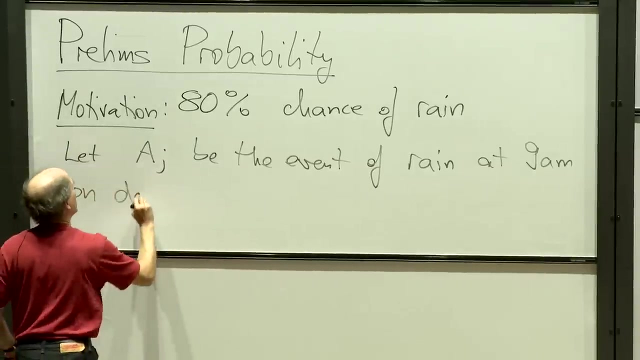 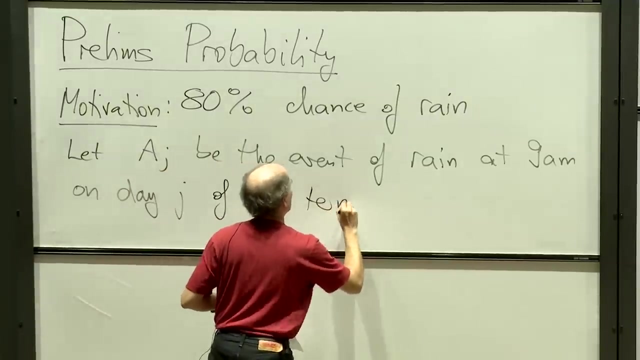 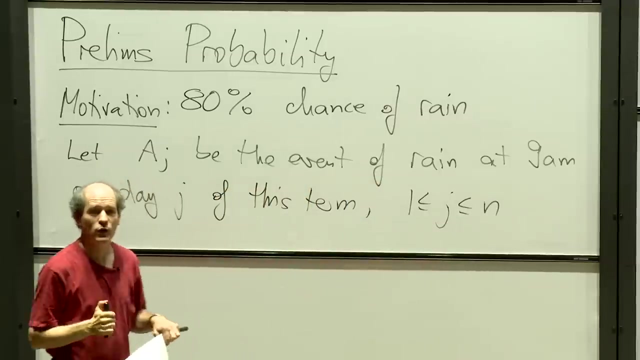 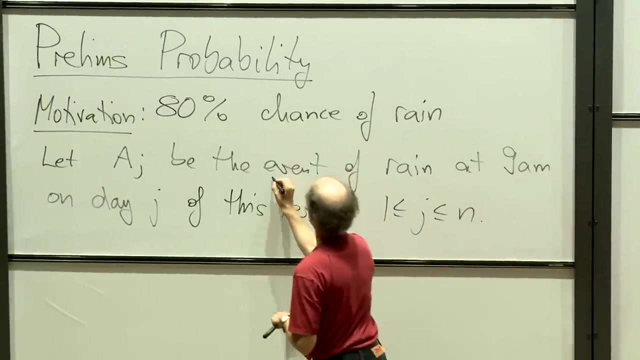 we might do more generally is say: let AJ be the event of rain at 9 am on day J of this term, right, and then you can take one less than J, less than n, where n is probably 40 or 39 if you exclude today. all right, so now I've used some language that I'll 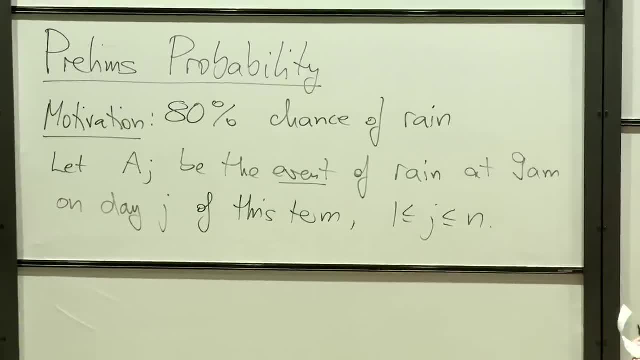 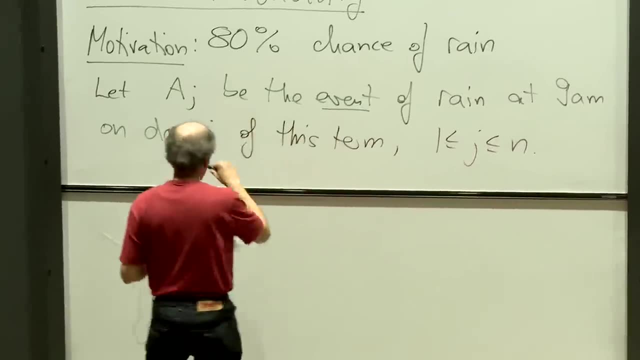 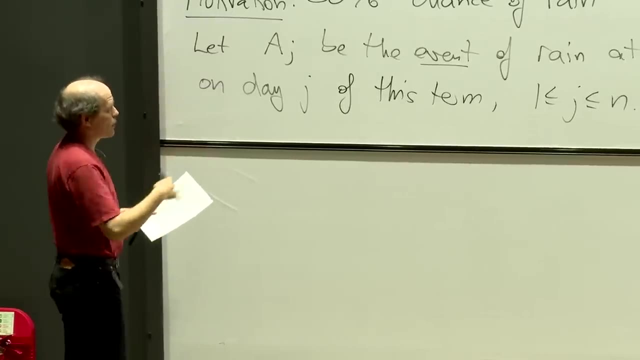 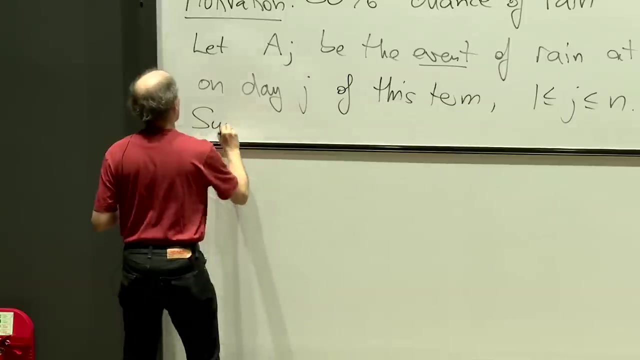 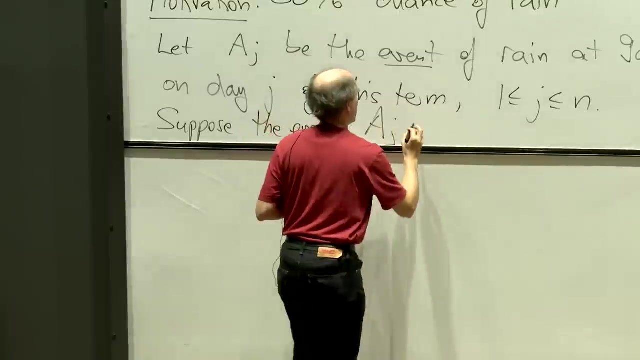 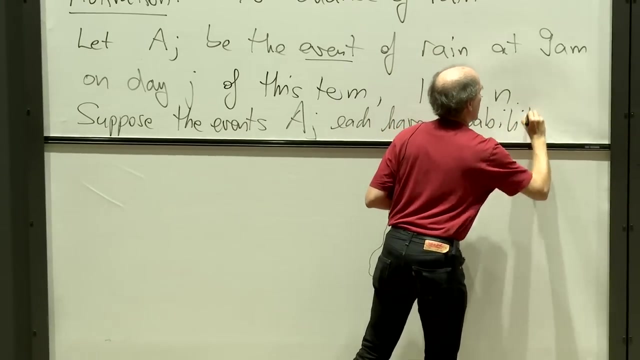 get back to call this an event. actually I want to call this an event in the mathematical sense. that I will explain. and then the next point is that we want to assess probabilities. now, when data are involved, is complicated, but at the outset we might just say and suppose the events AJ each have probability, P might be. 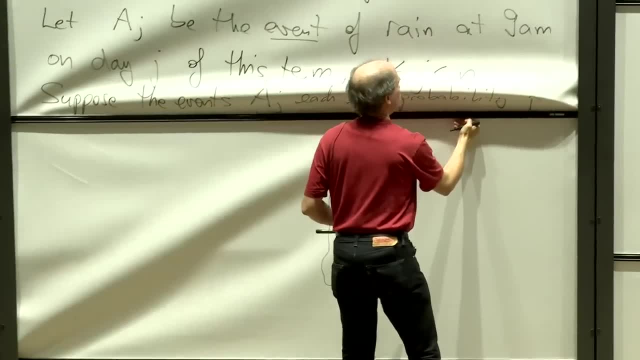 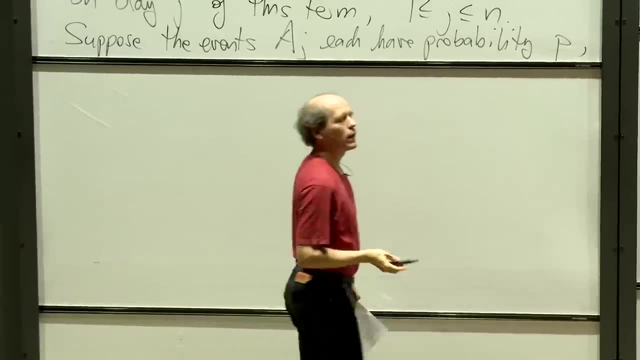 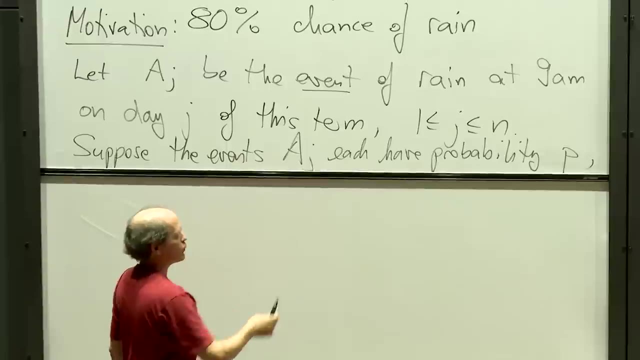 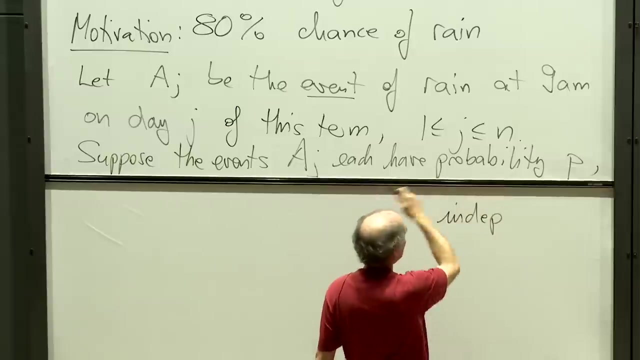 being something in zero one for this to make sense. right, that's getting more and much closer to specifying a model, but we need to say something more here and in order to fully specify a model, and that is some assumption about how these events are related to each other, and the simplest way of doing this is to say: 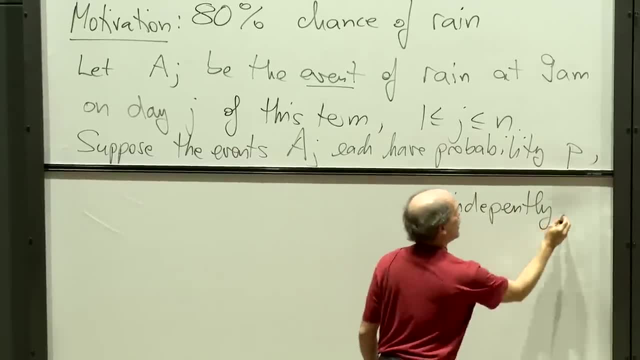 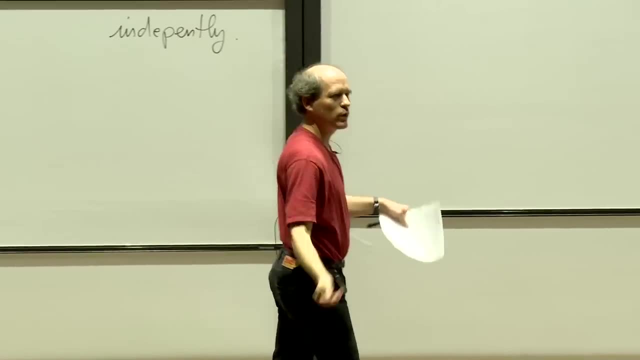 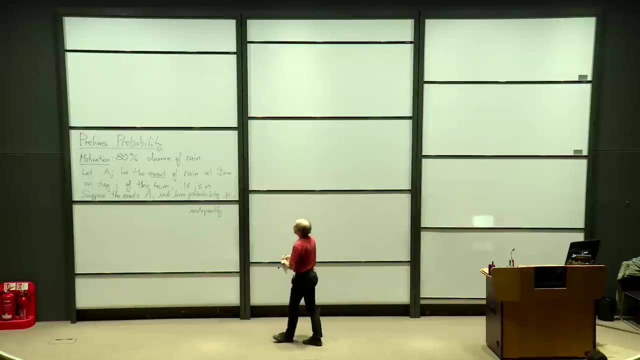 independently. now there are several questions, particularly coming from where we started with statistics, with, yeah, statistics mainly. So there are several questions here. What's p? clearly, But estimating p from data is not what we do in probability. That's left to the statistics course. 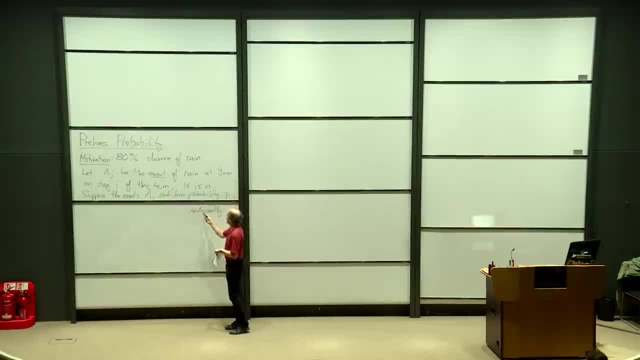 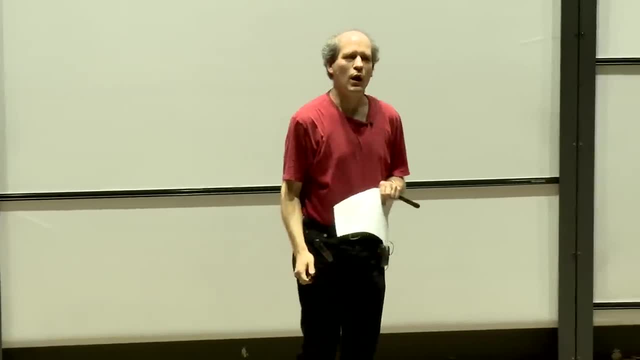 And then there are questions about assumptions, notably independence. but also, is it the same probability each time? Even if you look at the weather forecast, they tell you: well, tomorrow the probability of rain is less than 5%. On Wednesday it's 20%. 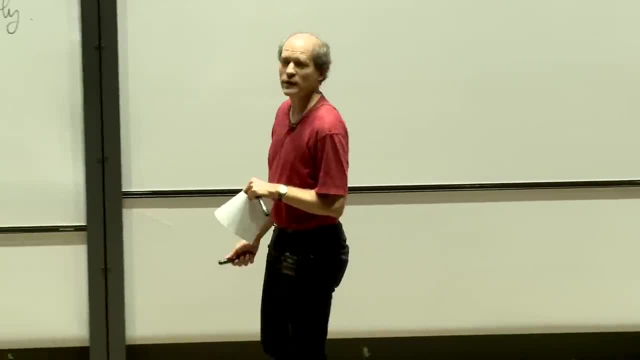 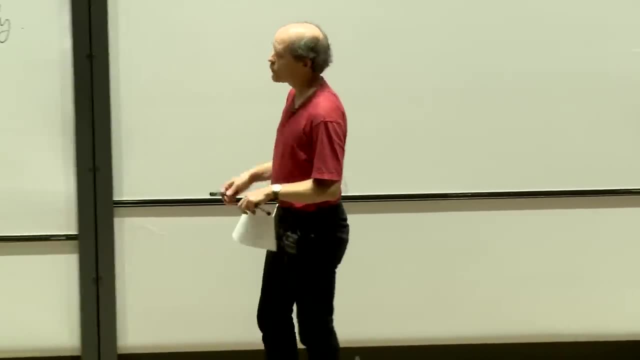 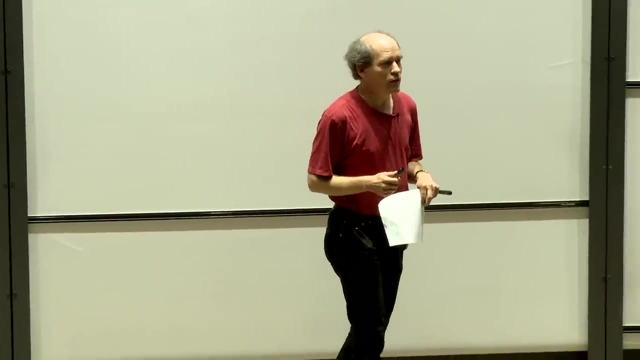 On Thursday 10% And on Friday it's 80%. So clearly the Met Office suggests models where the p varies, But we have to start somewhere, And this is the kind of setting that you will see most likely in this course. 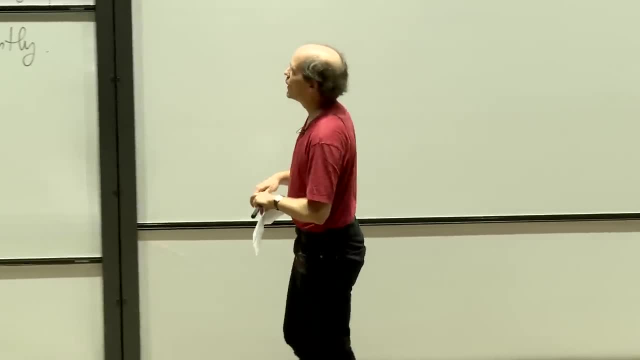 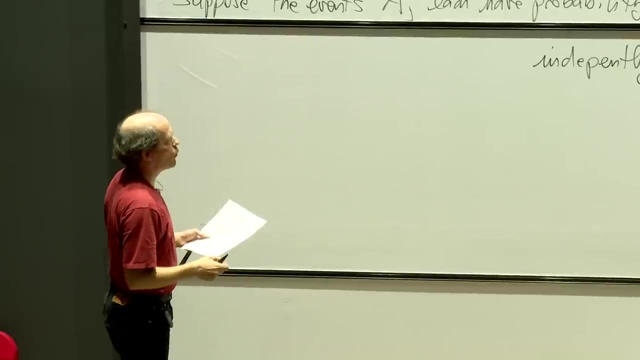 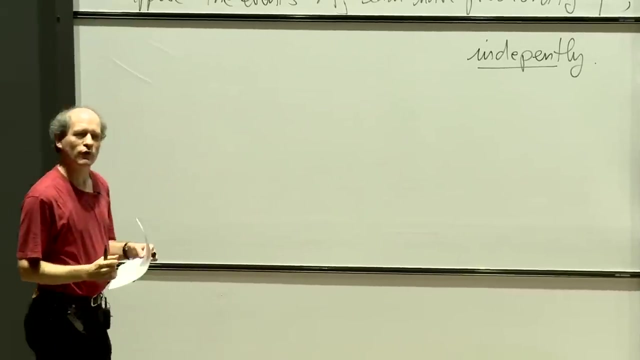 with events that are independent and have the same probability. But of course that generalizes in some way easily, but as far as the independence is concerned not so easily. I'm using words here that I will of course explain in due course. 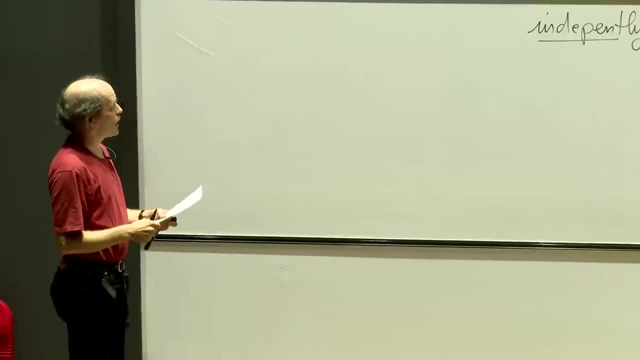 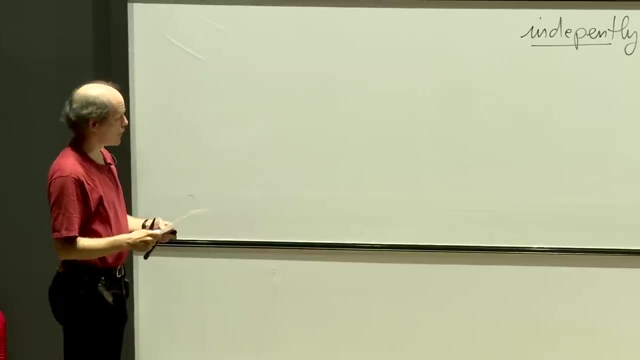 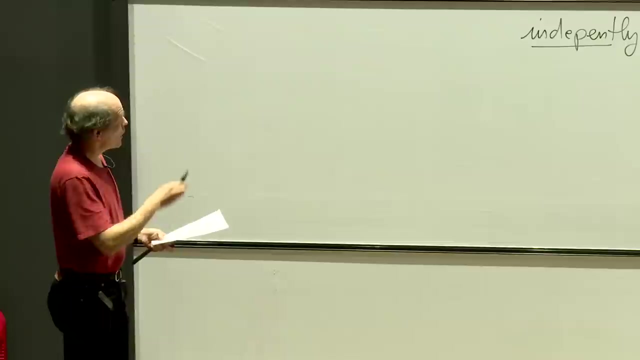 The word event. I will make precise as the next thing. I do pretty much The word independent. if you haven't seen, it is coming in much later, Or you can certainly use your intuitive meaning for now. Once we have something like this, we can answer questions such as: 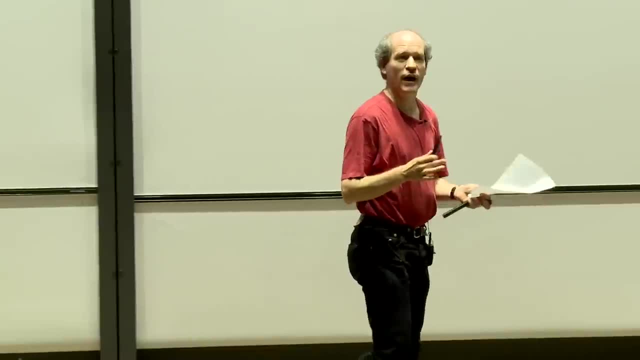 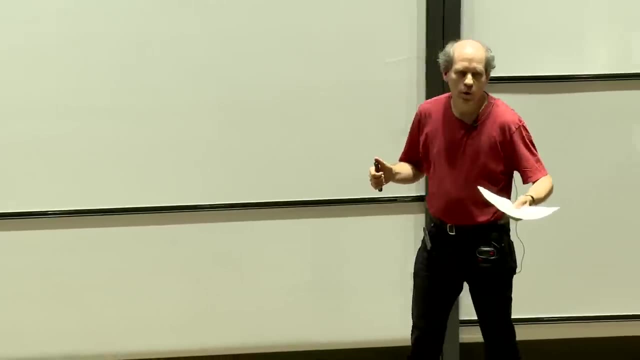 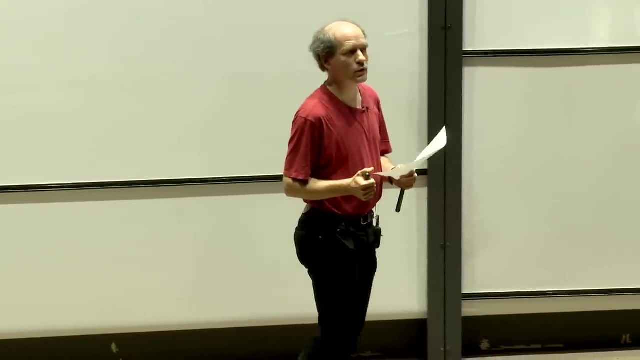 what's the probability that we have rain for k days out of those n days this term? And you can probably answer those with your school probability. If you've learned probability at school, that will be among the kind of questions that you may be able to answer already. 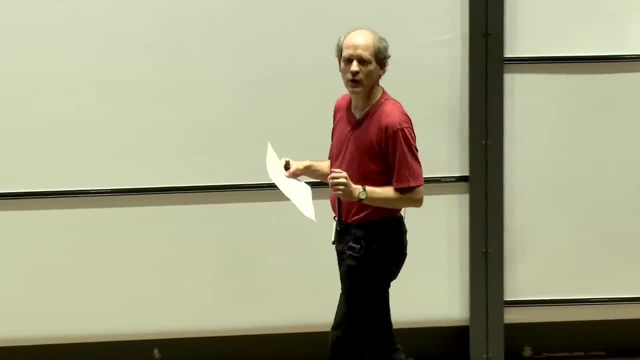 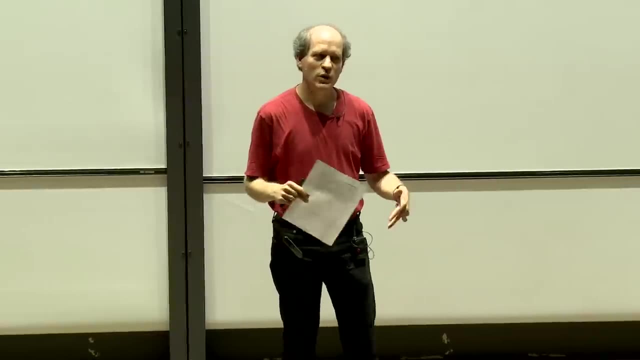 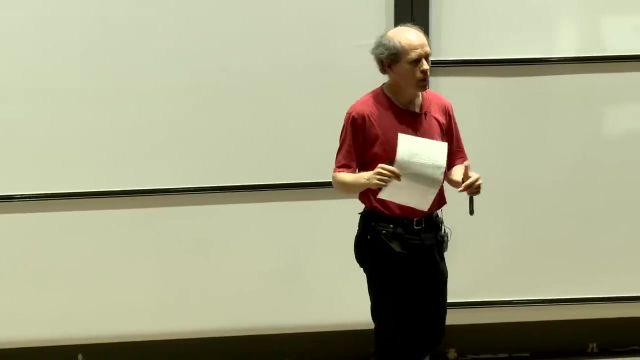 But what we are doing here is putting some of the things that you learned at school on a more formal basis, And so I would always encourage you to think: how does this question relate to the course rather than just to what you know already? Because that way you pick up the formalism that may not be strictly necessary. 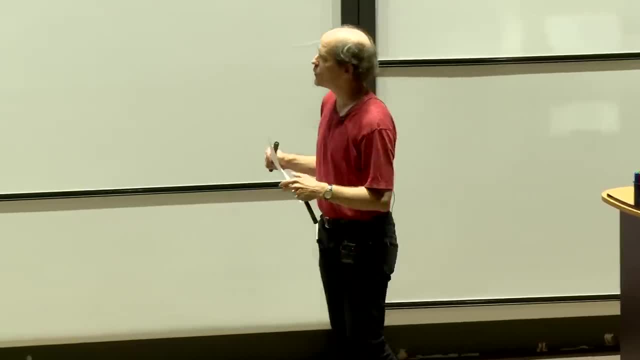 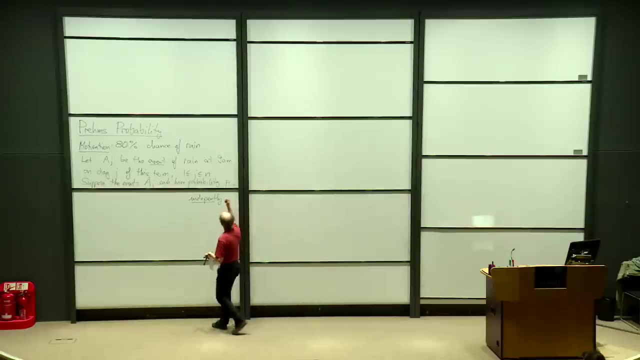 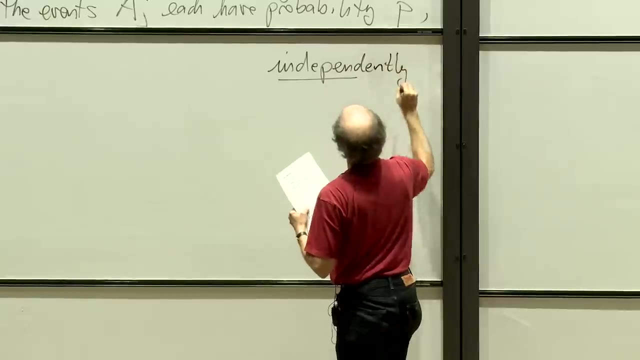 for the questions at the beginning of the course, but where you will need to be more fluent as we go along Now. and there is a common mistake here in the word independent, that it kind of has too many letters. Okay, I think this is okay anyway. 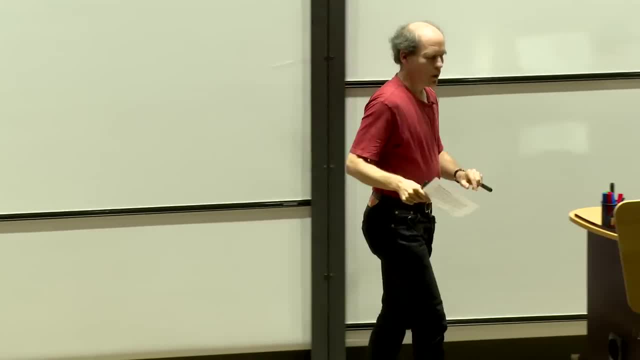 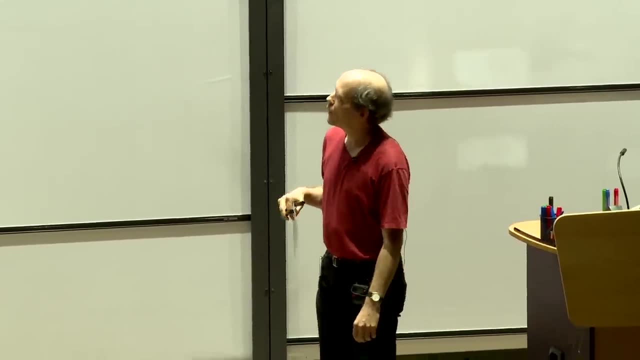 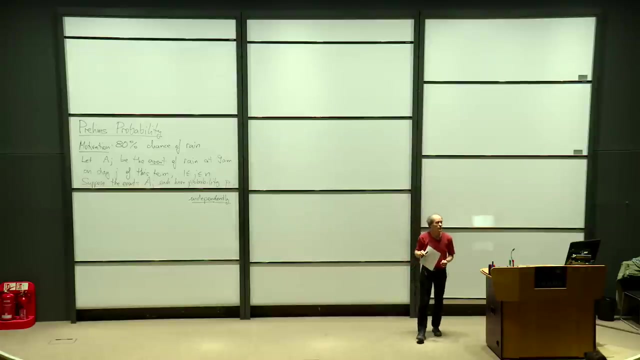 Right, so I've written on the board. it's my first lecture after a while. I always have to remind myself to write in large letters And you can already see I started very large and got a little bit smaller. How is it at the back of the room? 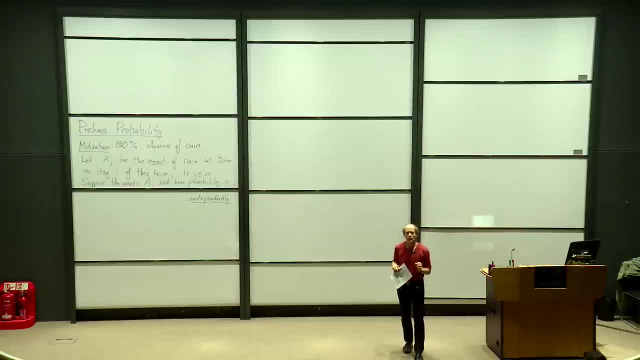 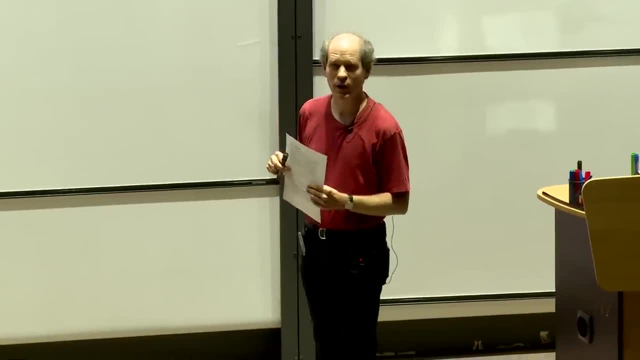 Can you see everything that I've written? Okay, Thank you. If ever I get even smaller and you can't, please tell me, Because that's useful feedback, useful interaction that we can have in a lecture, So please don't hold back. 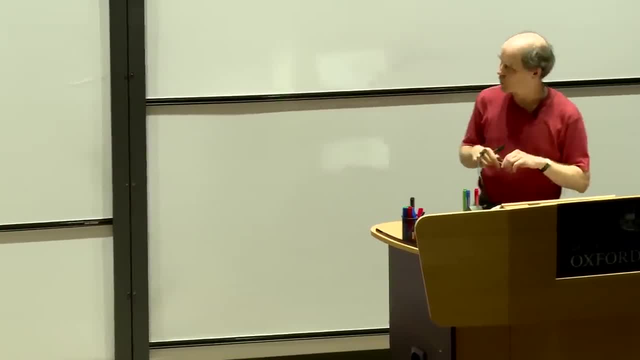 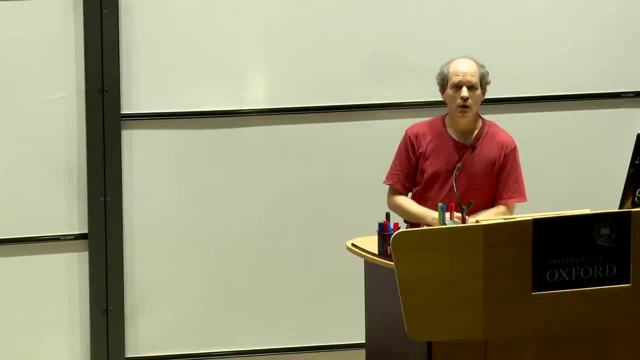 Now, before I continue with writing there, I've got a bit more advice here. My style of lecturing is going to be chalk and talk, as it used to be called. Here's my chalk And I'm going to write on the board. 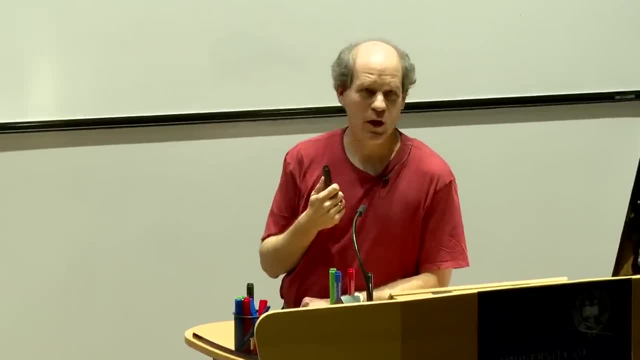 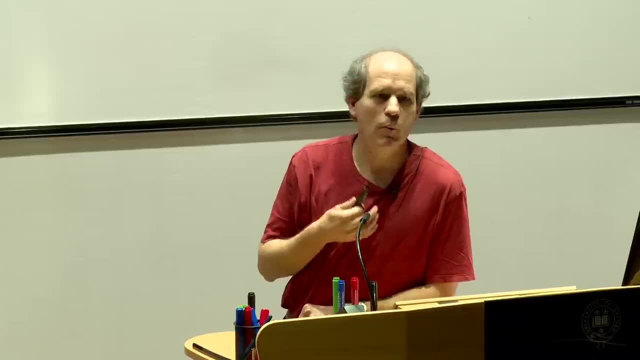 And paraphrase what I'm writing, but I'm also going to give some extra explanations, And what I'd like you to do, or recommend you to do, is to respond by something you might call ink and think Ink, because it's a very good idea to take notes. 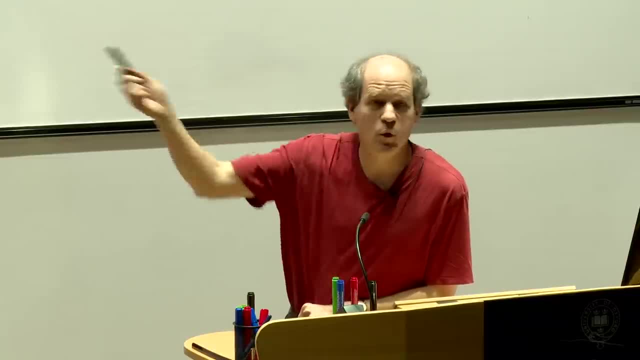 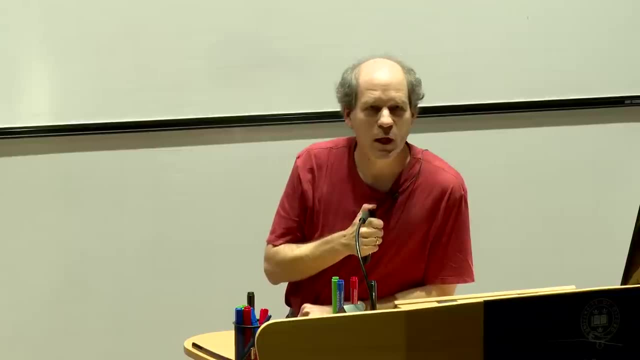 And think, of course, because there's a little more than getting what's on the board onto your piece of paper, But the important process of getting it through your head and out at the other end is already a first way of processing, And you may well find that what you write with your own hand you feel more committed to when you're trying to fully understand it. 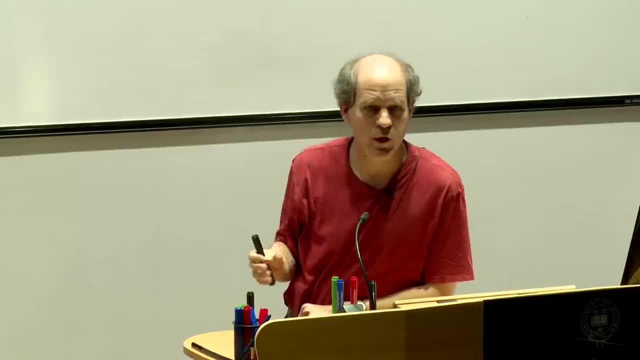 And if you've written something that you're not quite sure about, you can leave a trace and say: oh, I want to get back to this, So I really hope you can do that. Mathematics is a very active discipline. You really have to do it yourself. 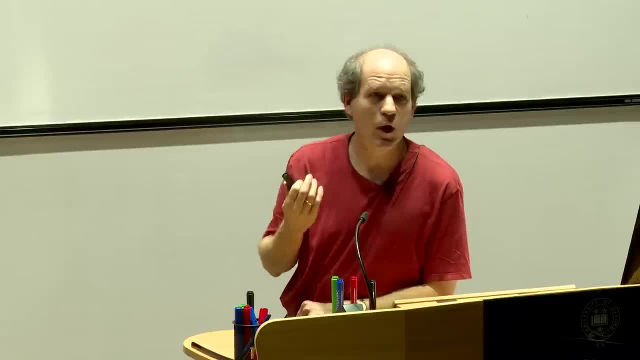 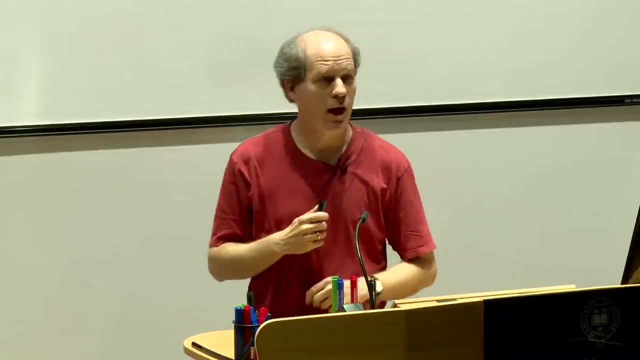 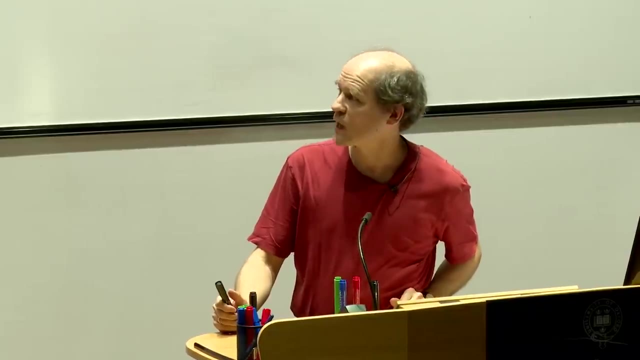 You can't rely on what you see in front of your eyes, So make sure you get the most out of lectures by doing something such as taking notes, if you can. If you feel you're falling behind and you can't listen very well, there are other ways that you can try, such as having printed lecture notes. 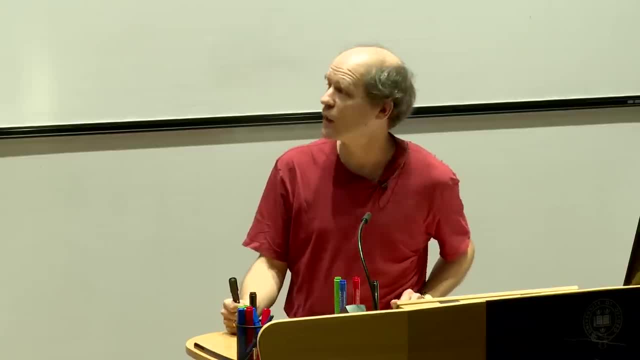 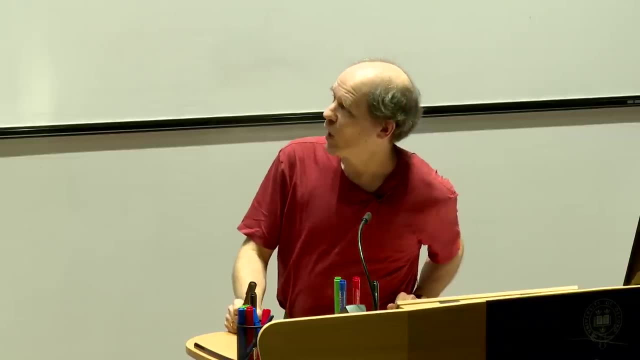 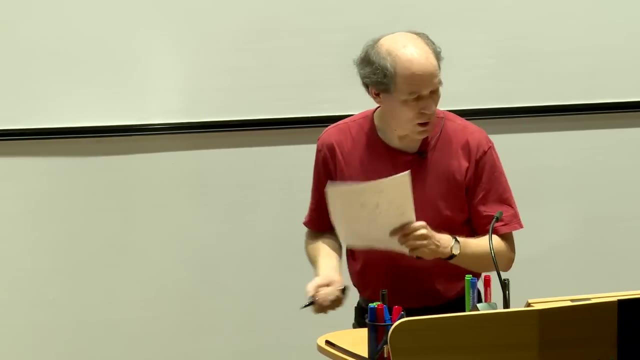 Or I mean anything can be done with a tablet and a stylus, But you can annotate things usefully as well, As long as you stay active. that's the best way of working. That's the best way of making use of the lectures that we offer. 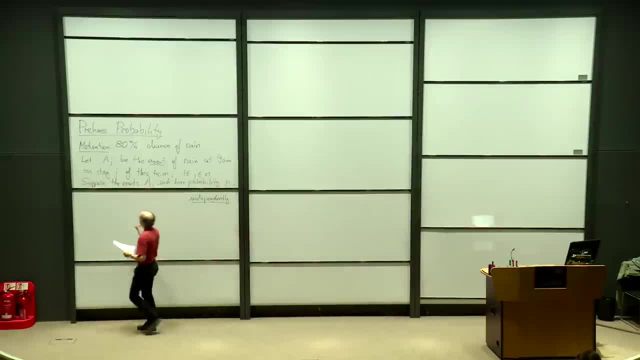 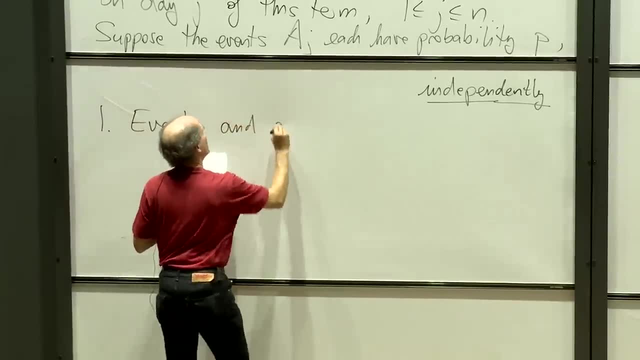 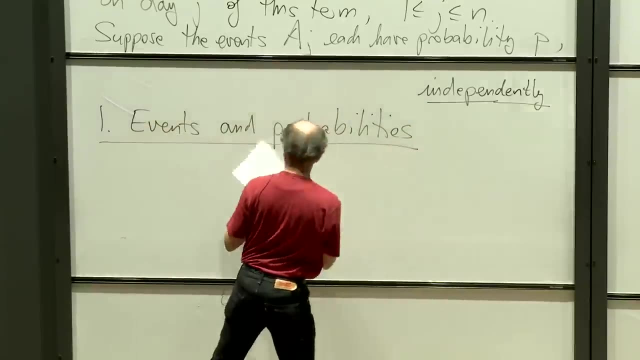 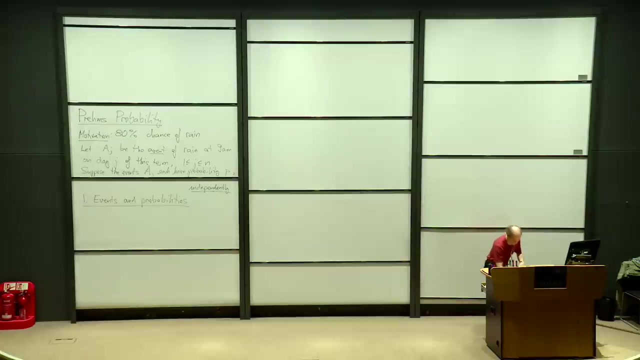 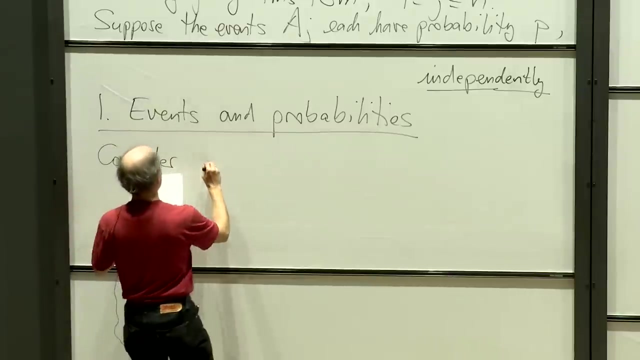 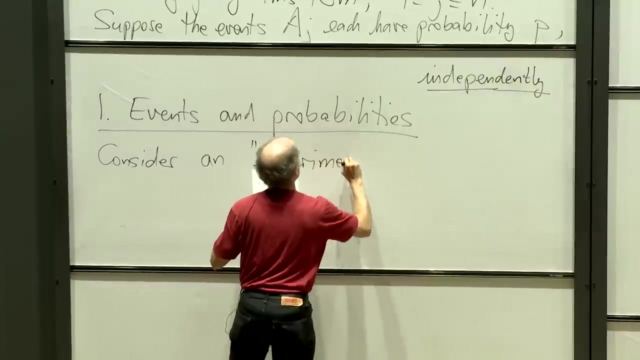 Okay, So let's get started with chapter one: events and probabilities. I think I need more pens, So the specific setting that we've had so far, Let's see what generality we can put this in. So let's look at an experiment. 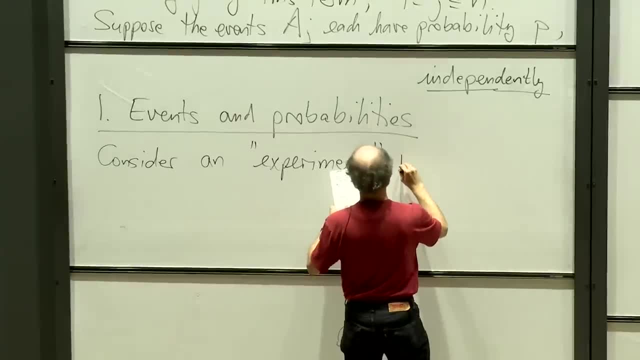 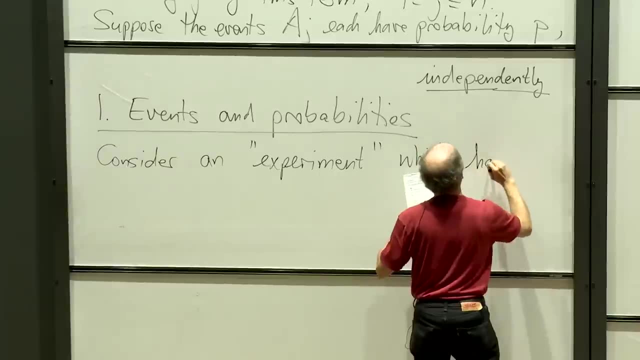 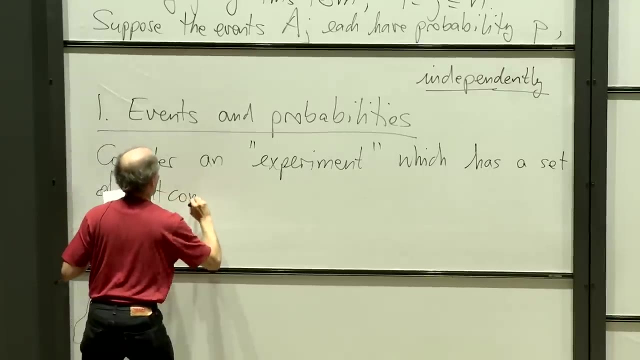 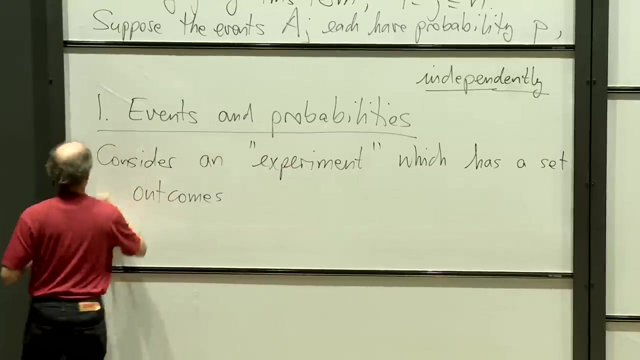 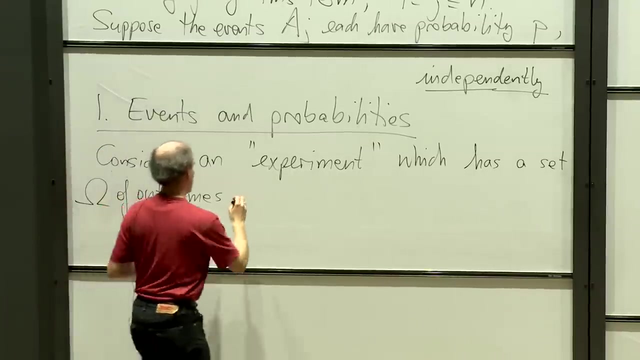 And that word is sort of in inverted commas, because not everything you might think of as an experiment. But let's look at an experiment which has a set of outcomes And let's call this set omega of outcomes And let's call the outcomes little omega in capital omega. 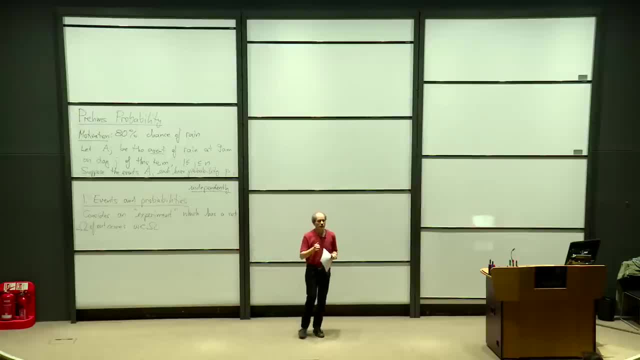 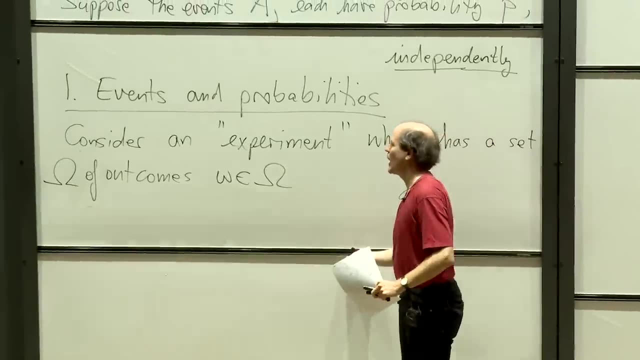 And, if you're well, for the mathematicians among you, certainly the introduction to university maths lecturer put a video online where he writes out all the Greek letters and points out that some of them are more useful than others. So certainly omega, the last letter in the Greek alphabet, is something very prominent in probability. 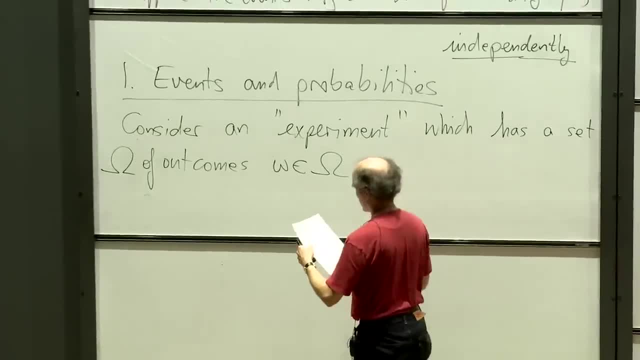 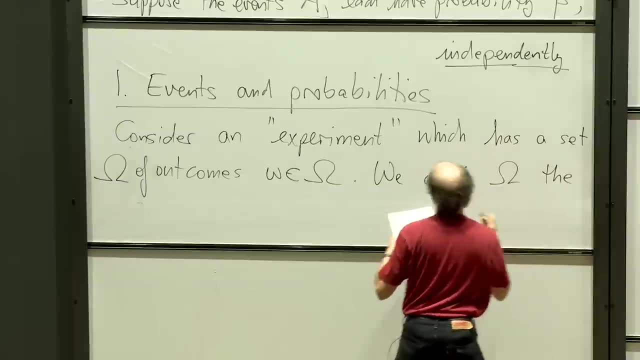 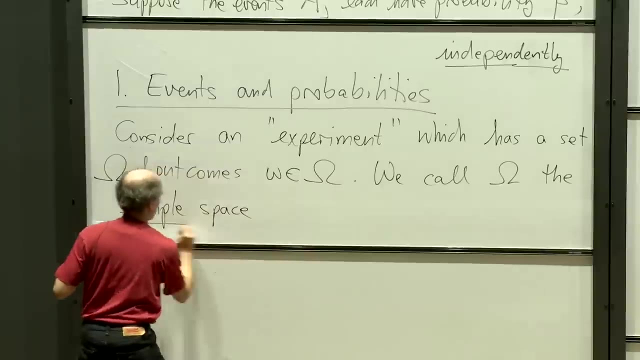 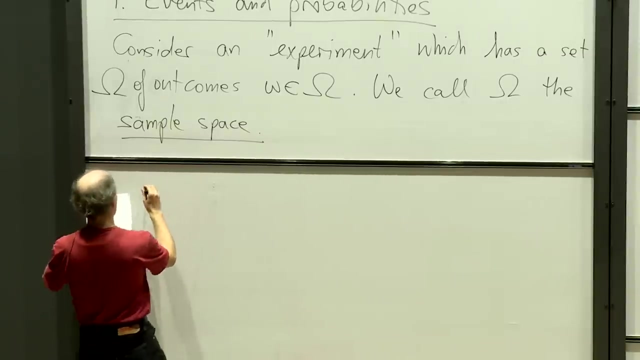 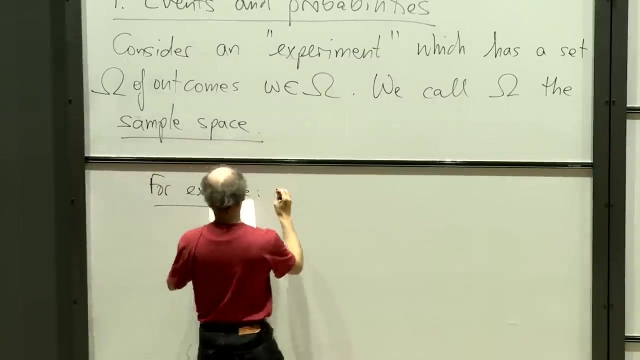 And so I'm using those letters here. So we call omega the sample space, Okay, the set of possible outcomes. So what sort of experiments might you want to have in mind? So here are two examples. So if you're tossing a coin, 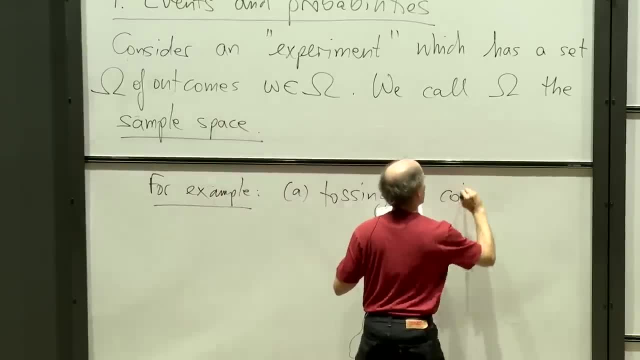 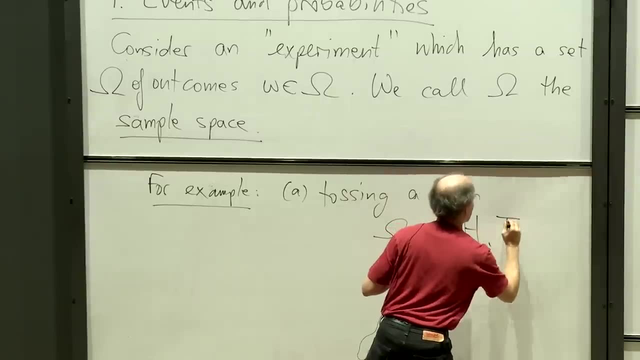 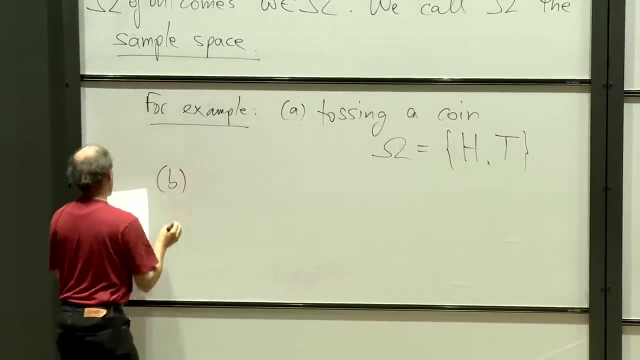 what are the possible outcomes? Well, quite clearly, two possible outcomes. heads and tails is what they're usually called, So let me write H and T. Second example, if we are throwing dice- and let's make this a little bit more interesting- 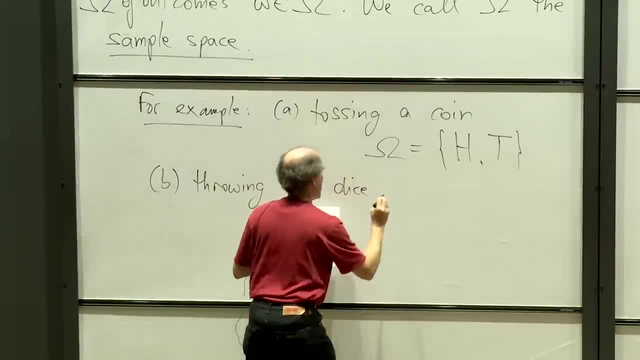 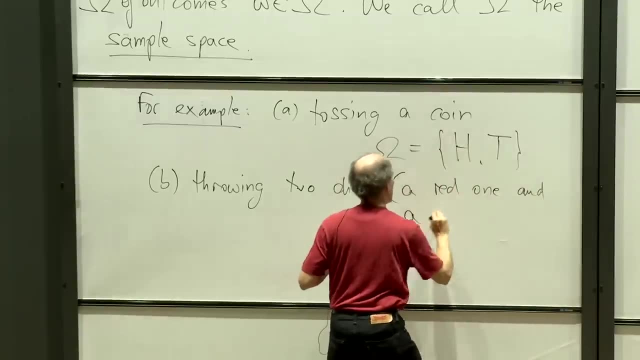 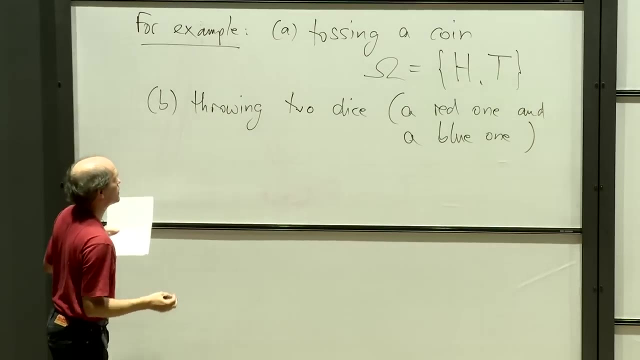 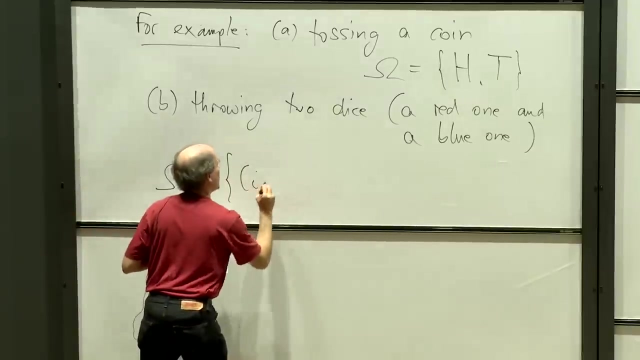 let's throw two dice And let's make them distinguishable: A red one and a blue one. What is the set of possible outcomes of this experiment? Well, in this case, we are observing two numbers between one and six. Let's call them I and J. 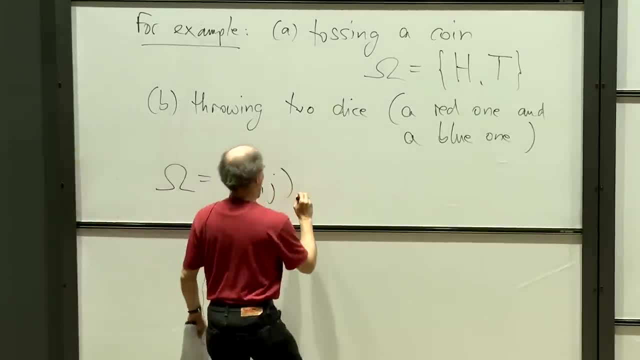 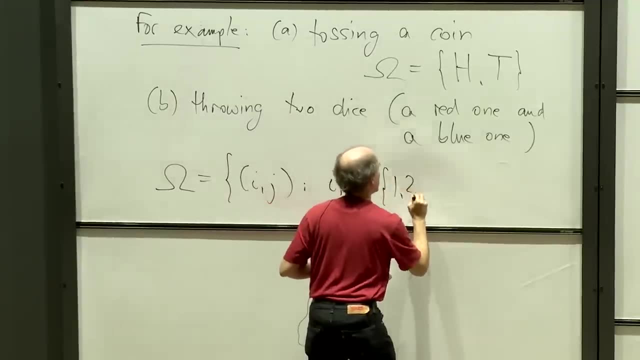 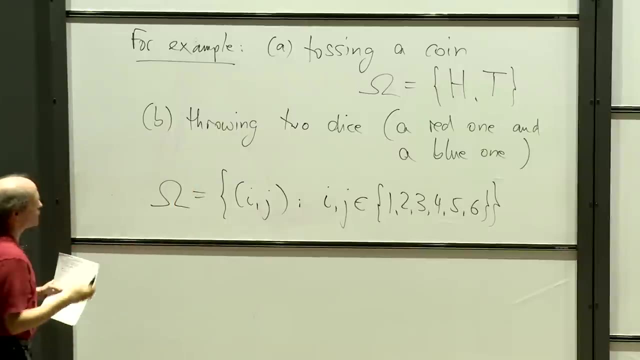 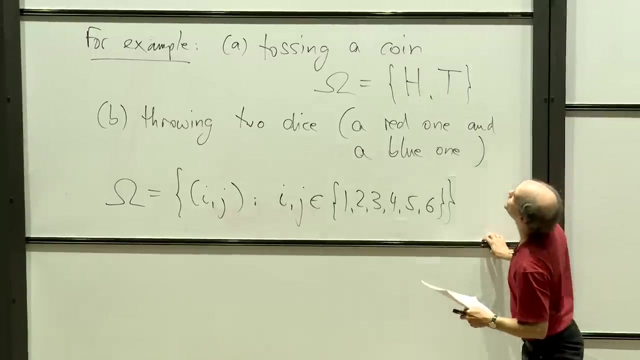 Put them into a pair like this, And let's say we want I and J elements of one, two, three, One, two, three, four, five, six. Okay, so these are natural examples of sample spaces of some simple experiments. 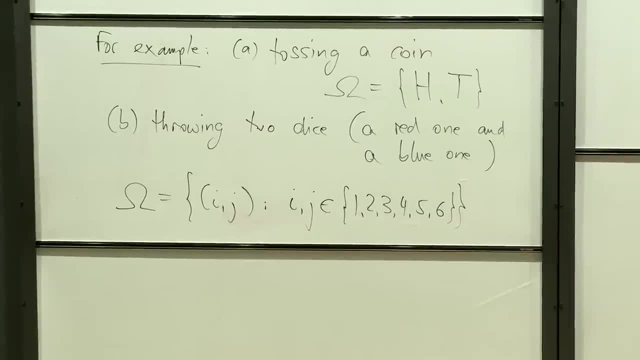 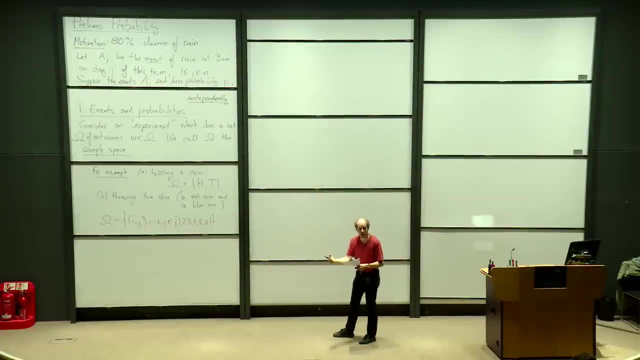 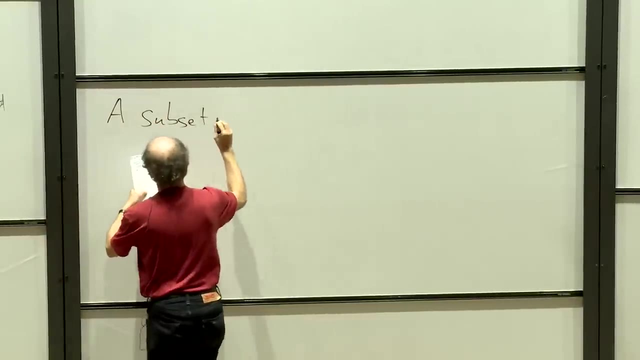 So once you have an experiment, we can define events, certain things happening in the experiment, And that may not only be observing a particular outcome, It may be something a little bit more interesting And more generally. we call a subset. of omega is called. 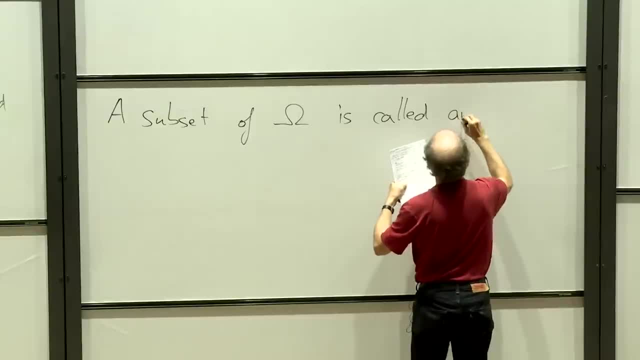 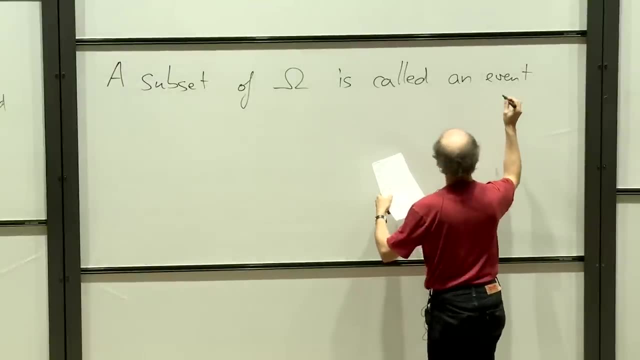 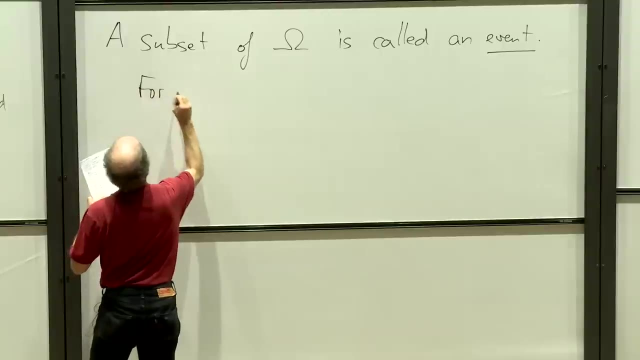 or any subset of omega is called an event Or well, for now, There may be some restrictions later, but not for a long time in this course. So again, for example, in the two settings where we have a sample space specified. 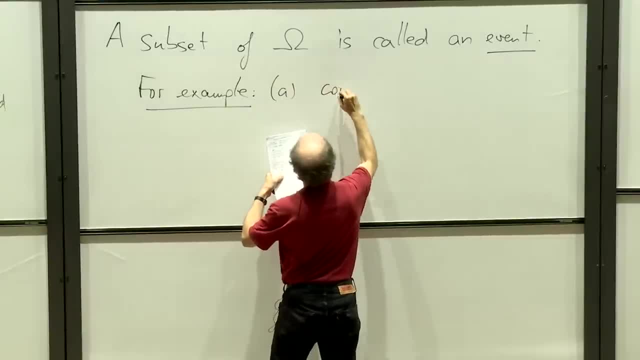 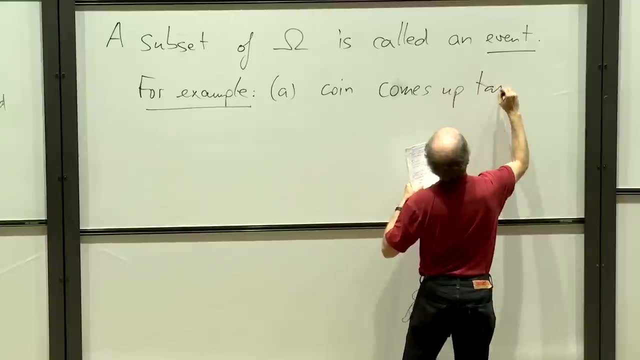 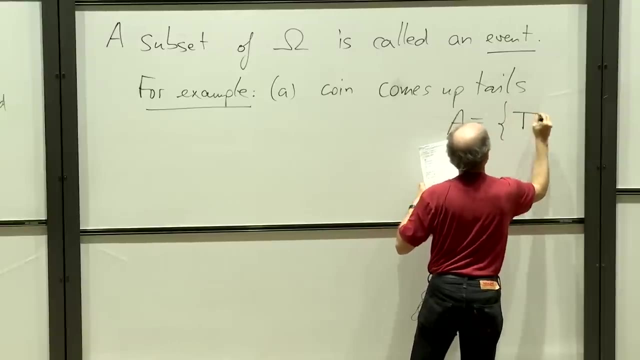 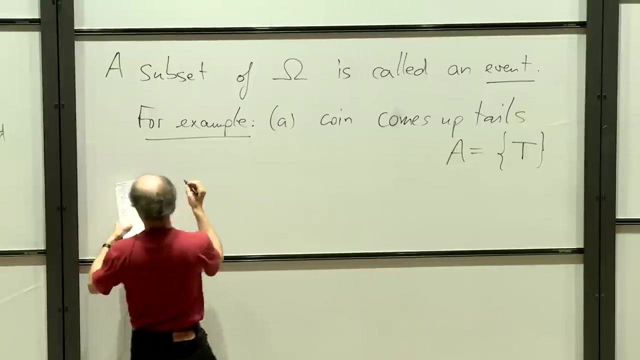 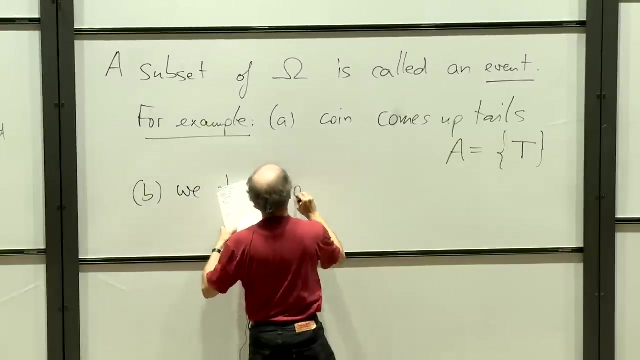 we can look at the event that the coin comes up tails. That is an event. let's call it capital A, which is the singleton set that contains the outcome, T Or B. in the setting of throwing two dice, we observe a total of nine. 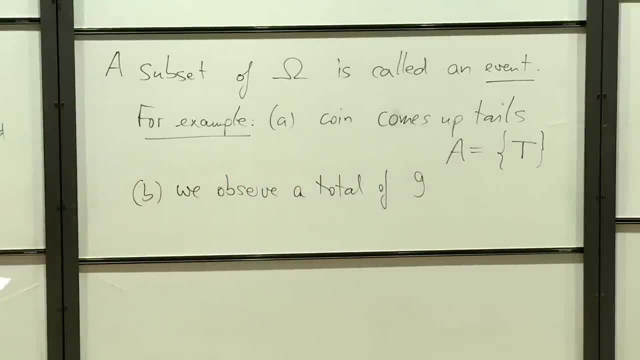 That is, the sum of the two outcomes of the individual dice is equal to nine And that corresponds to an event A as a subset of our sample space that has several members, because you can achieve nine in four different ways. If the first one is a three, 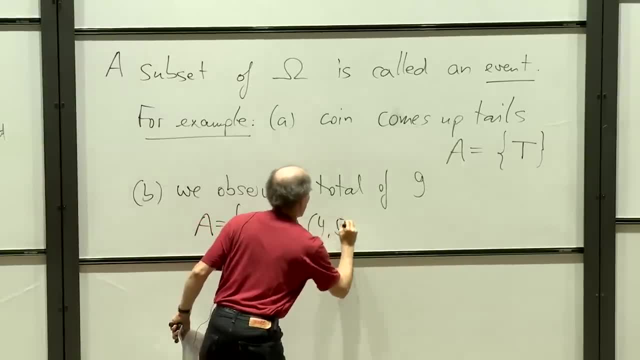 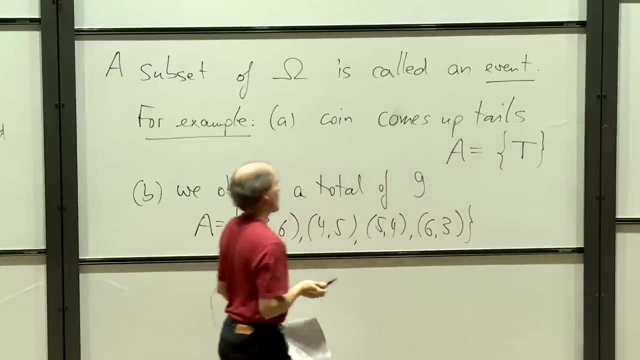 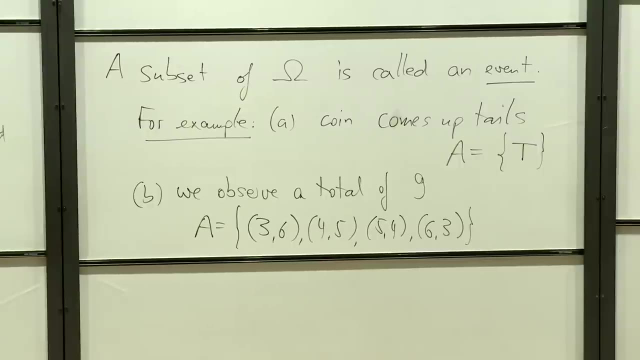 the second one has to be a six. you can have four, five, five, four or six, three. Okay, So this is just simple definitions and terminology that we are going to use. Now we are talking about sets here. 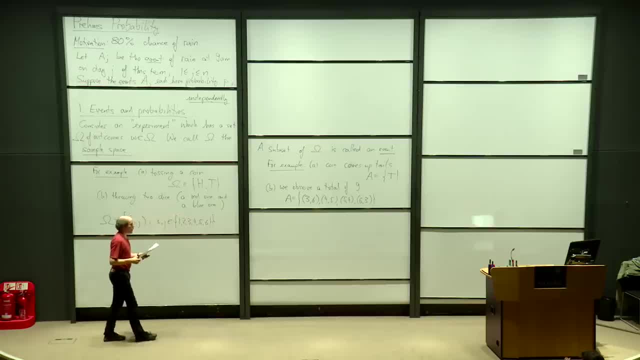 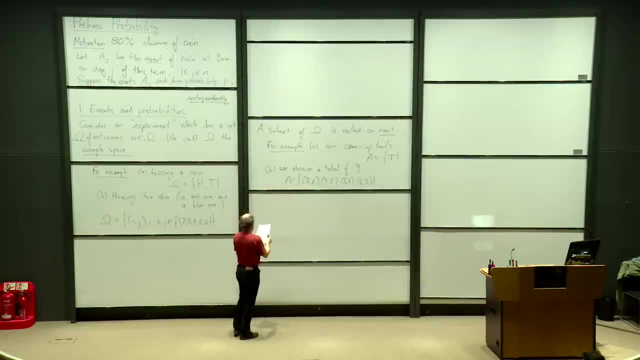 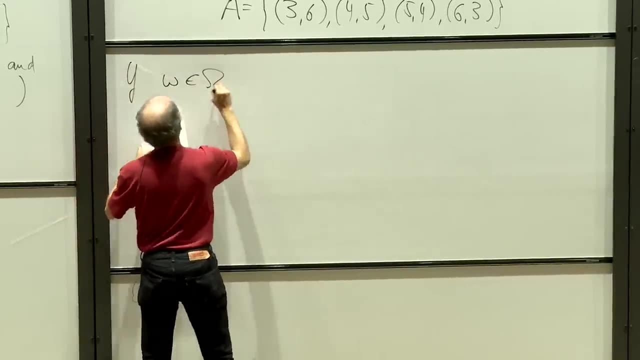 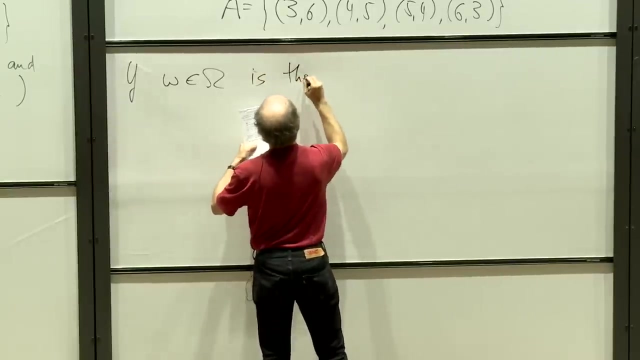 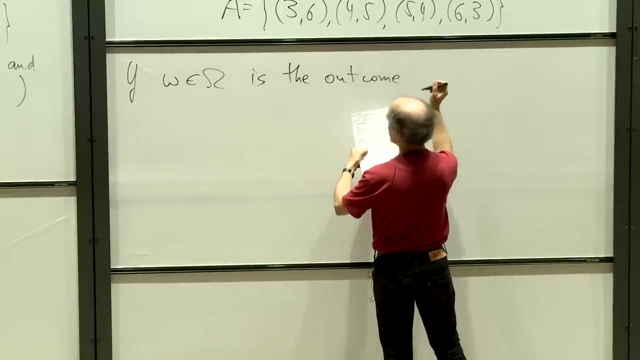 so it makes sense to just use the language of sets in our course here And recall some of the notation as well. So first of all, if omega is an outcome, and if this particular omega is the outcome that we observe, then we can talk about what it means that the event A occurs. 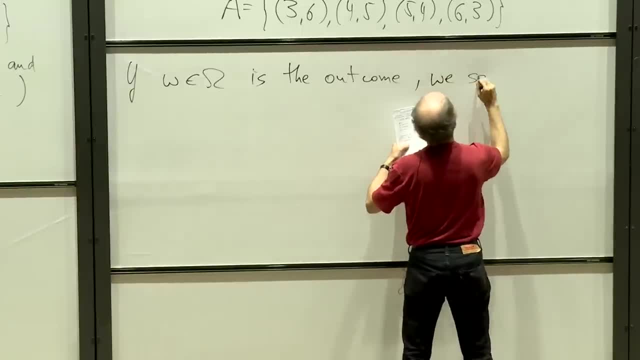 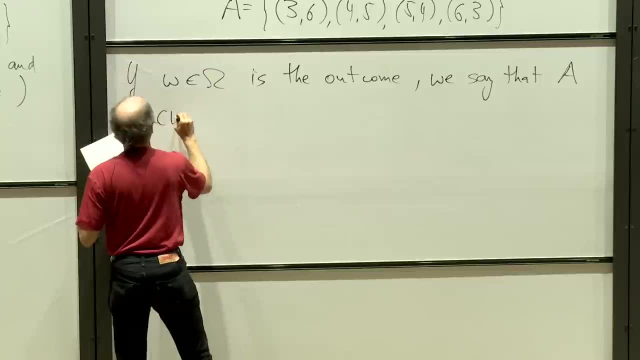 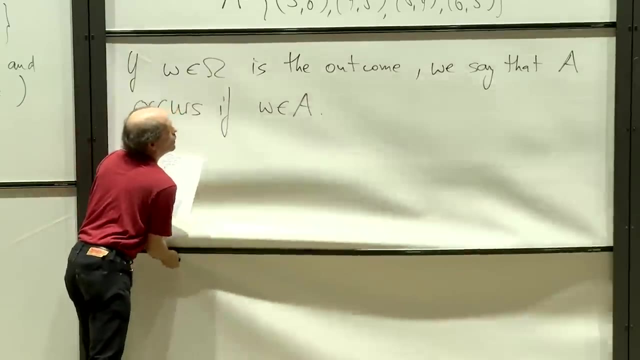 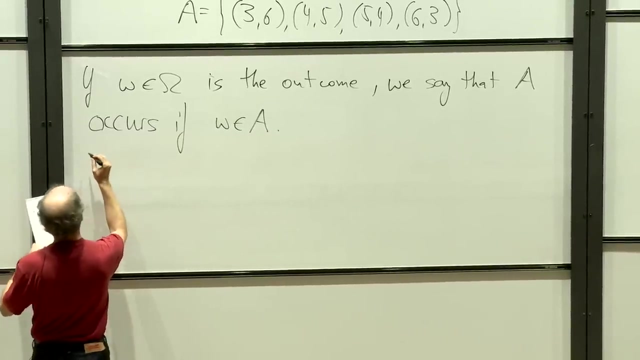 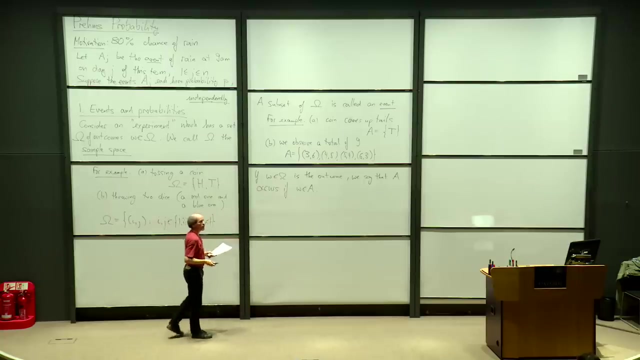 So if omega is the outcome, we say that A occurs if omega is in A Right, Quite, naturally. So how can we use this terminology? Well, I've said, these events are sets, so we have set operations that we can interpret in terms of events. 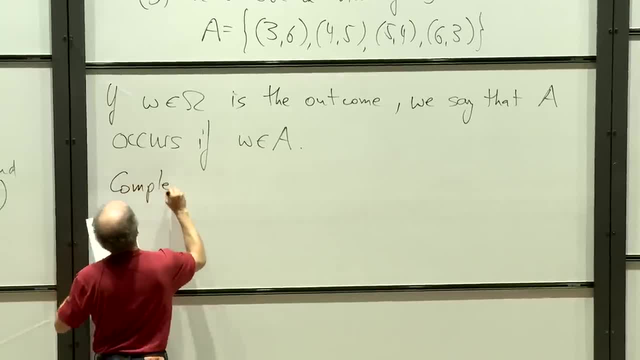 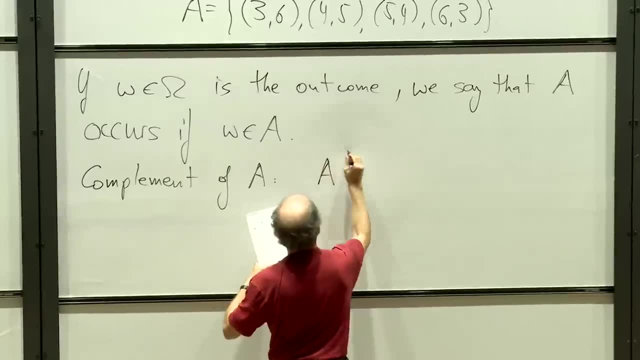 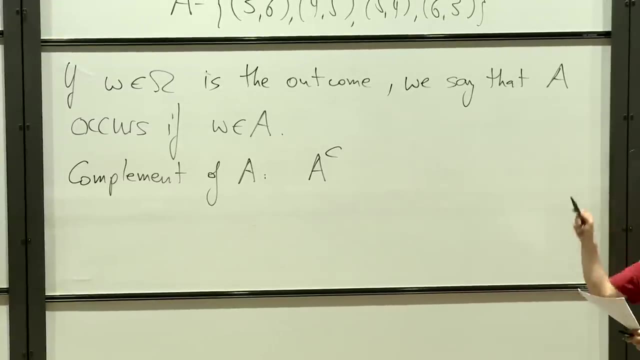 So the first one here is the complement of an event, So the complement of A, and that is denoted by A with a superscript C generally here in our mathematics course in Oxford Some people may put bars on top or have some other notation. 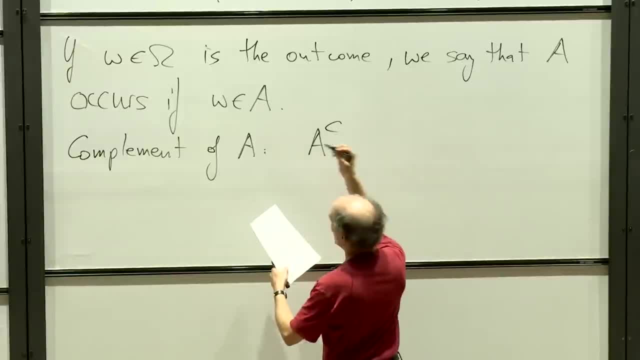 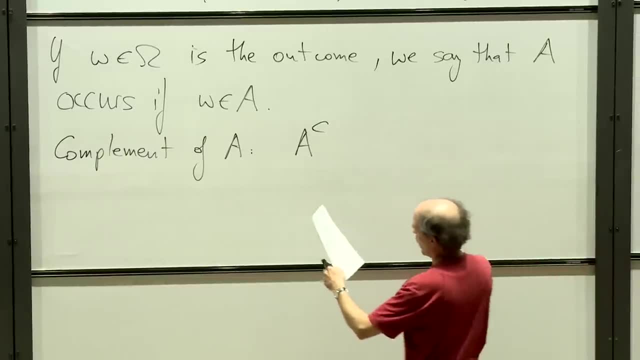 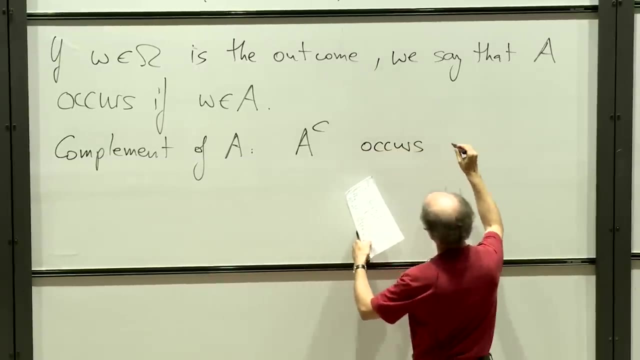 but this is what I recommend you use. Now, if A is an event, A complement is an event as well, because it's also a subset of omega. In fact, it's complement within omega that we are taking. And what does it mean for A complement to occur? 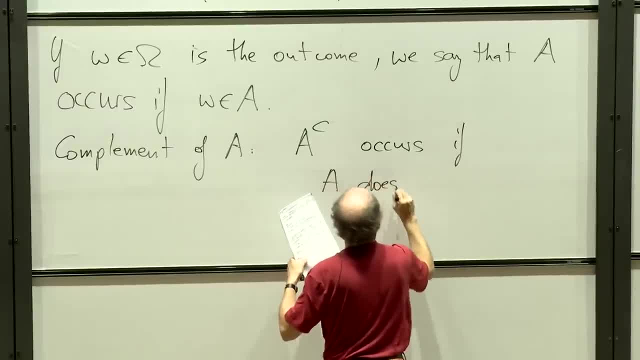 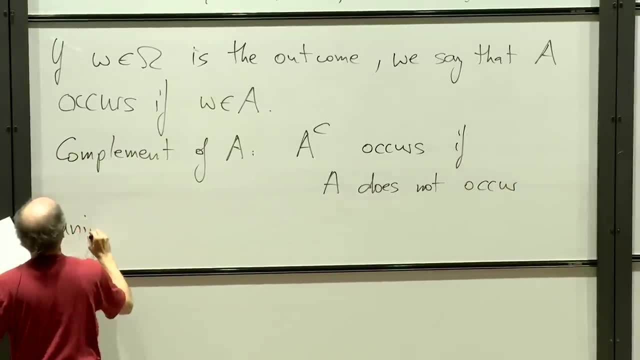 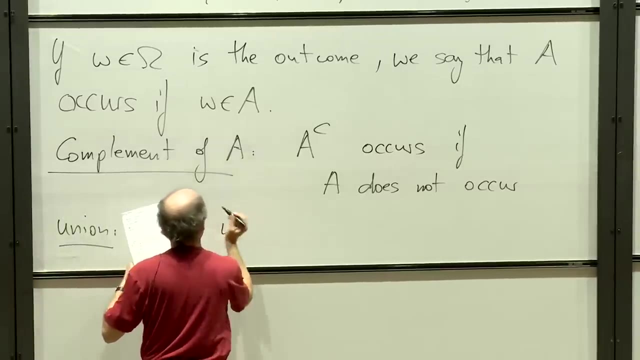 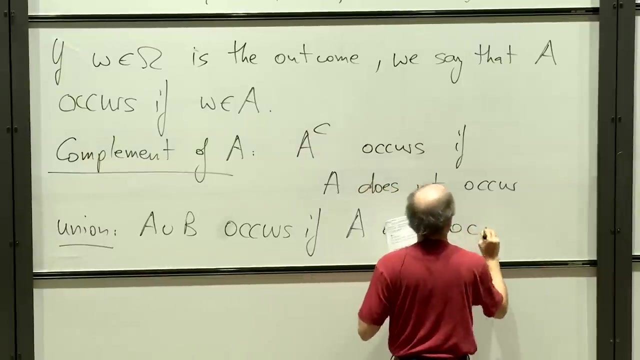 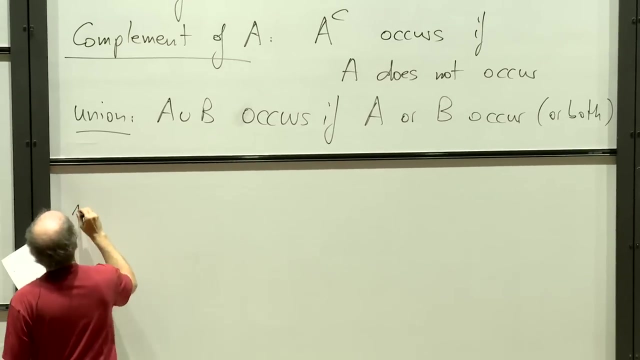 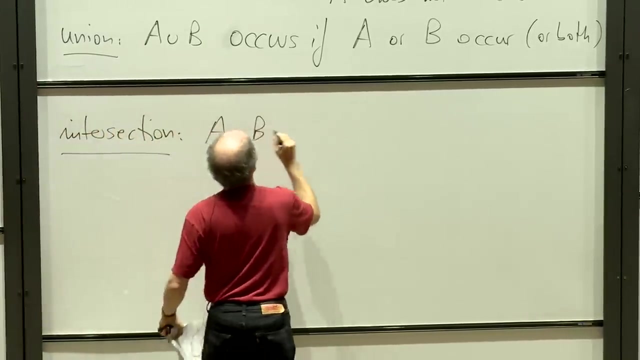 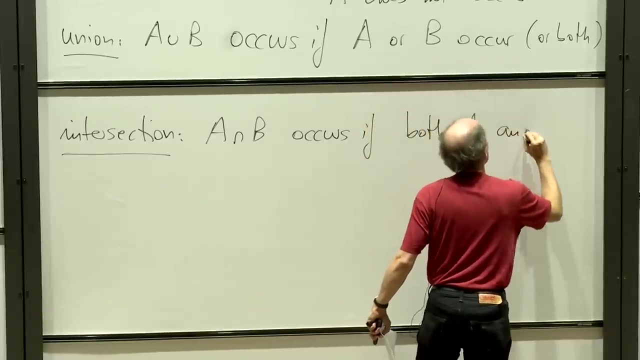 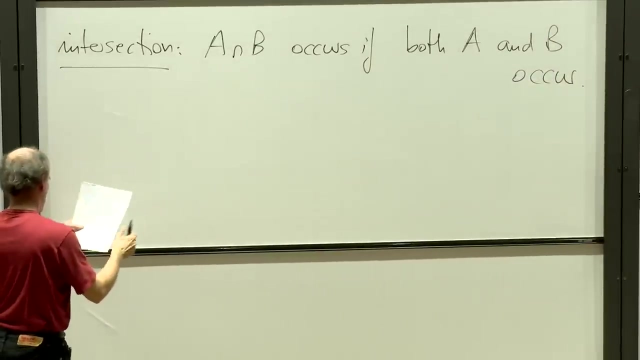 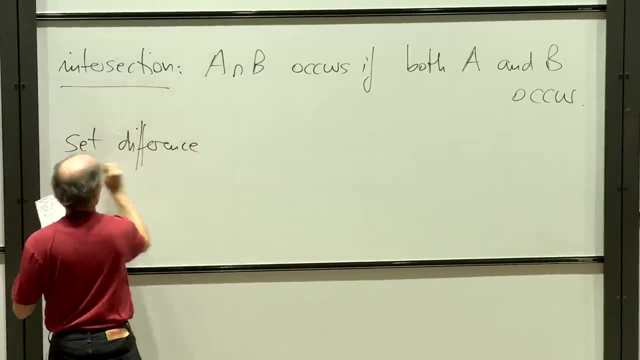 It means that A does not occur. Okay, Now we can have union. So a union A, union B occurs if A or B occur or both. and intersection A, intersection B occurs if both A and B occur. What more Set difference A minus B? 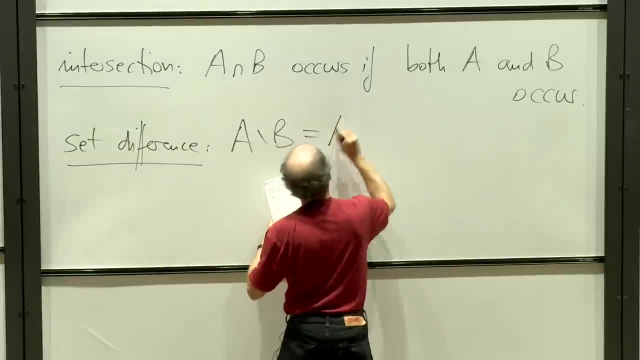 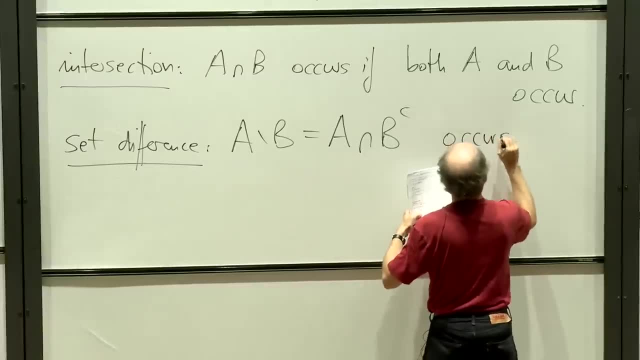 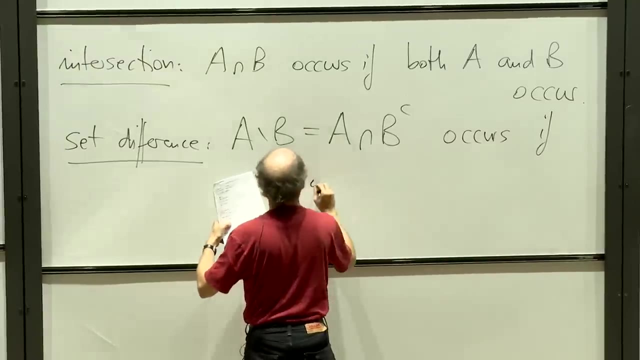 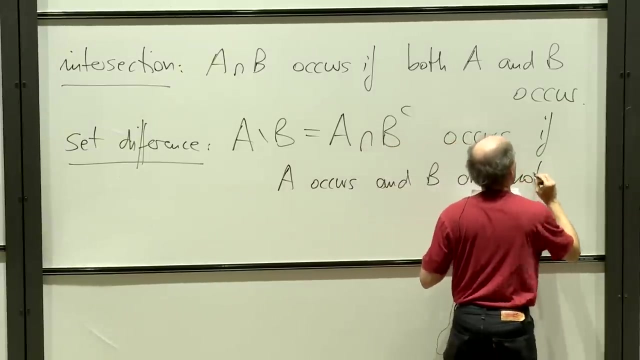 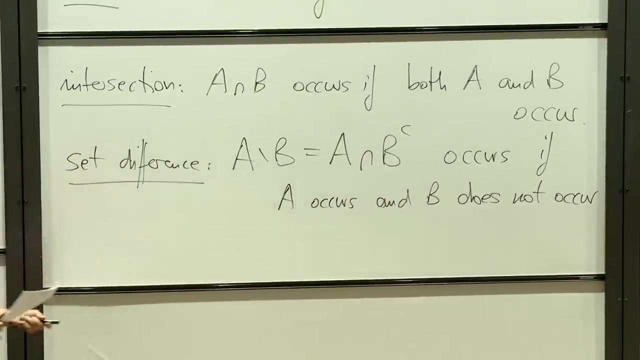 we can define in terms of what we've already defined as A intersection with B complement, And we can say this event, A minus B, occurs if A occurs and B does not occur. Okay, So here is set notation just what it means in terms of events occurring or not. 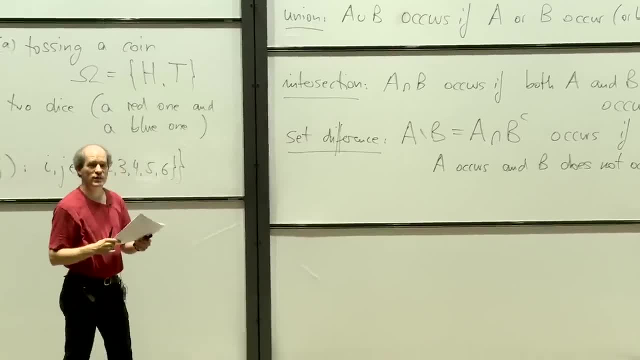 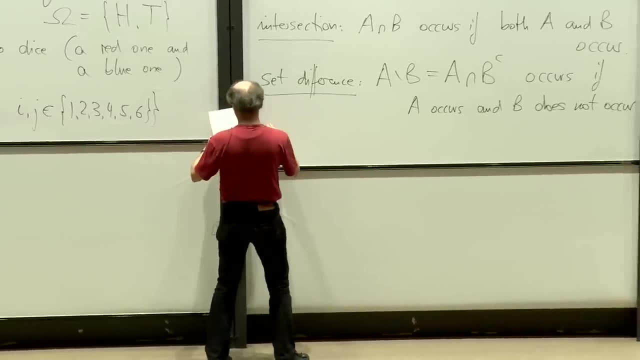 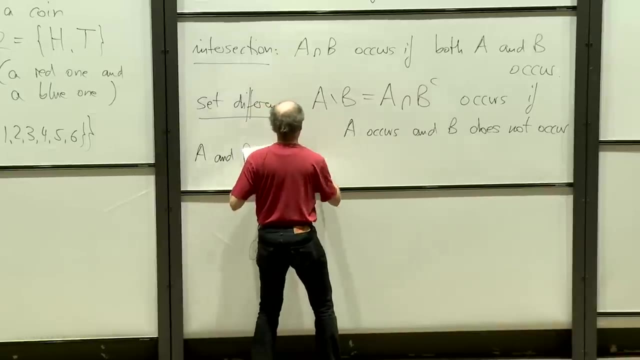 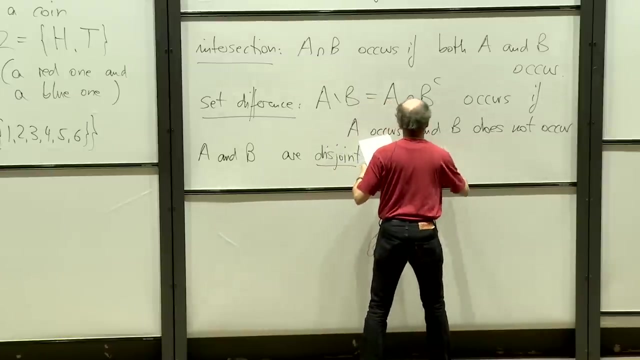 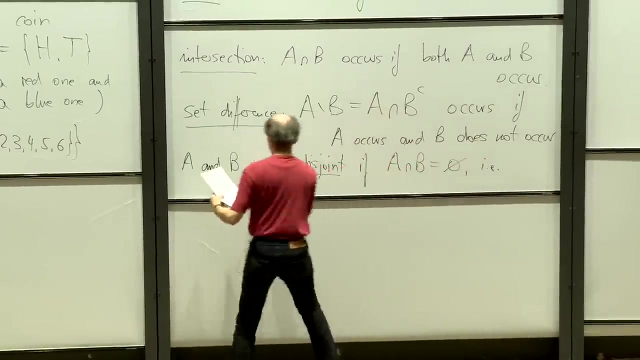 in our idea of representing experiments and outcomes in this way. So one more notion here: A and B as sets or indeed as events. in our context we call them disjoint if A intersection B is the empty set, ie A and B. 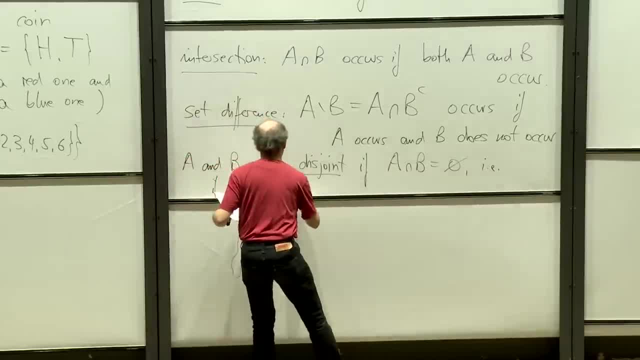 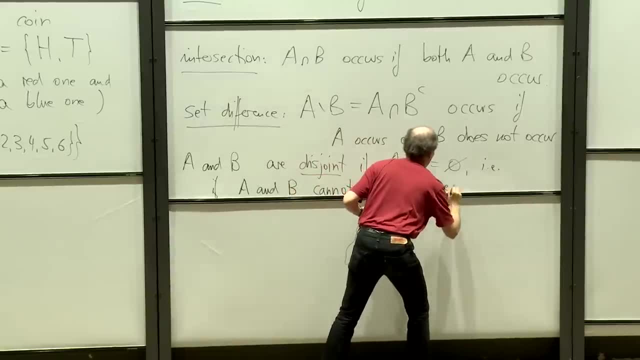 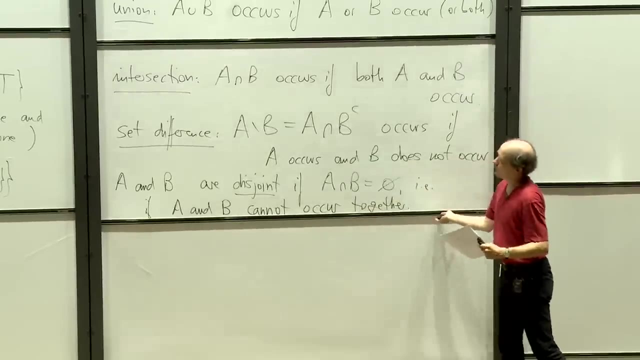 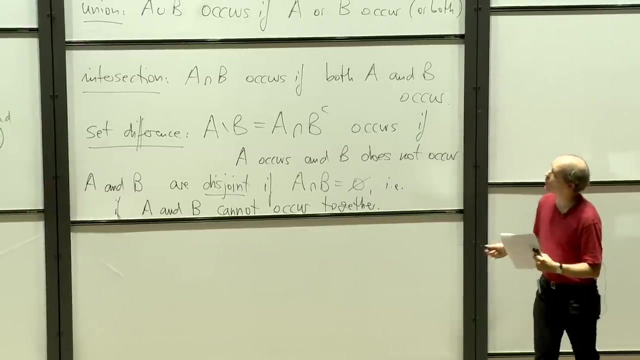 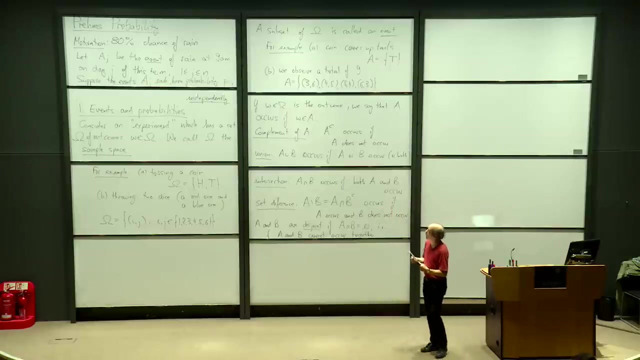 well, let's say if A and B cannot occur together. Okay, So that's a bit of set notation. We were on our quest of defining a probability model, So I've made sense of what it means to say: let A, j be the event of rain. 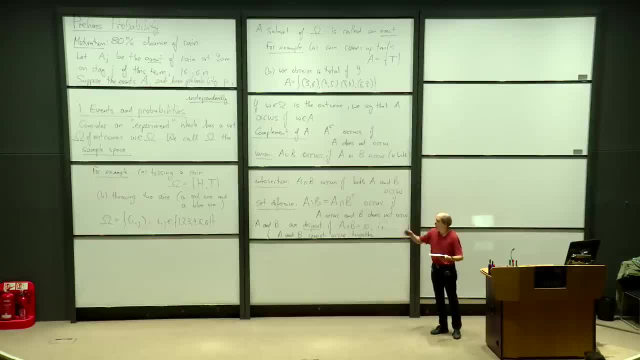 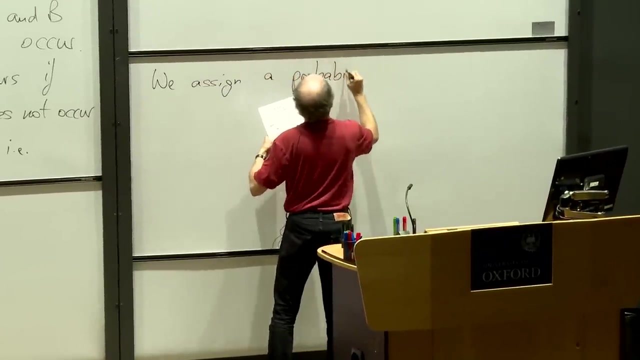 at 9 am on any particular day. I can use suitable sets to represent that, But now we assign probabilities to these events, and so that is our next general task. Now we assign a probability that we denote by P of A. 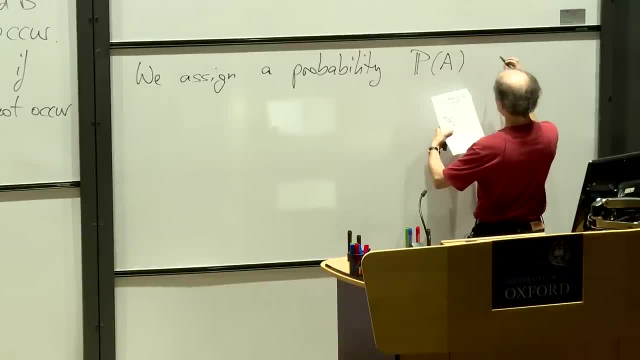 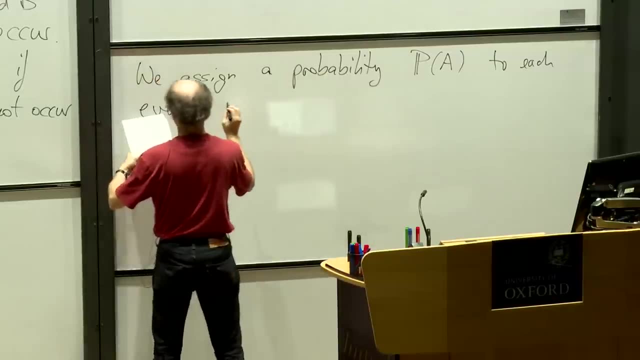 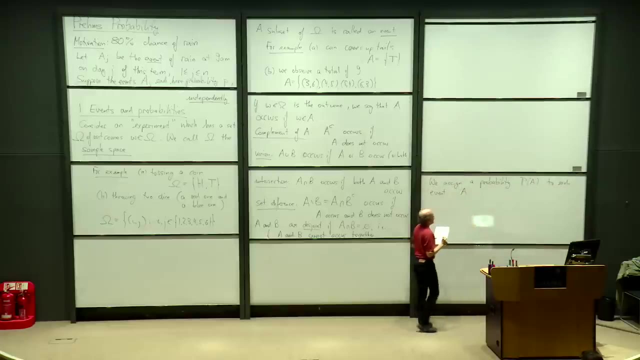 with a double bar. so to each event A, and that's kind of a little bit too general for a general definition and I think in any case I'm postponing the general definition of what is required here to Friday, For today I'd like to restrict to the simplest case. 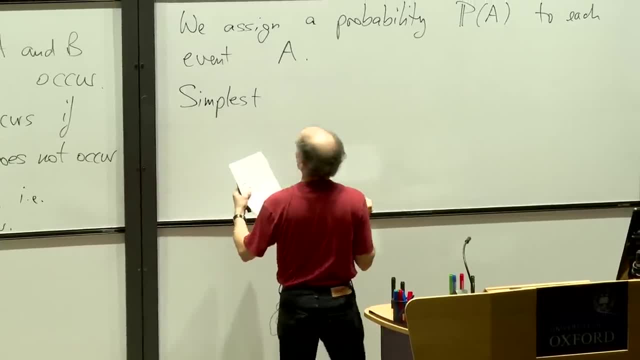 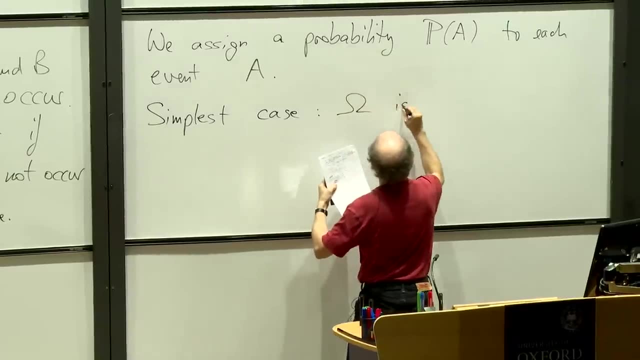 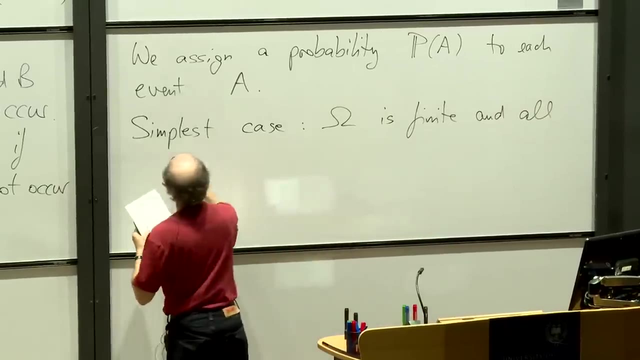 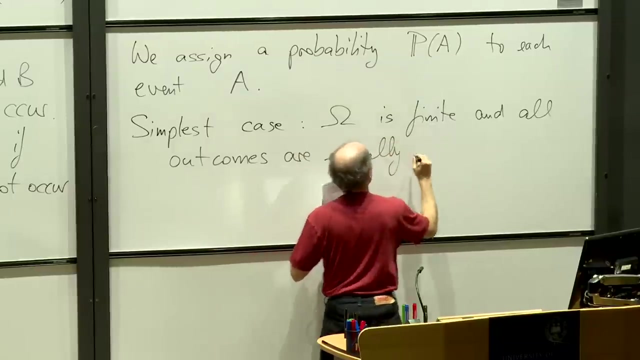 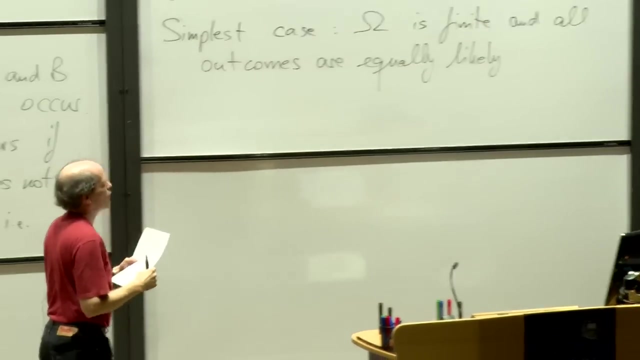 that is relevant to our two examples of throwing dice and coins. So the simplest case is where omega is finite and all outcomes are equally likely. Now, outcomes are the little omegas, events are the collections of omegas, subsets of capital, omega. 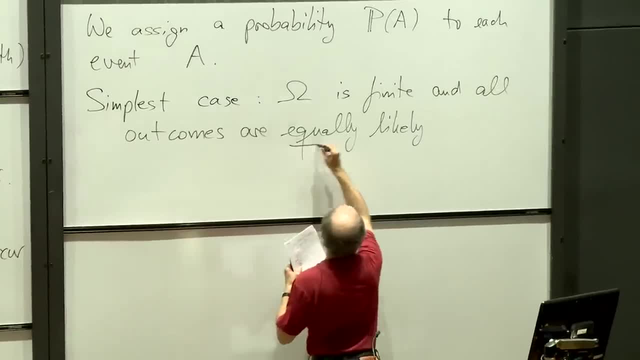 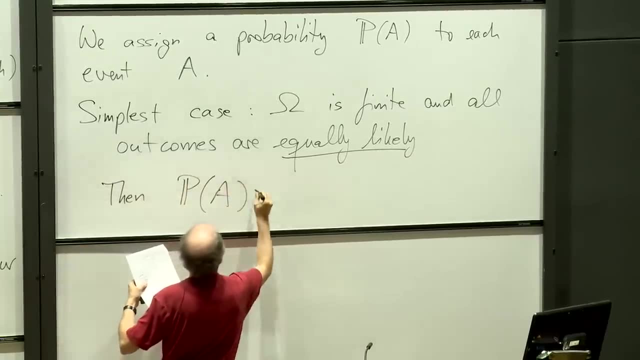 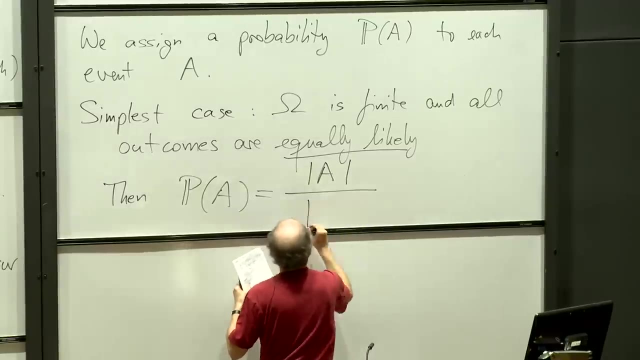 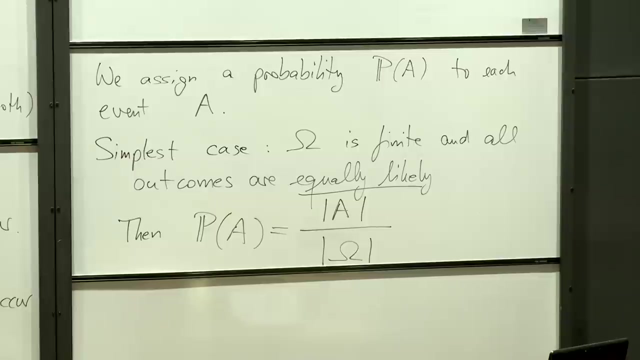 and so the consequence of the little omegas all being equally likely is that the probability of any event A is proportional to the number of elements. So number of elements of A, and that needs to be divided by the number of elements of omega, for the simple reason that 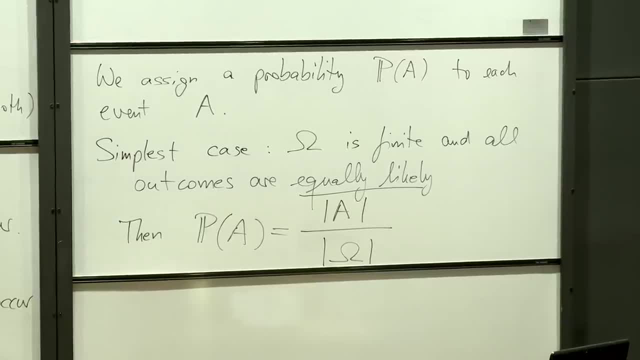 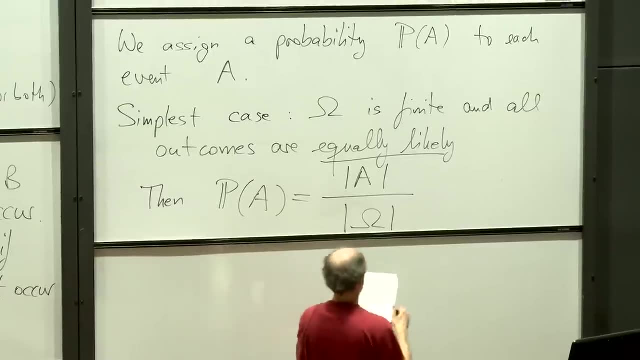 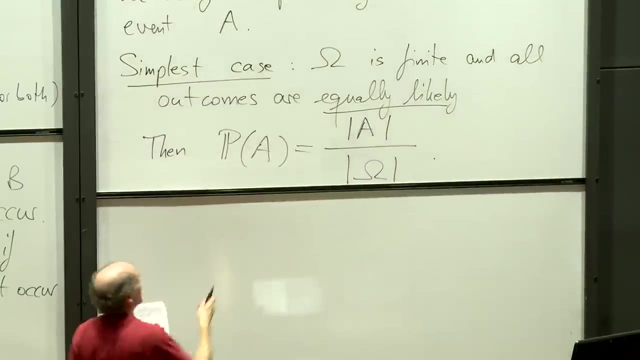 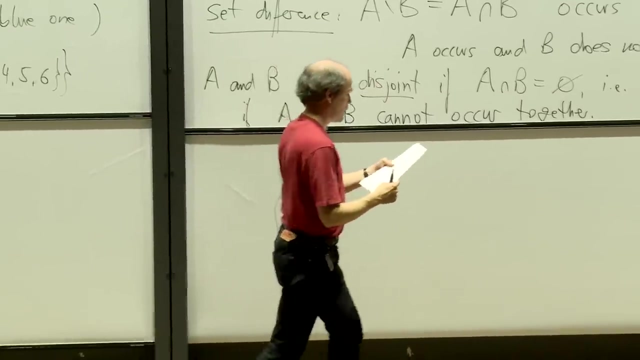 one of the outcomes has to occur, And so if you take A equal to omega, you want to get a one out of this. So that's our simplest case of a sample space that is finite and a probability assigned that is making every outcome equally likely. 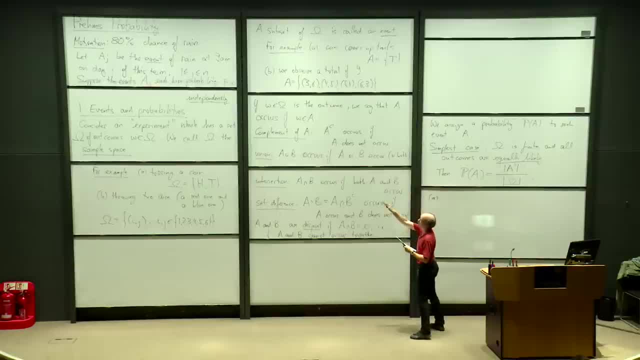 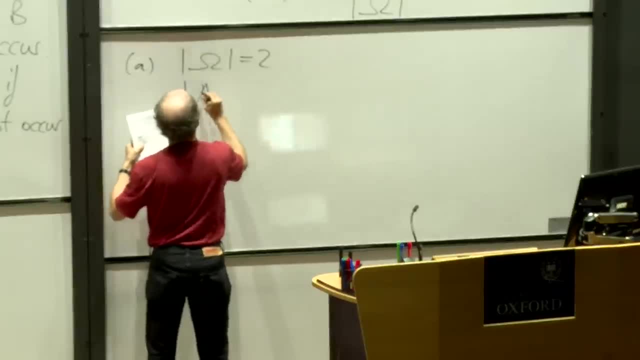 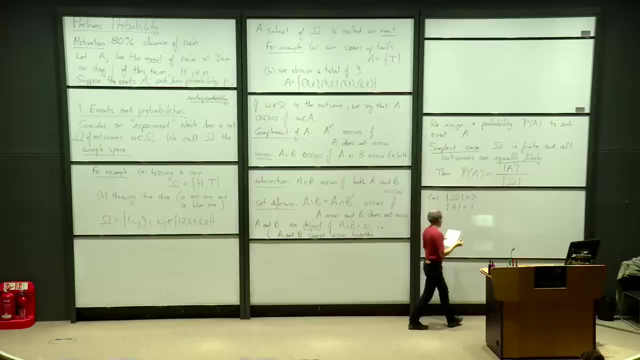 So in our examples A and B from over there with the coin toss, to begin with we have a sample space of size 2. We defined an event, that we observed tails, which consisted of the single outcome tails, And so we can then conclude. 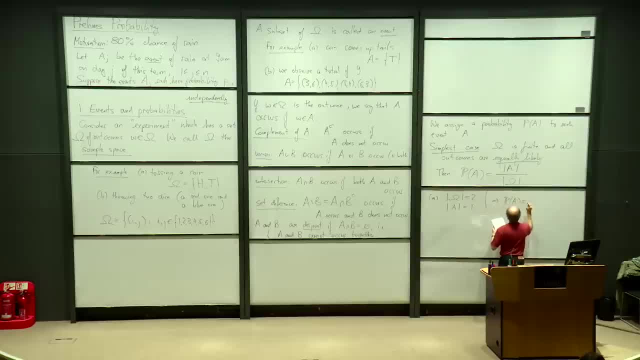 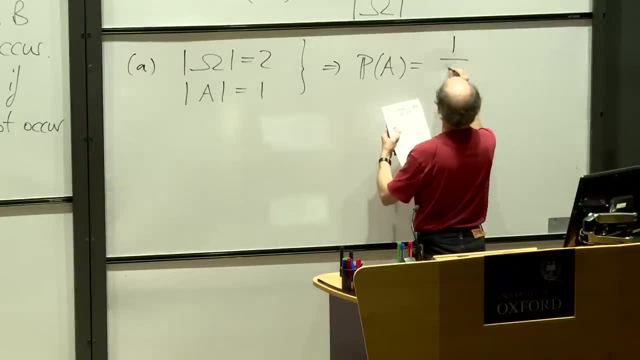 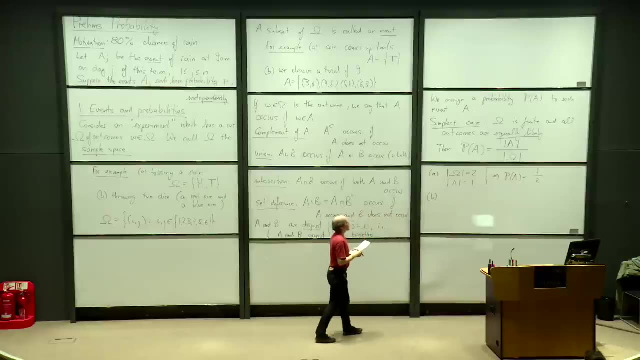 that with this definition, and certainly in a natural way anyway, the probability of observing tails from a coin toss is 1 divided by 2, one half In the second example, where we have two dice and this set of outcomes that have a sum of nine, 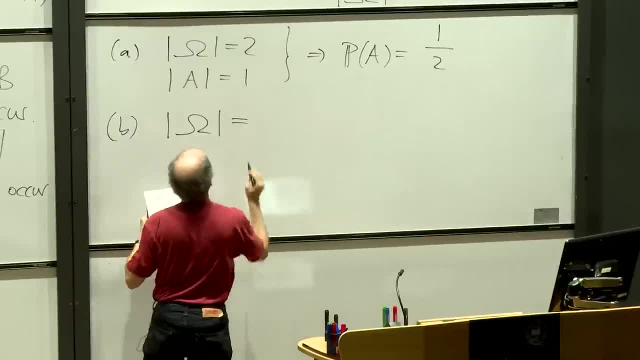 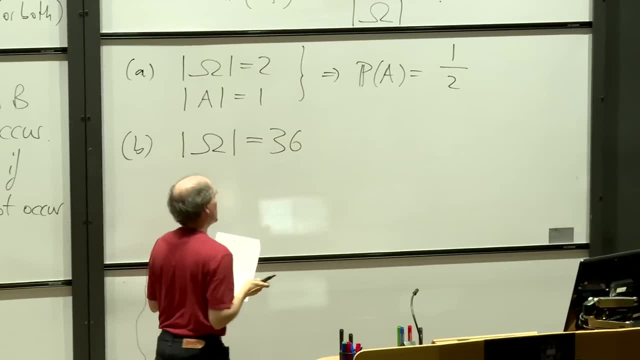 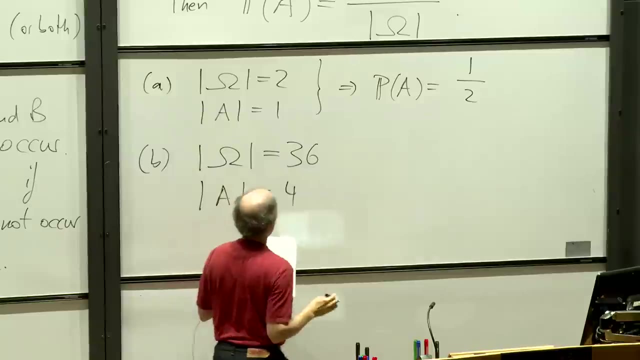 we have a sample space, omega, where every combination of two numbers, one up to six, is possible. That makes it 36 possible combinations, And the event that we've written out explicitly clearly has four elements, And so in that setting the probability of our event. 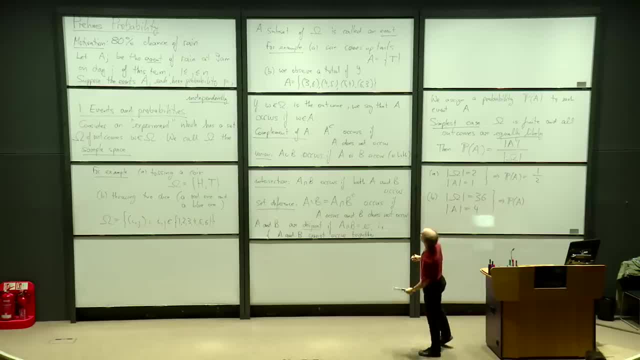 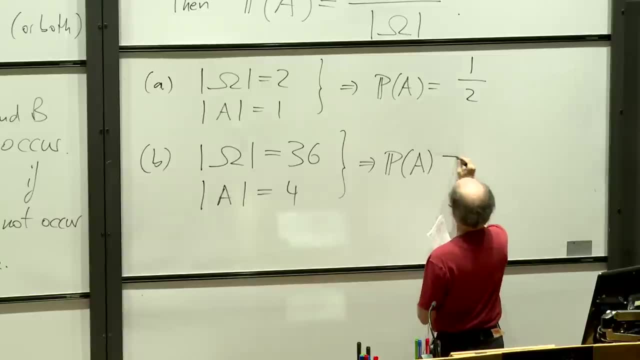 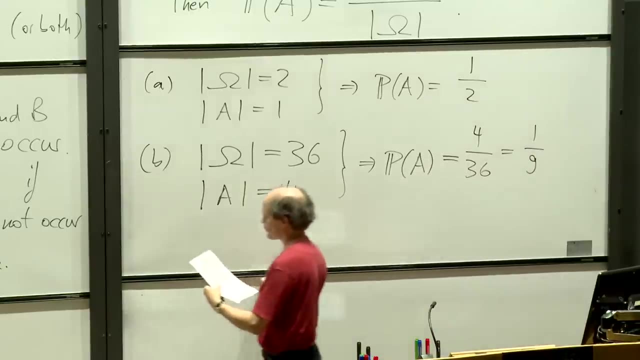 did I call it A or B? Up there it's again A. So that event has a probability of 4 divided by 2.. 4 divided by 36, and that is one ninth In the second example. I mean it's still a simple example. 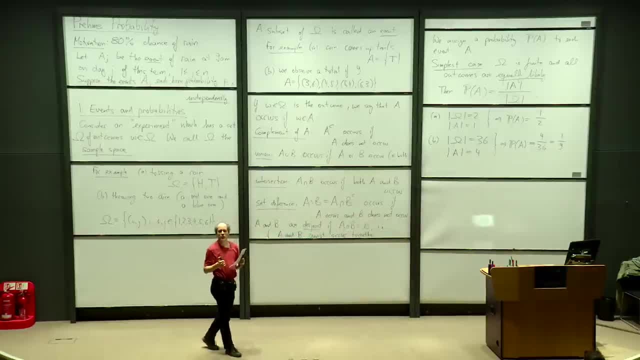 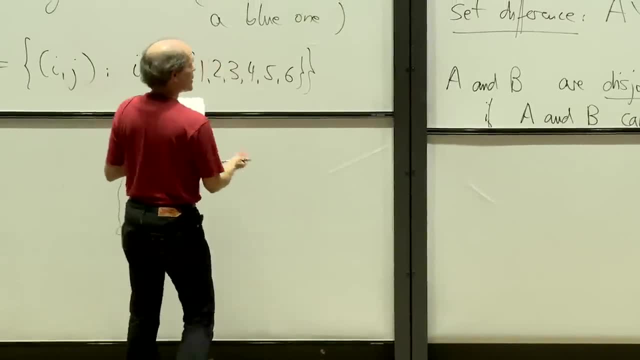 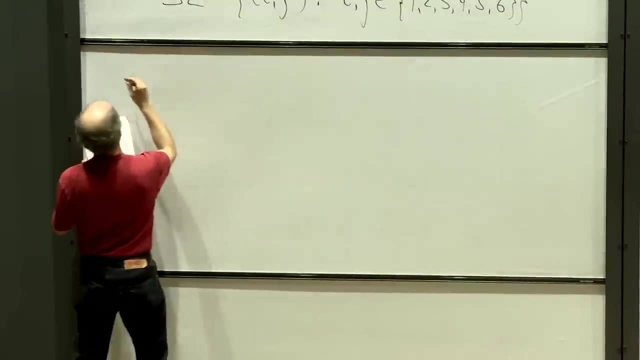 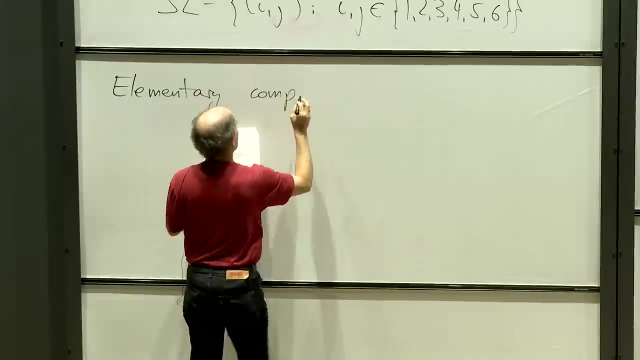 but you can kind of see that calculating probabilities in the setting where all outcomes are equally likely involves counting, And counting is a topic that merits a little more discussion here in some generality. So let us start with some elementary combinatorics. Combinatorics is the mathematical discipline. 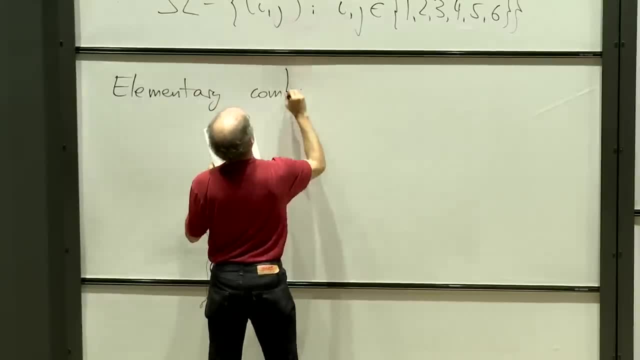 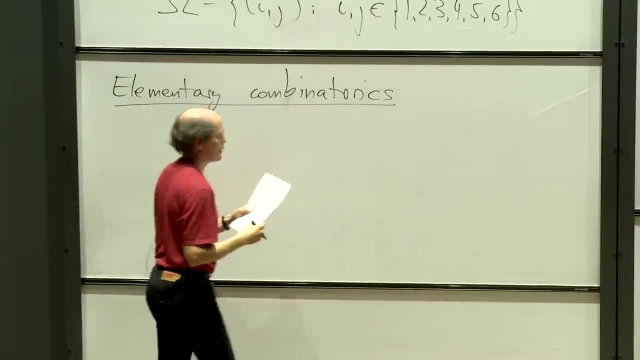 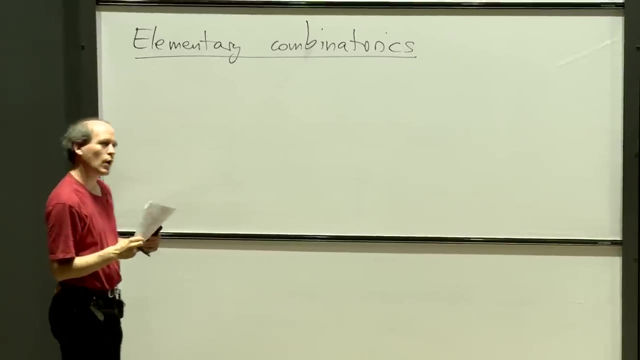 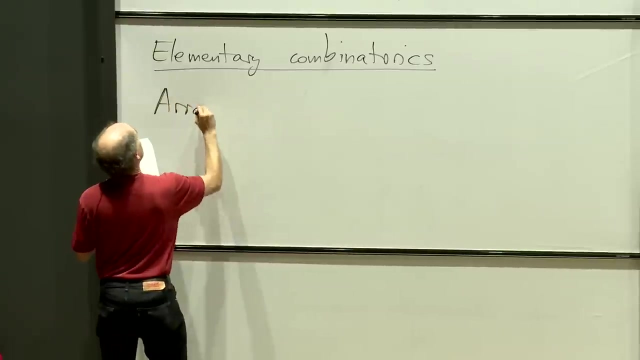 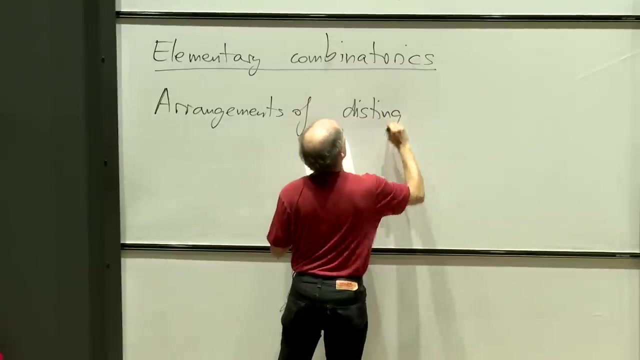 of counting in some sense, And you can count lots of different things. A kind of useful discussion for us today is to look at what's called permutations or numbers of arrangements of objects, And let's start with arrangements of distinguishable objects. So they are all different. 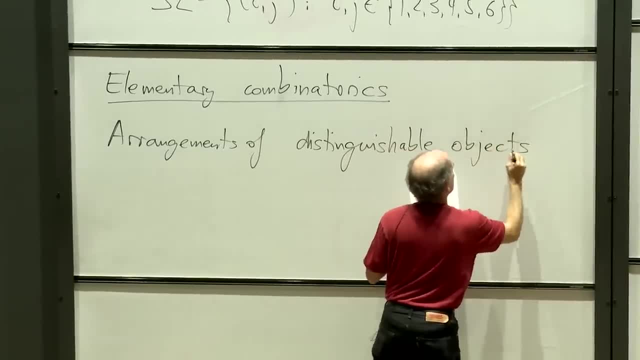 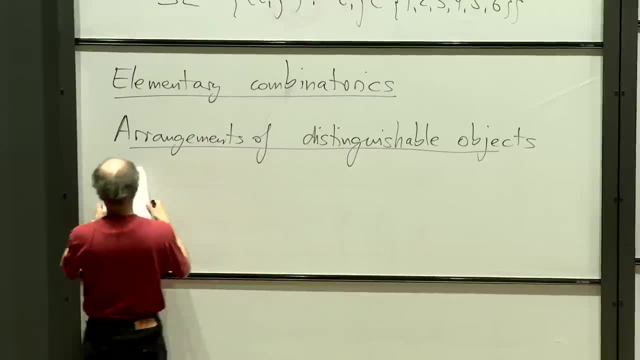 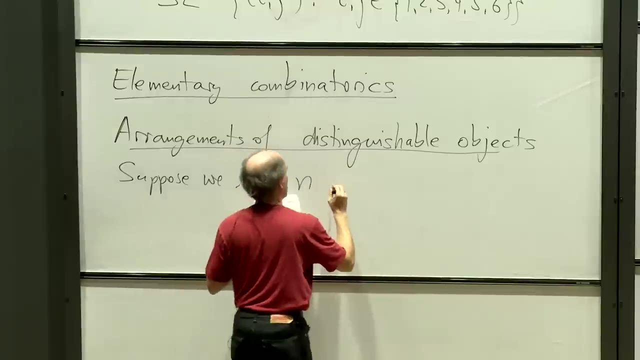 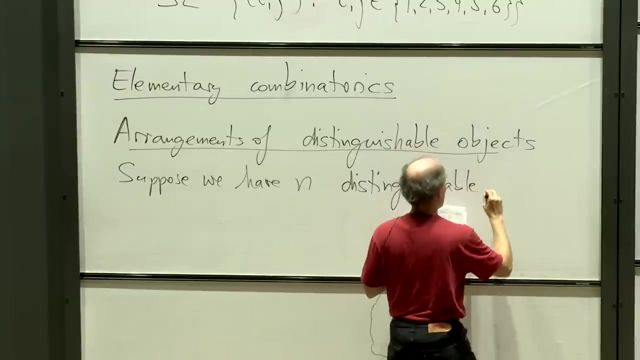 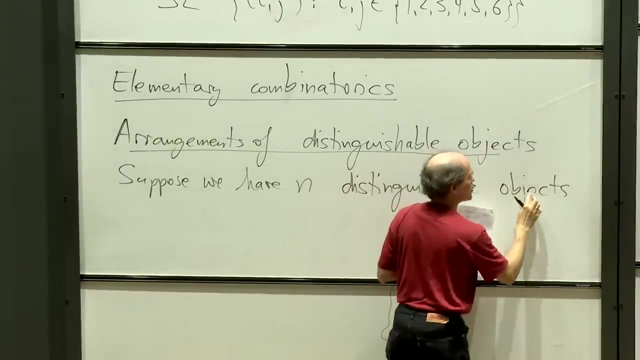 And you want to bring them into an order, arrange them in a particular order. So suppose we have n distinguishable objects, For example the numbers 1 up to n, But some of this phrasing suggests that this is actually more general than that. 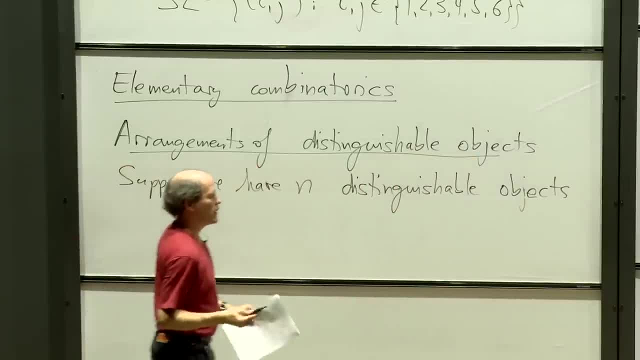 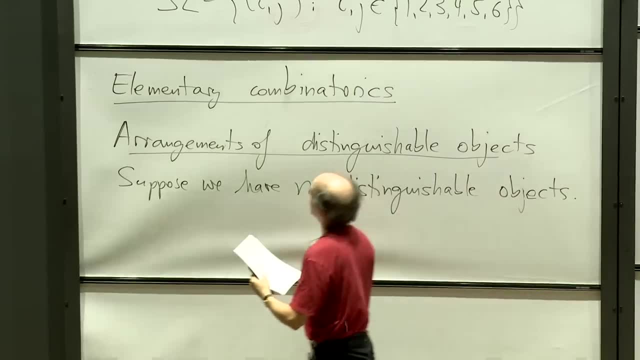 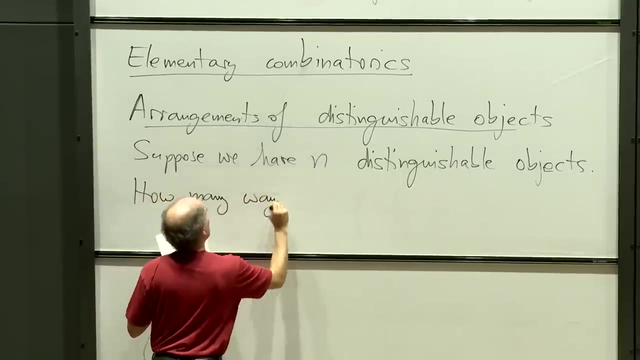 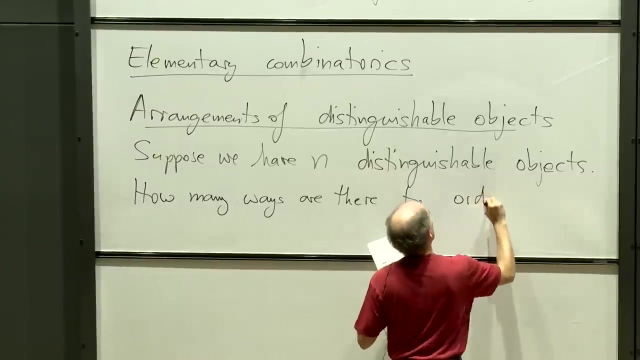 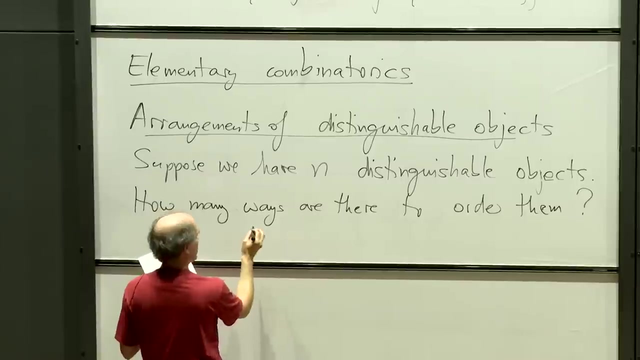 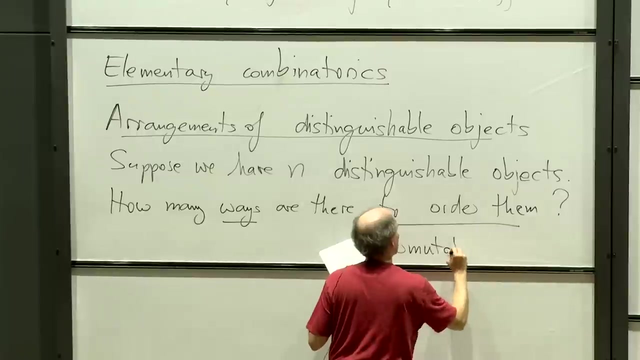 And so we don't need to be very specific here. Any n distinguishable objects feed into the following discussion. We can ask: how many ways are there to order them? OK, And a way to order them is a permutation. So, for example, 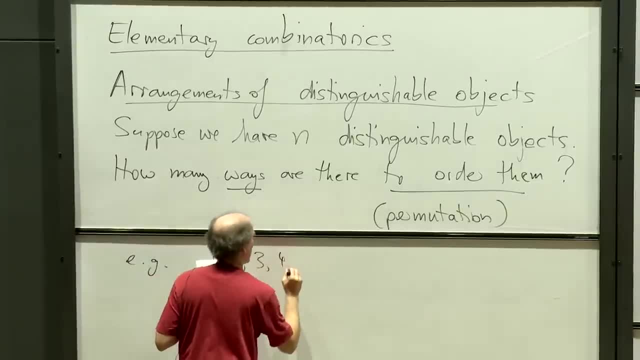 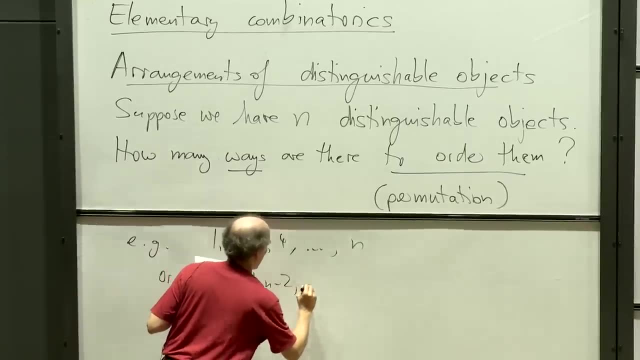 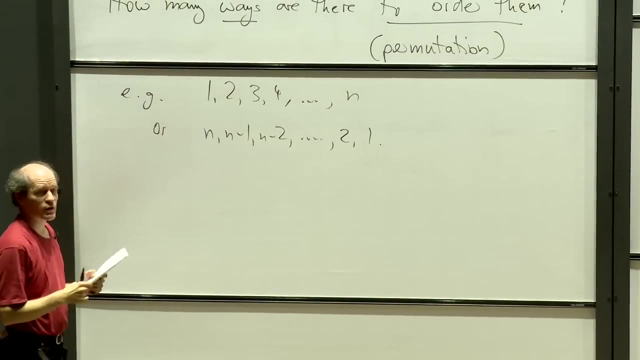 you could just have them in the order 1 up to n, Or you could have them in the reverse order, But of course there are many other orders And the question that's being asked here: how many are there? And in order to work that out, 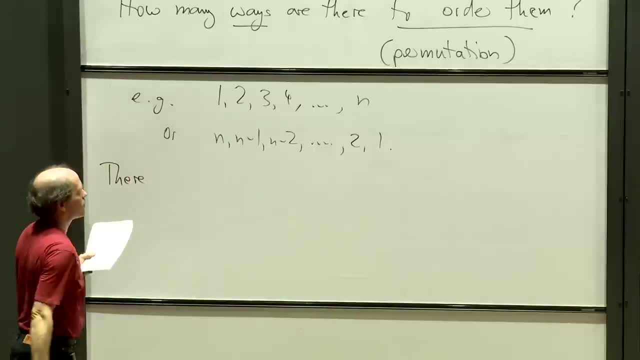 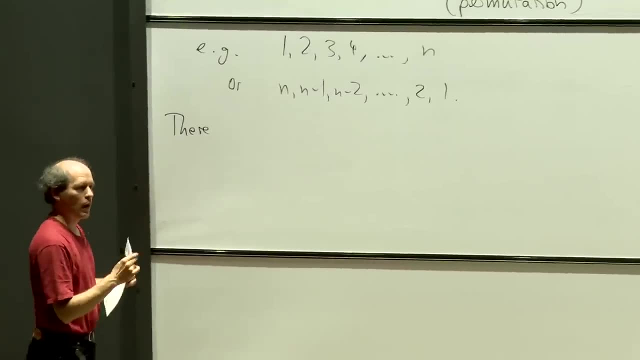 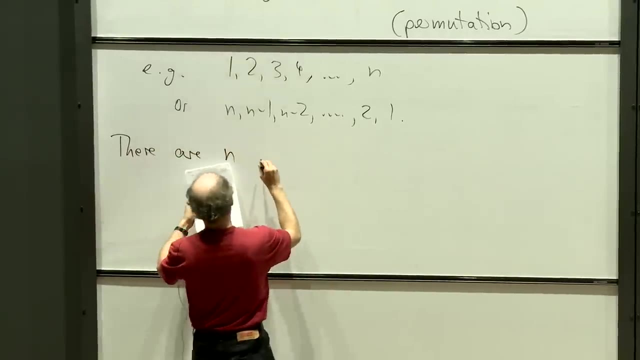 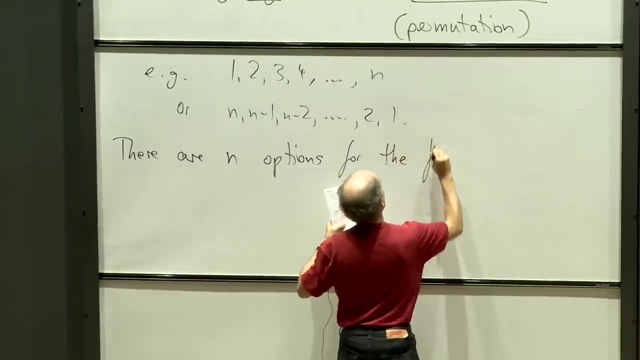 you can kind of start at the beginning If you want to list them all in an arbitrary order. we can first wonder how many possibilities are there for what we put into the first position, And there are clearly n options for the first object. OK, 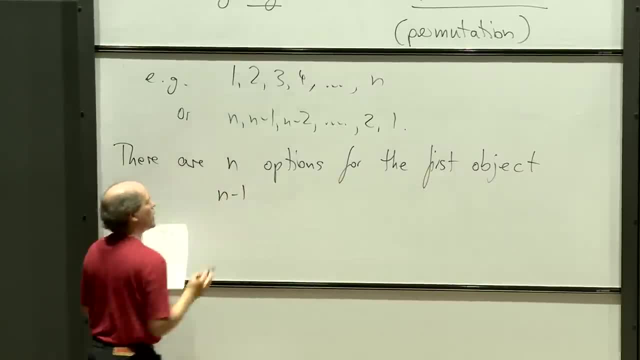 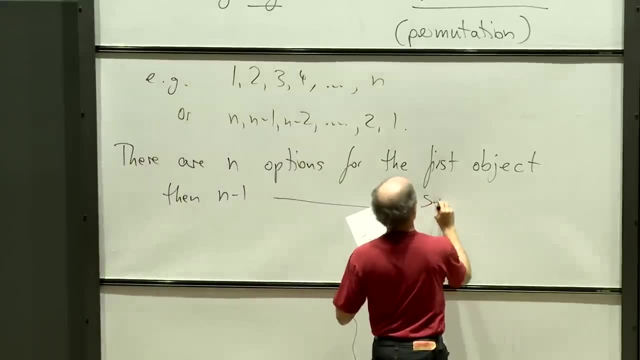 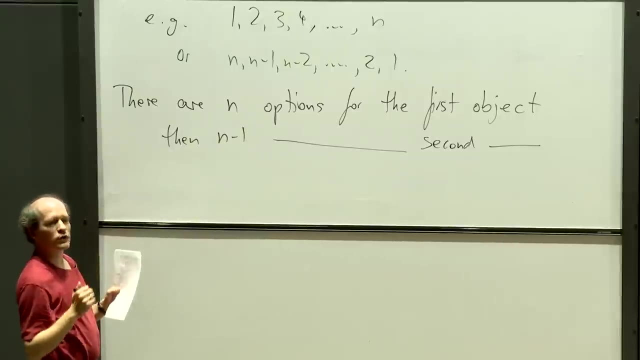 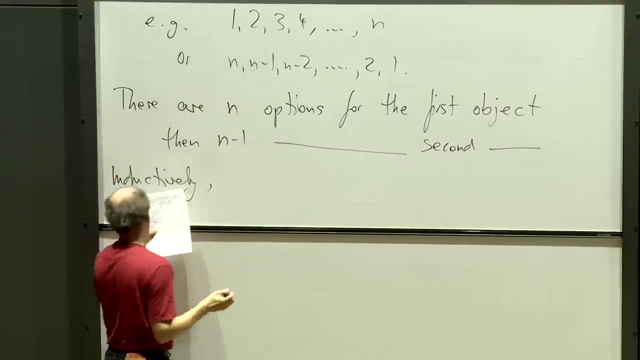 And once you've chosen the first object, there are n minus 1 remaining options for the second object. OK, And then, after you've done this a few times, you can argue inductively And notice that if you've already chosen your first m objects, 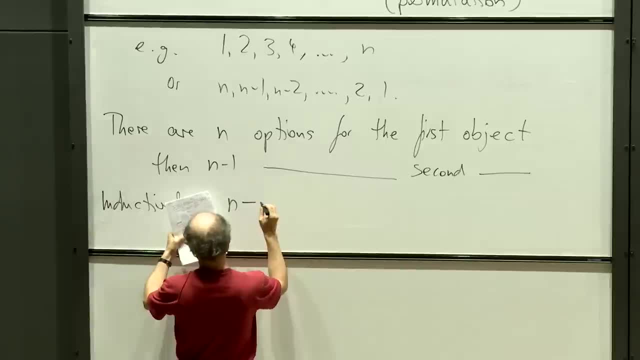 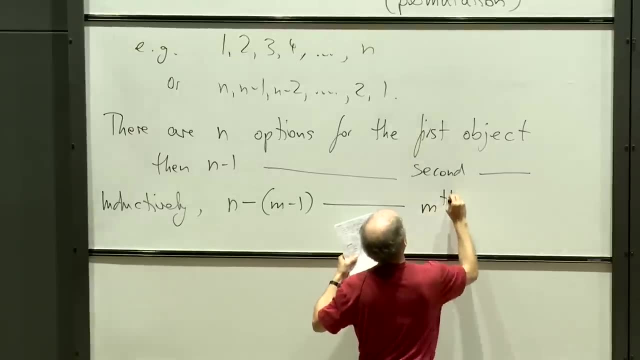 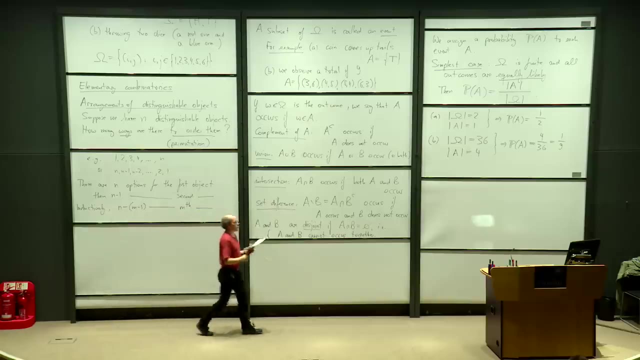 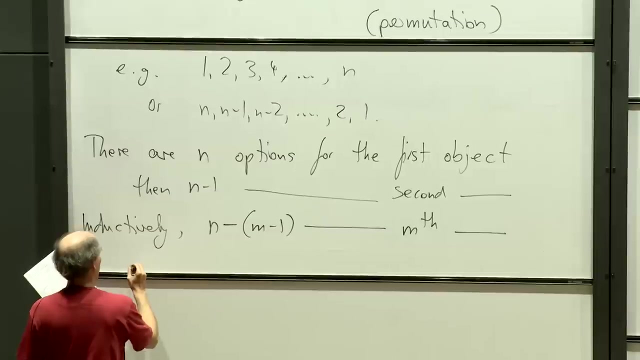 or say m minus 1 objects, then there will be n minus m minus 1 remaining to choose from for the mth object. OK, And if you like this kind of generality here with the m, then that's great. But let me just write: 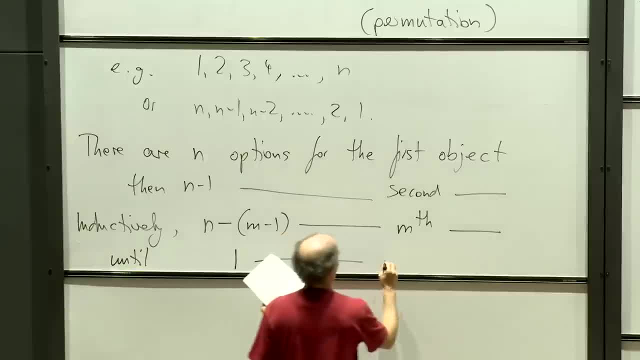 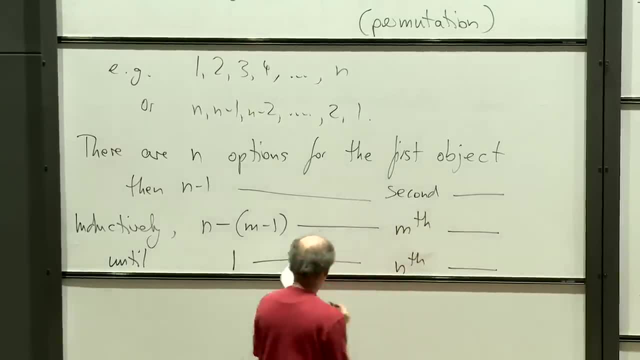 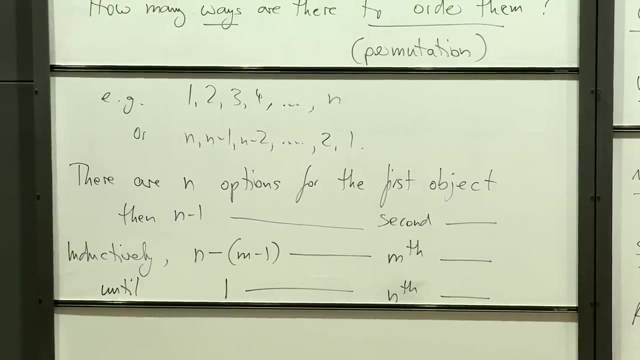 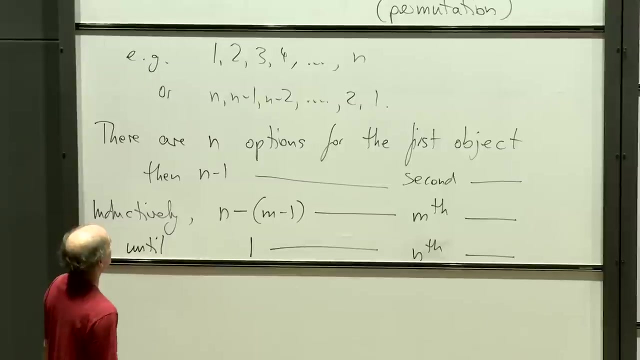 until there is only one option for the last Object, Or let me say the nth object. But the word inductively is kind of a powerful word, because it kind of suggests that you can be completely rigorous about this If at this stage you prefer to say: 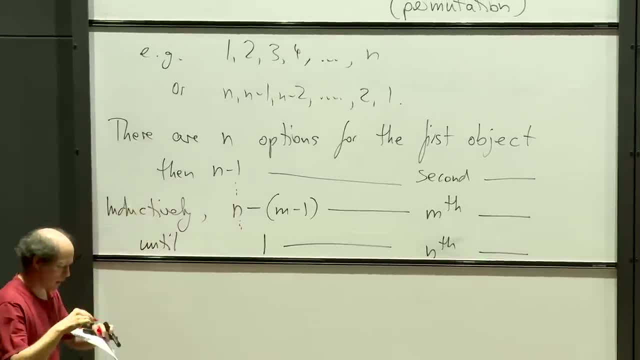 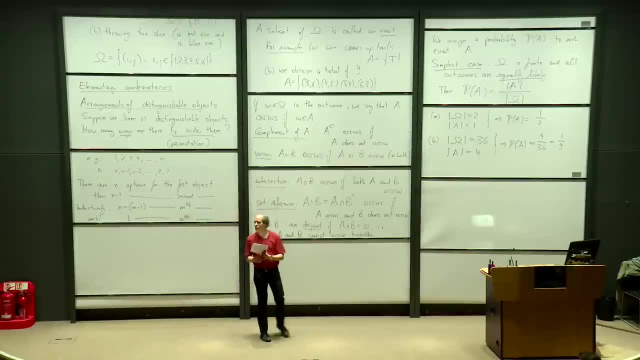 well, let's just put dots in between. that will still be fine, I think in this course certainly, Whereas the mathematicians among you, on the pure math side of the degree, will be told that maybe dots are to be handled with great care. 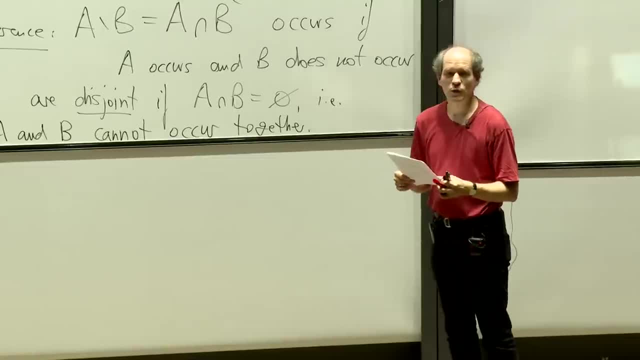 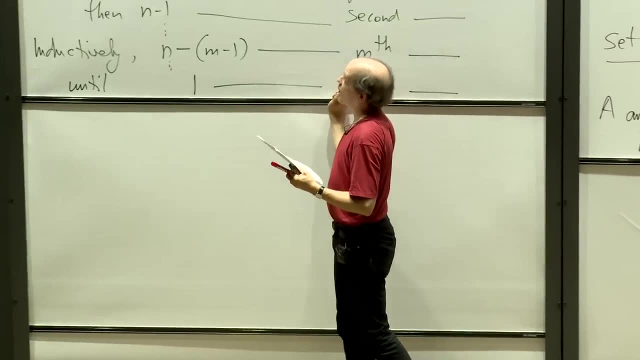 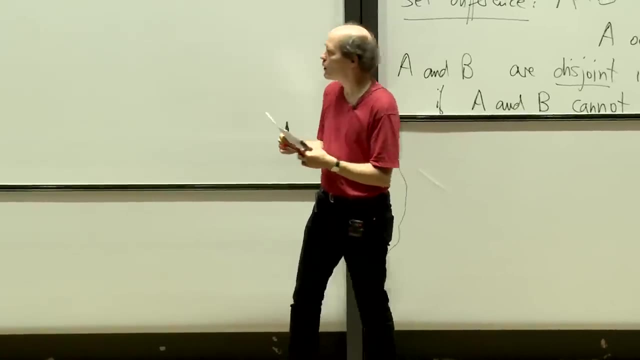 And we want to kind of handle dots with some care here as well And ultimately, anything that you write with dots and is a valid argument actually probably can be written out as a proper induction, And hopefully without too much effort, but with effort that you don't want to spend. 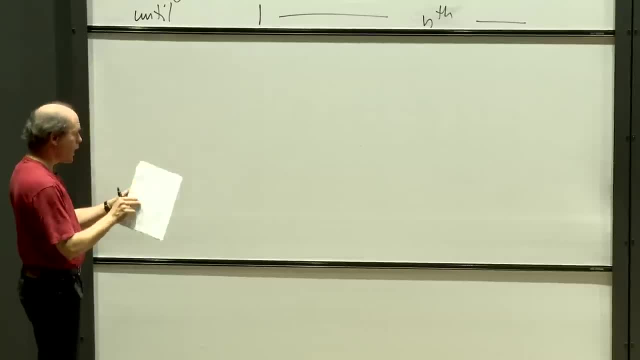 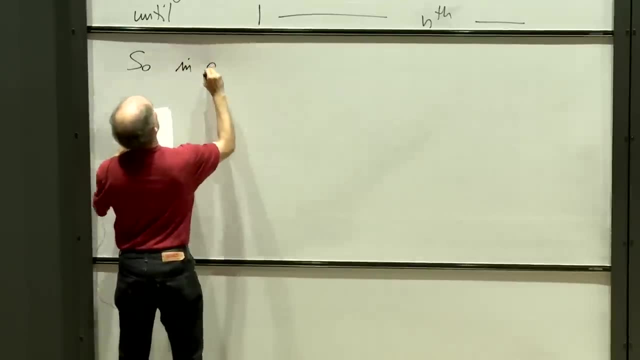 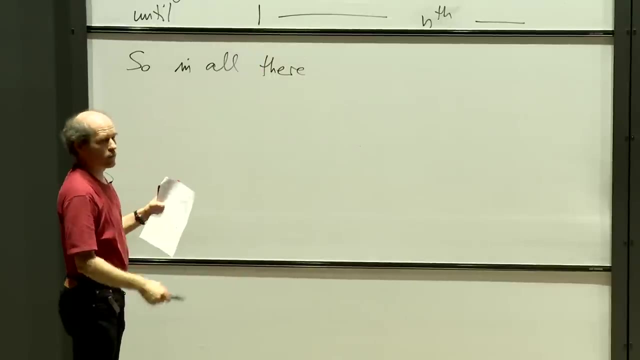 Every single time. Anyway, the conclusion for us here is: in all, we can put all this together to obtain the number of choices that we have here, And there's one more thought we need to have, which is: what do we do to n? n minus 1,. 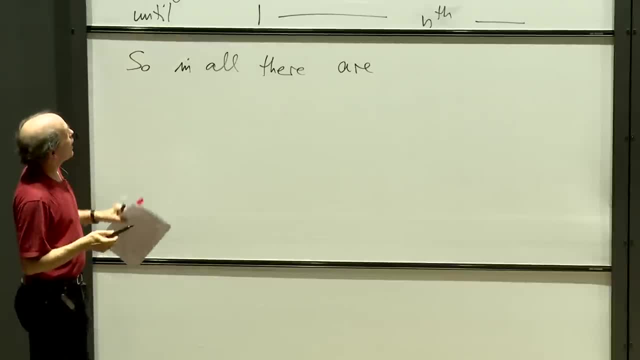 down to 1?. If you start at the top after the n options, for each one of those n options you have n minus 1 options. So altogether for the first two positions you have n times n minus 1 options. 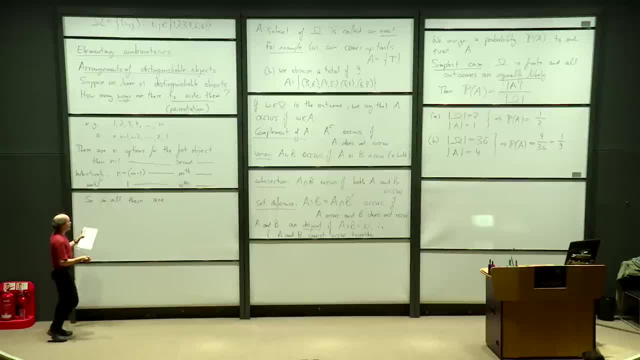 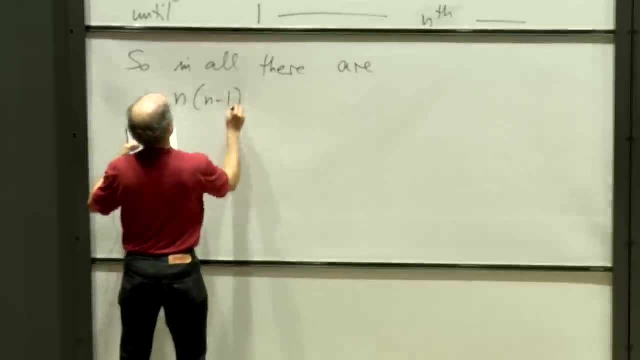 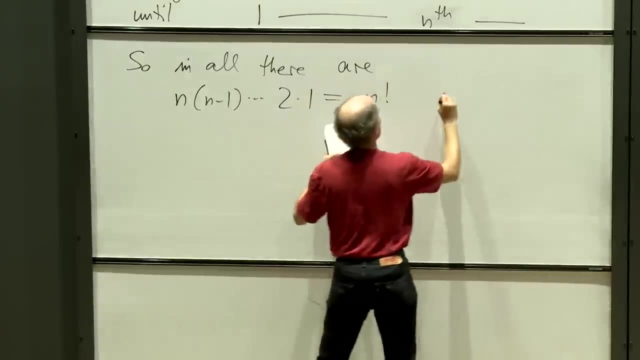 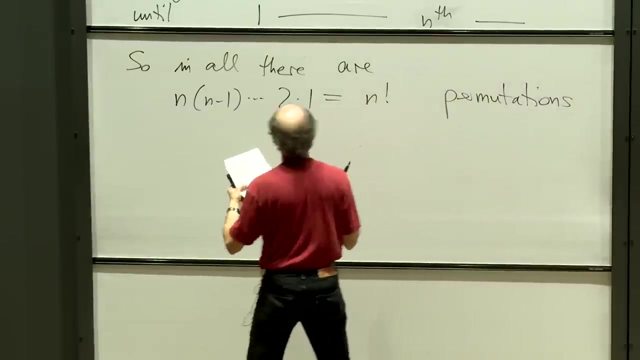 And the same reasoning applies inductively to say: you need to multiply all of these numbers. So together there are n into n minus 1, into 2 times 1, which is n factorial permutations. Let me write the word inductively here again. 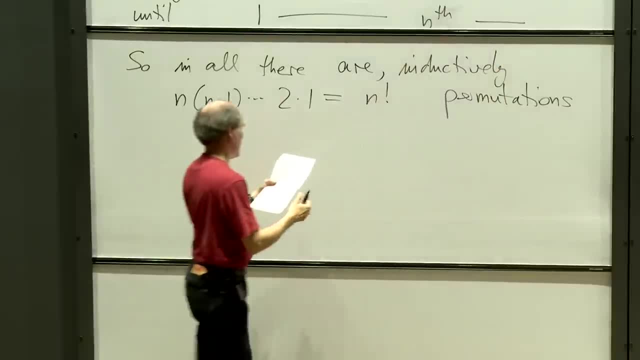 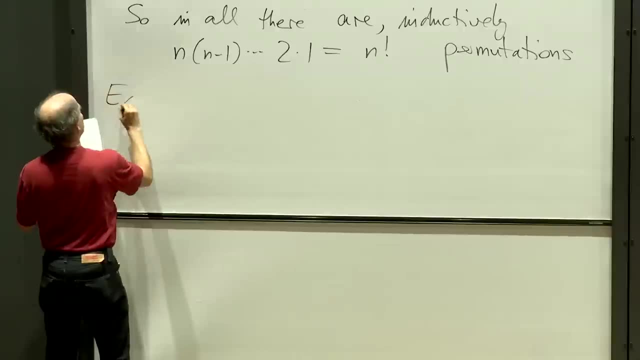 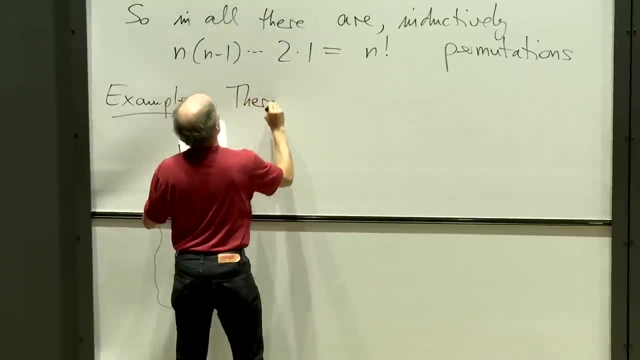 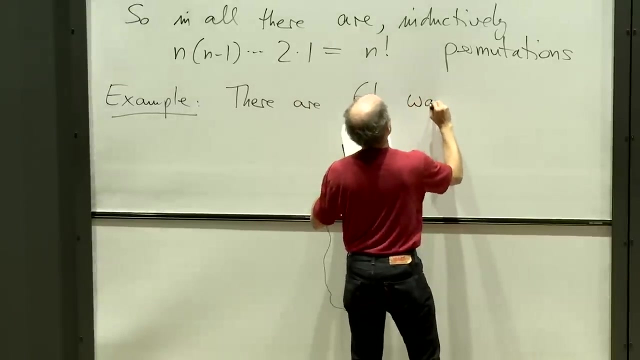 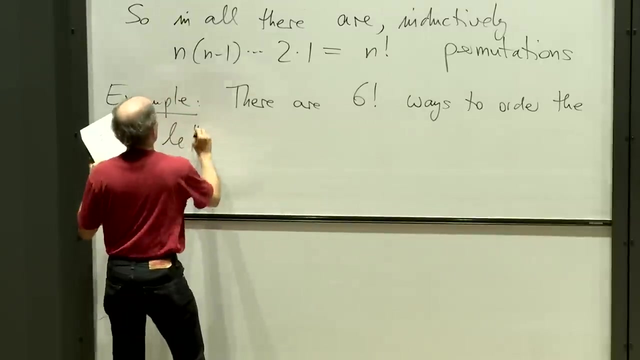 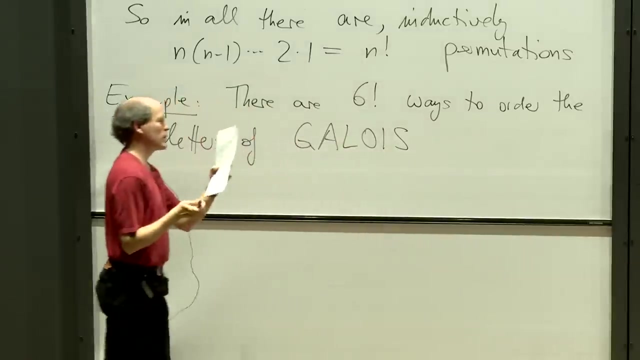 because, writing these dots, there is something that you can make more precise. So, as an example, there are six factorial ways to order the letters of a six-letter word, And let me use the word Galois here, which is a famous mathematician. 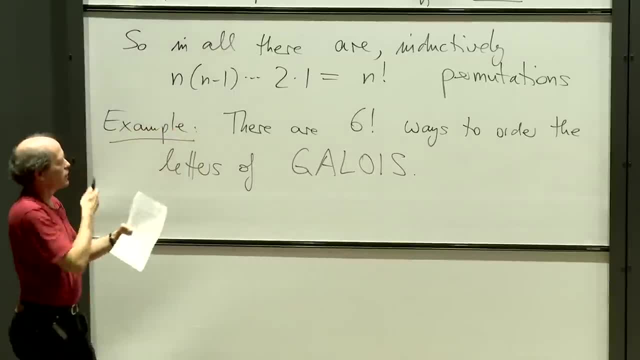 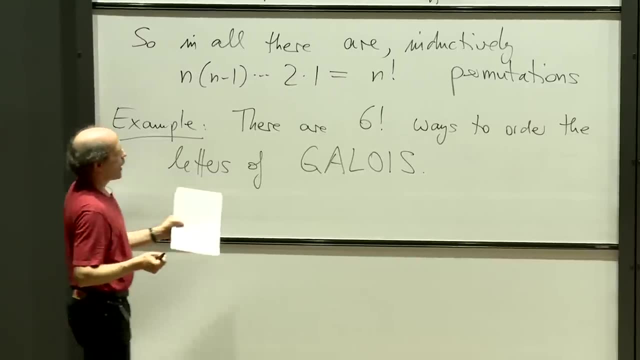 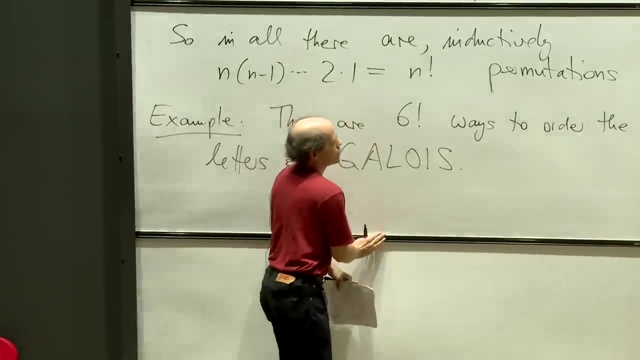 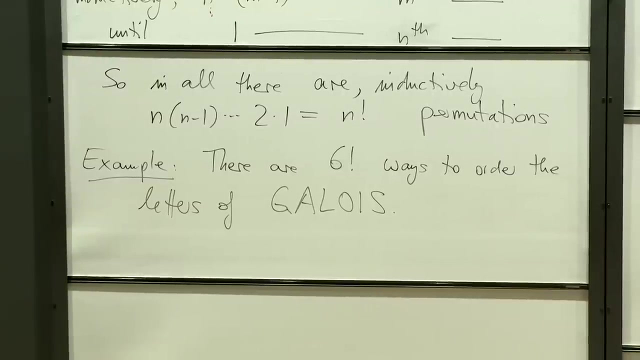 which, among his many distinctions, has the distinction that he has six different letters in his name, And of these six letters there are three vowels and three consonants. Now, that, of course, is not particularly specific to this name, but leading on to my question, 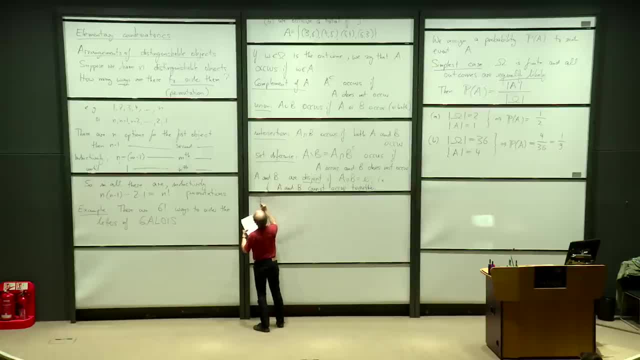 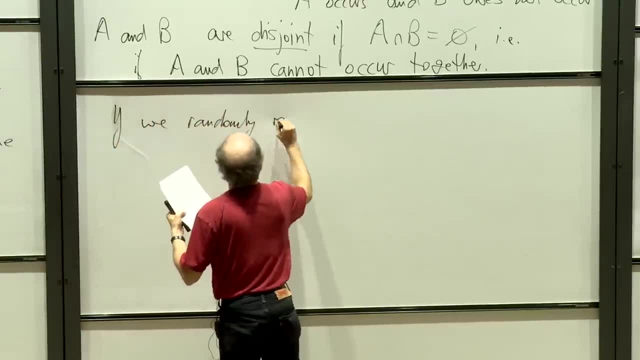 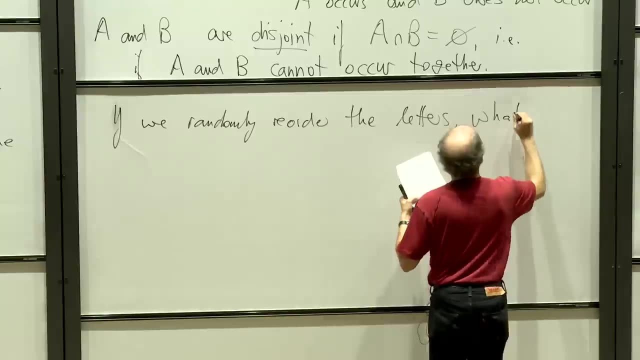 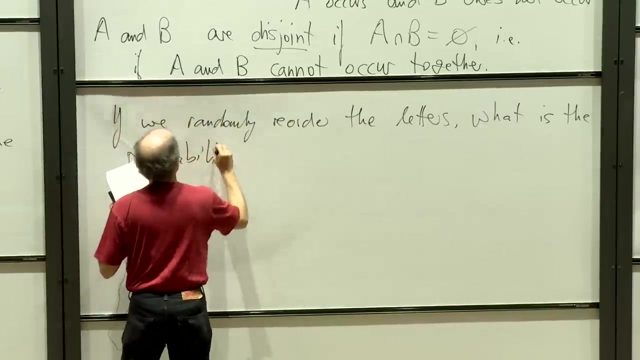 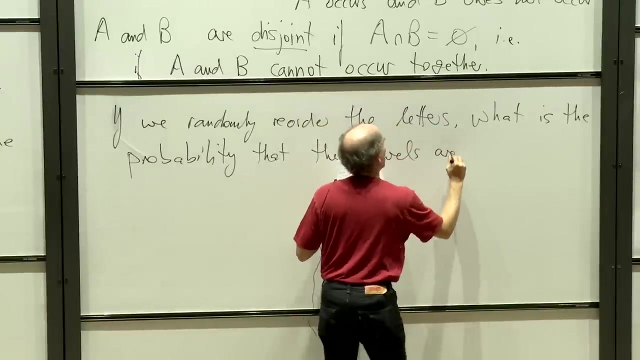 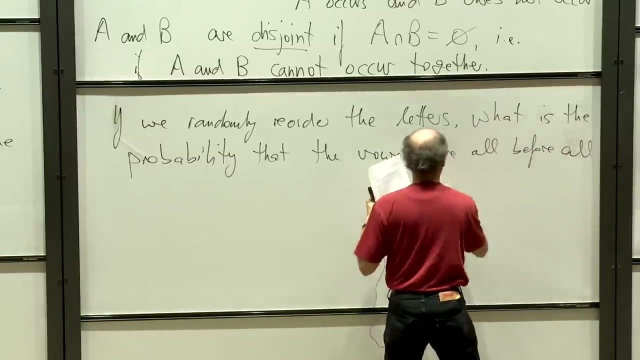 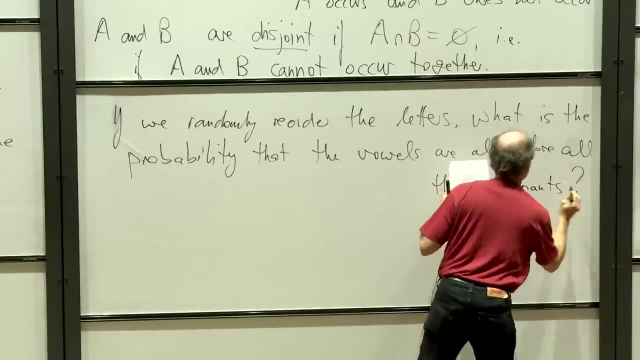 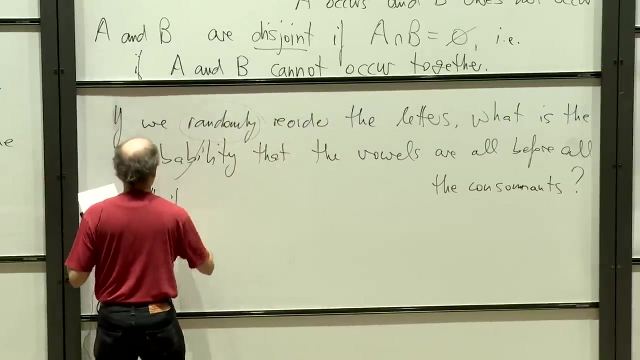 that I'm asking in this setting: if we randomly reorder the letters, what is the probability that the vowels are all before all the consonants? Okay, I've been a little sloppy here, So here what I really should say is uniformly at random. 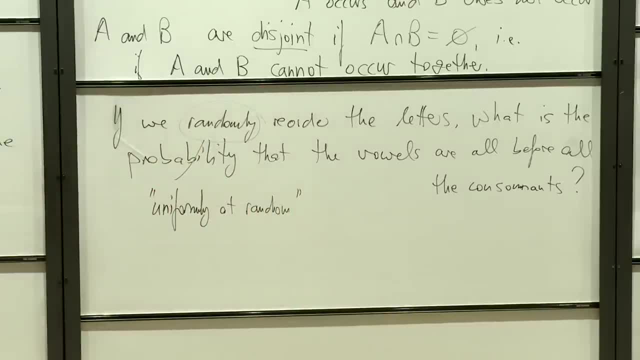 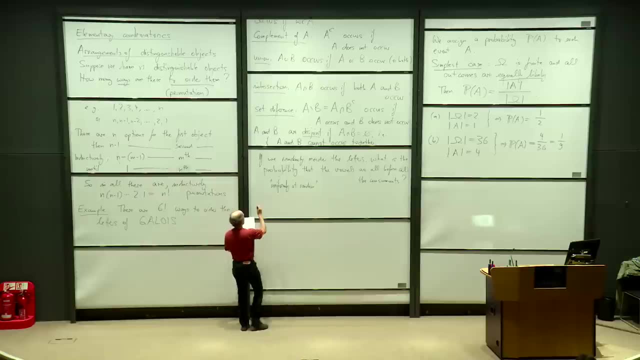 in the sense of what I've defined up there, all outcomes being equally likely, So all rearrangements here being equally likely, Then here's the answer: How many ways are there of achieving this event of having the three vowels before the three consonants? 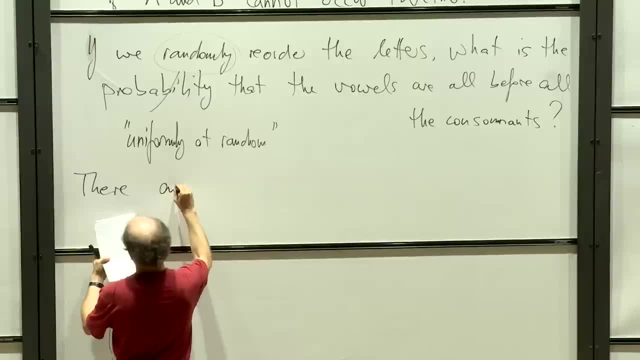 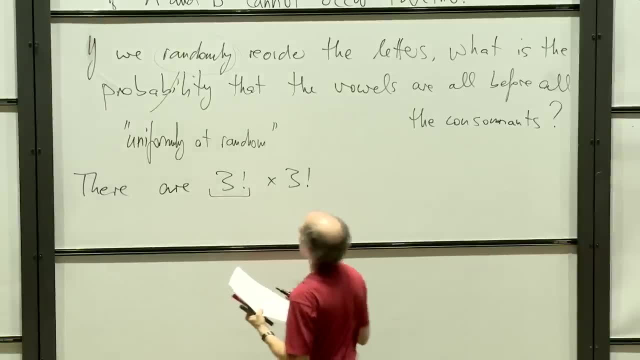 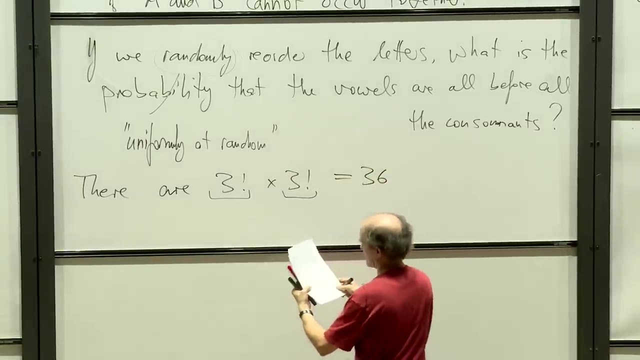 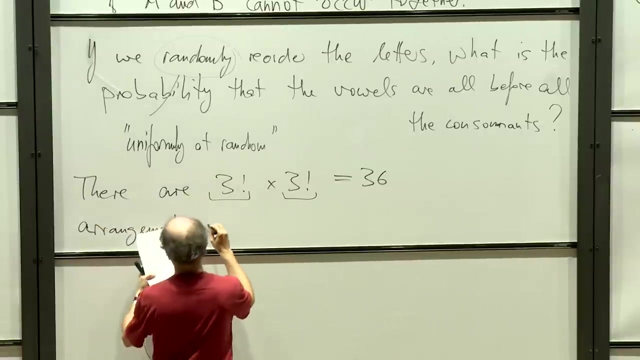 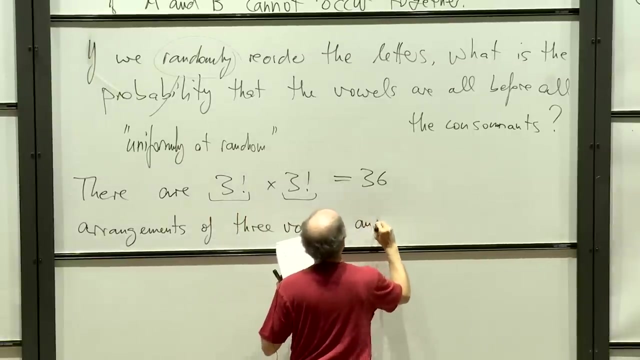 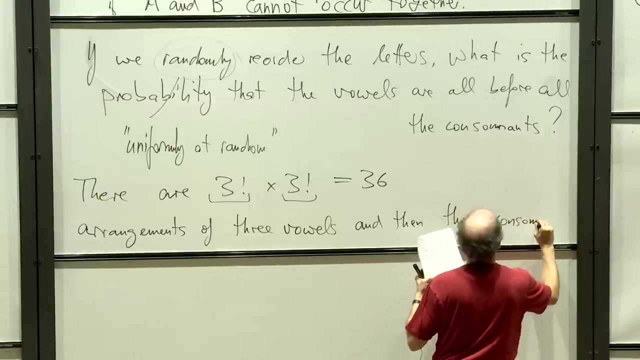 There are three factorial times, three factorial ways of first ordering the three vowels and then ordering the three consonants, And that gives us 36 arrangements, And what I've just said is of three vowels and then three consonants. Okay, So I've done some. 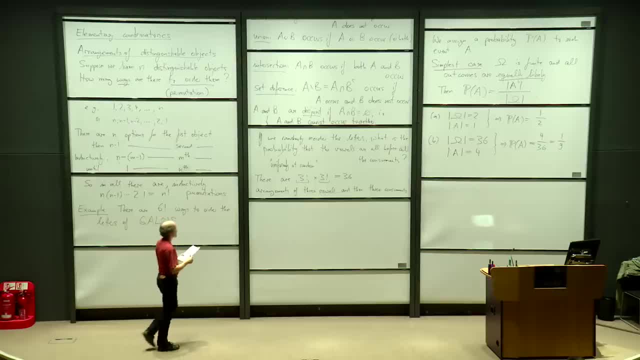 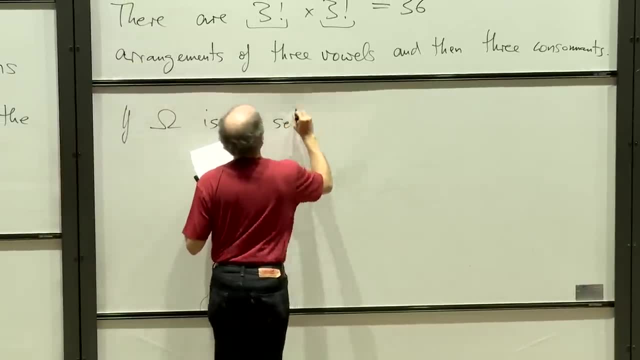 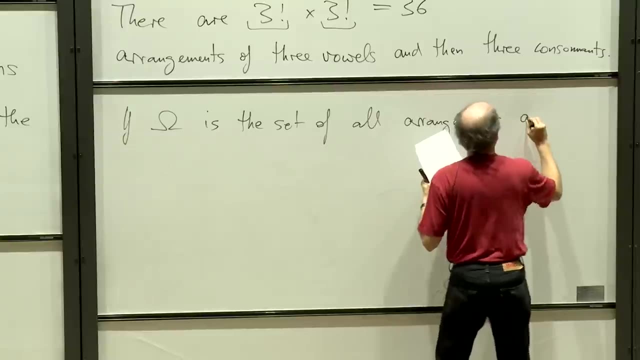 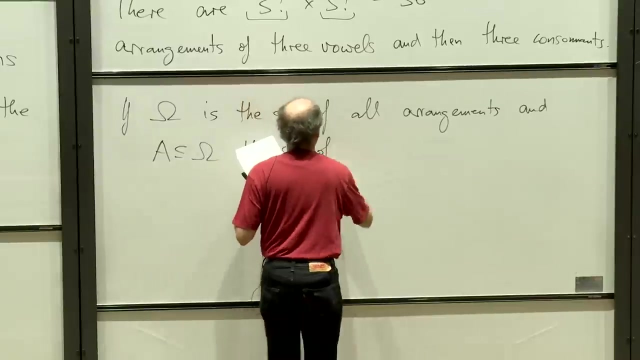 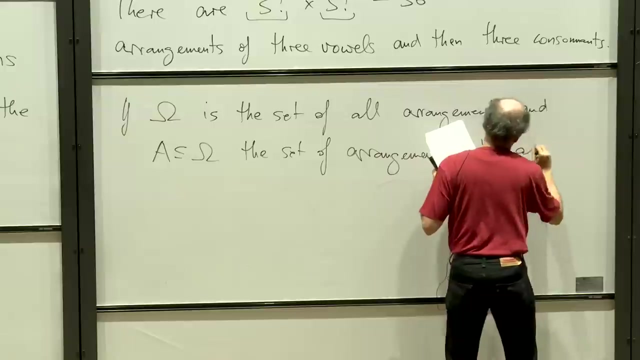 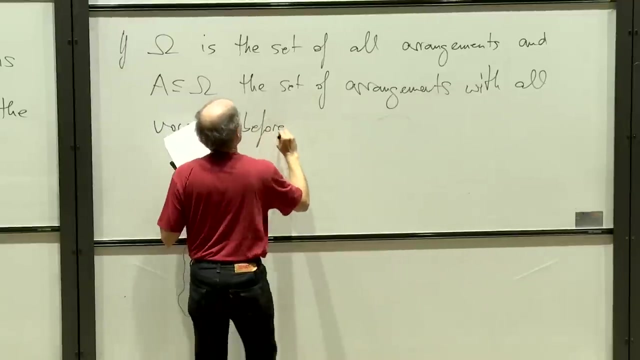 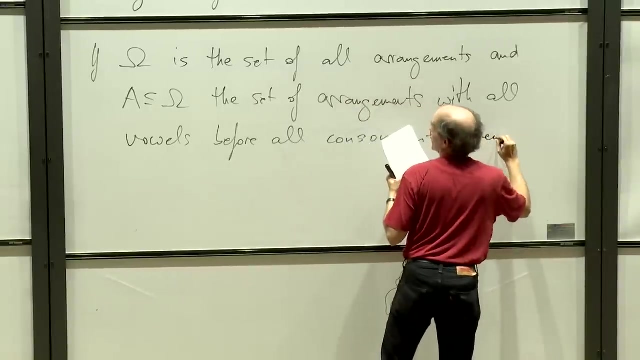 ad hoc calculations here. So let me maybe hook onto the notation a little bit better here. So if omega is the set of all arrangements and a subset of omega the set of arrangements with all vowels before, all consonants, then what I've calculated 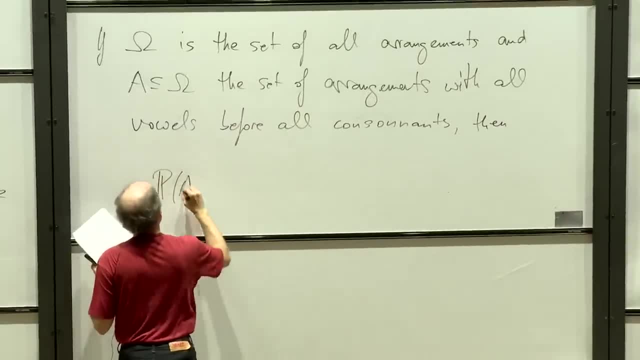 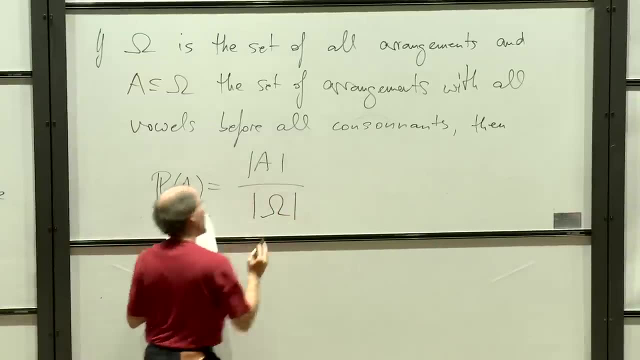 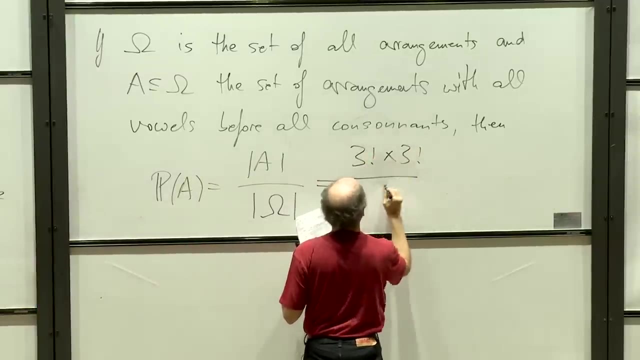 is that the probability of the event a, which, by definition, is the number of arrangements that have all vowels before all consonants, divided by the size of our sample space. well, that ratio now is three factorial times three factorial divided by six factorial. And if you work it out, 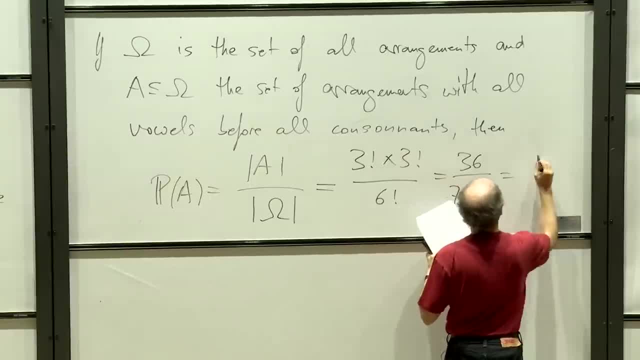 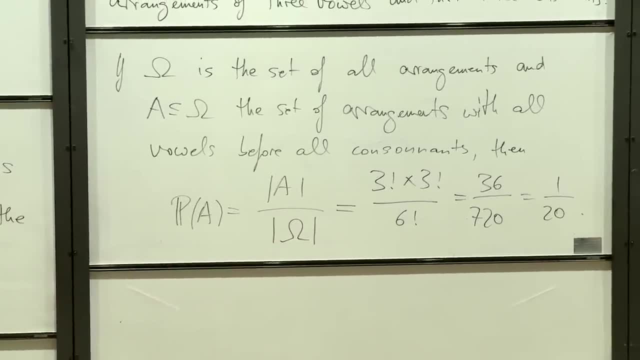 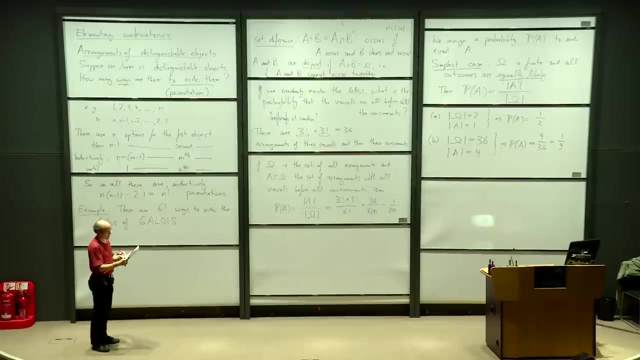 thirty-six divided by seven-twenty is one-twentieth. Okay, So you can try the same with some other words and, of course, if the number of vowels is different, then you get a different answer. Okay, So this was the simplest setting in which we can ask. 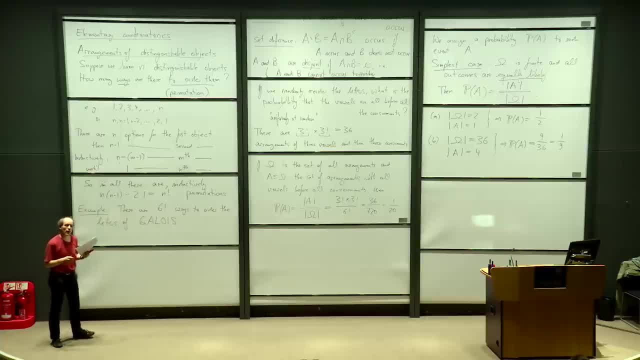 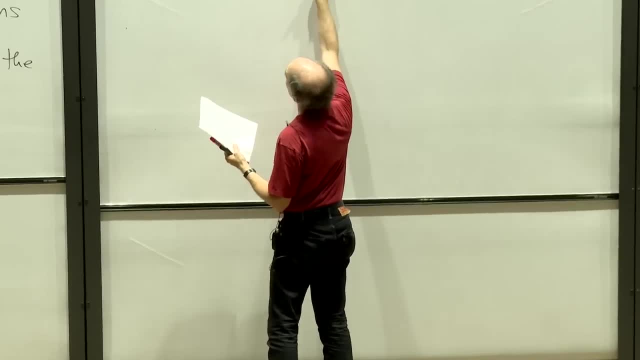 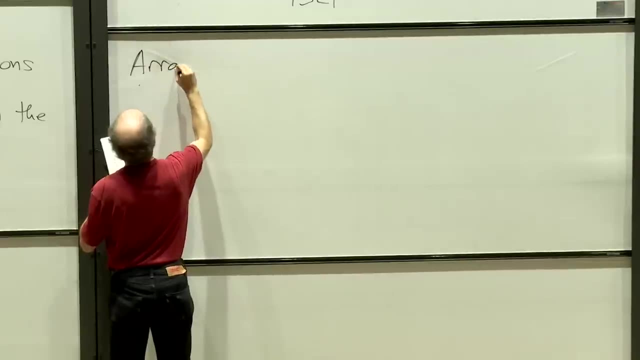 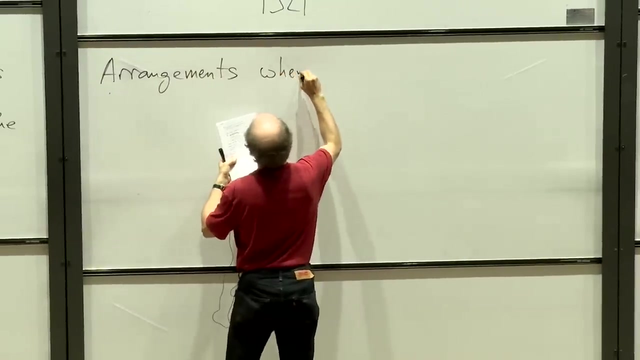 how many arrangements are there to order objects when all the objects are indistinguishable? So let me now move on to the more general task of finding out how many arrangements there are if not all objects are indistinguishable. So arrangements when not all objects. 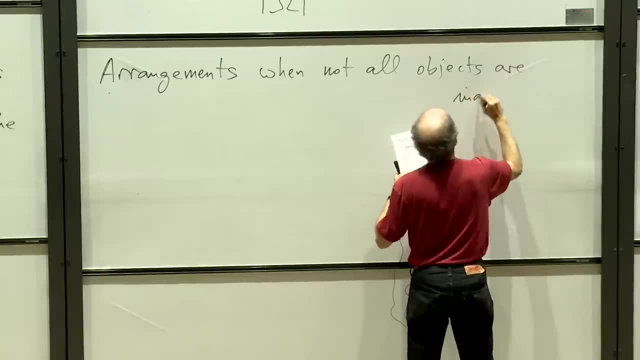 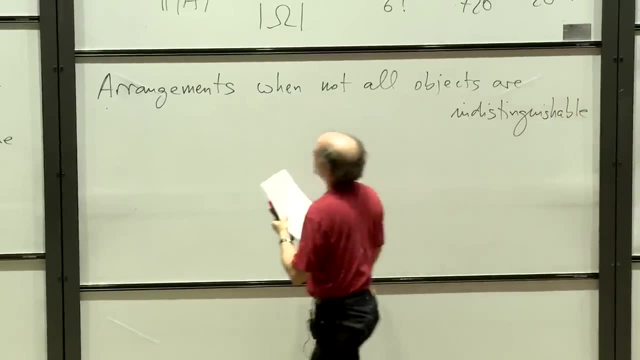 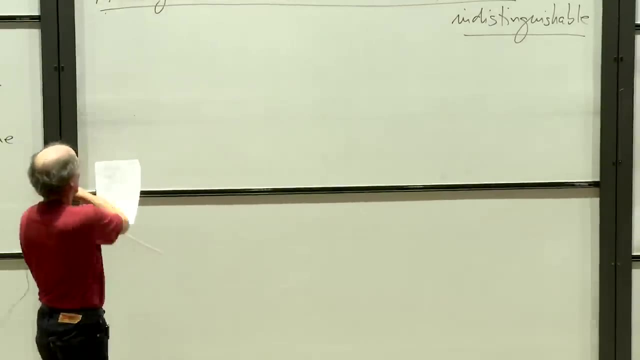 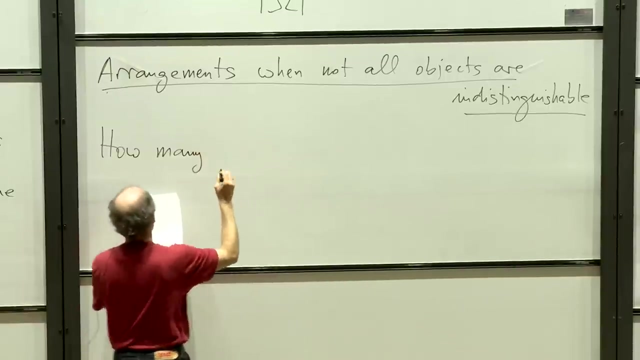 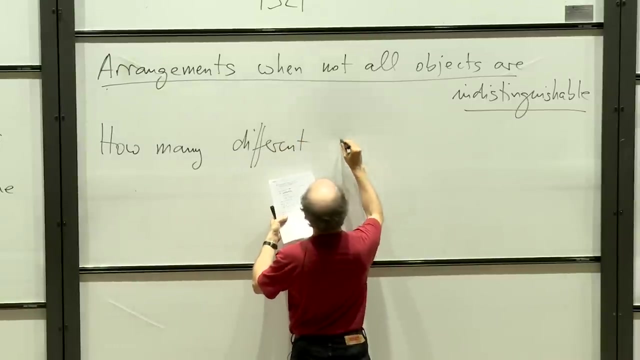 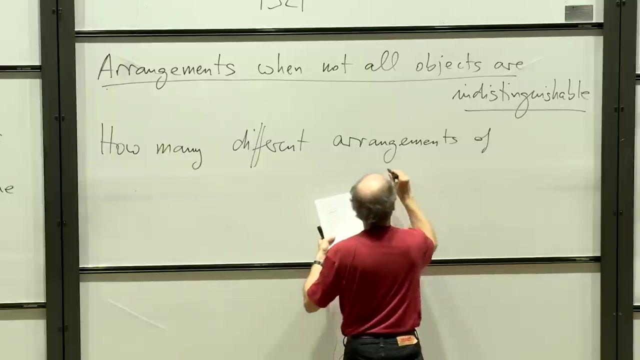 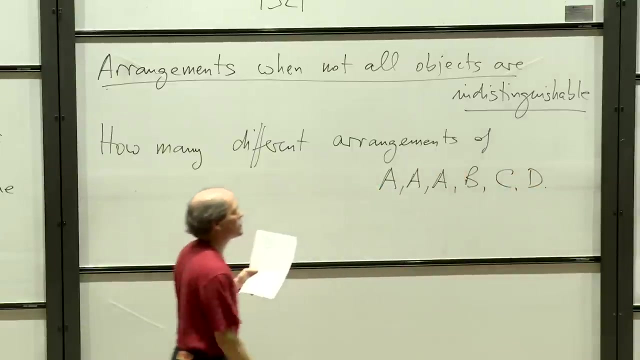 are indistinguishable. Okay, Let's start with an example. So how many different arrangements are there when I give you six letters? not all different. So different arrangements of A, A, A, B, C, D. So the letter A is repeated, We have three. 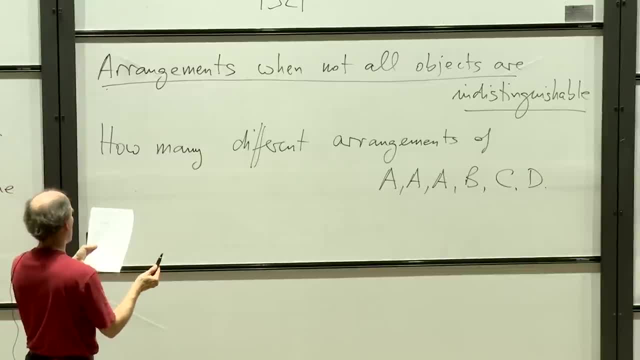 letters A and the other three are are distinguishable. So does this relate back in any way to the previous problem that we've solved? We can kind of make some slight modification and say, well, I've got A, A and A, but if I had three distinguishable? 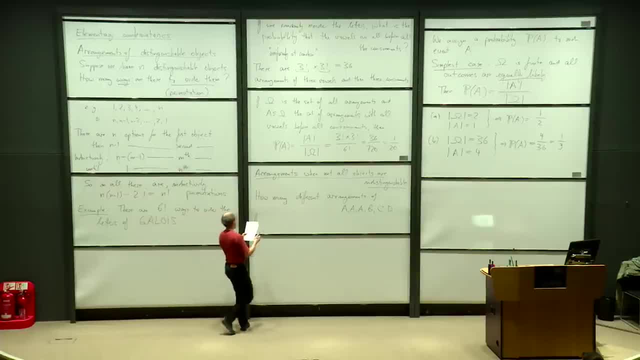 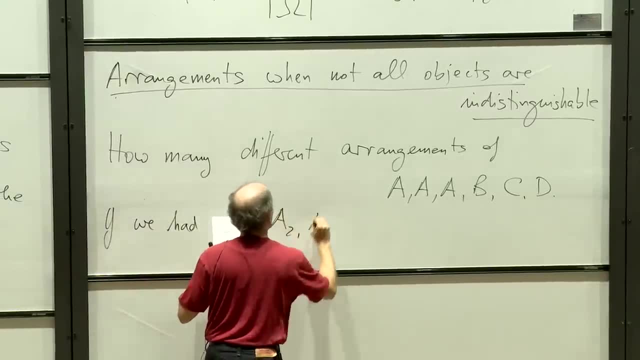 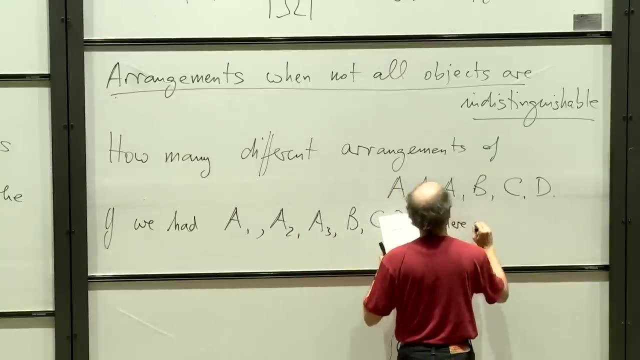 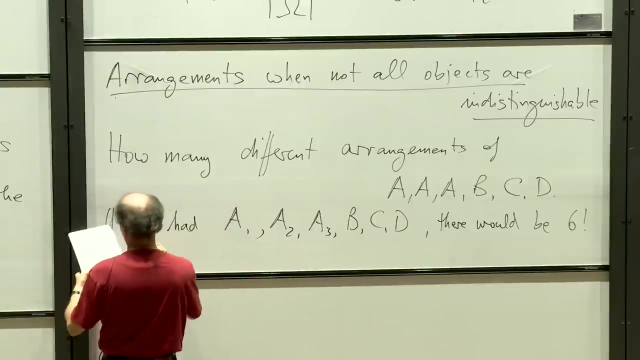 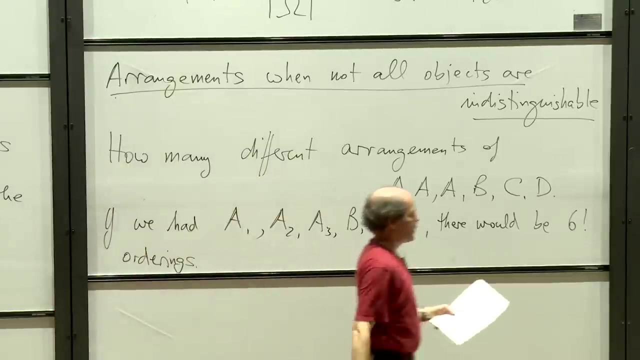 varieties of A, then I'd be back to the problem that I've already solved. So if we had A1, A2, A3, B, C, D, then there would be six factorial arrangements, six factorial arrangements or orderings. Okay, so what's different now? 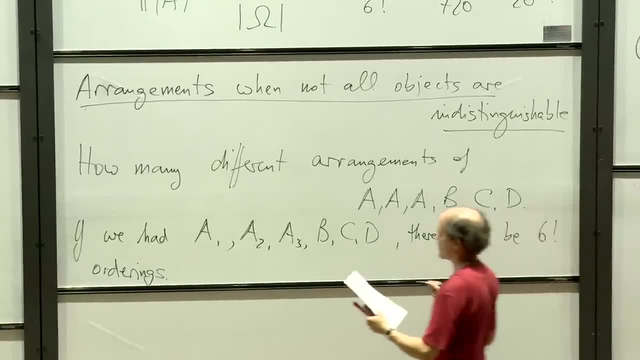 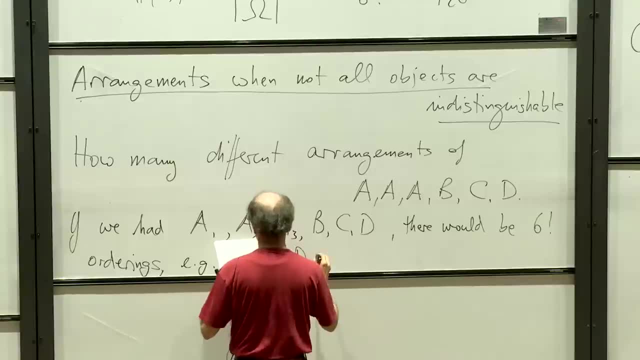 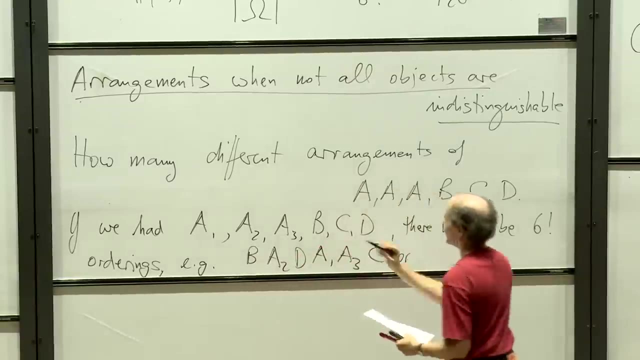 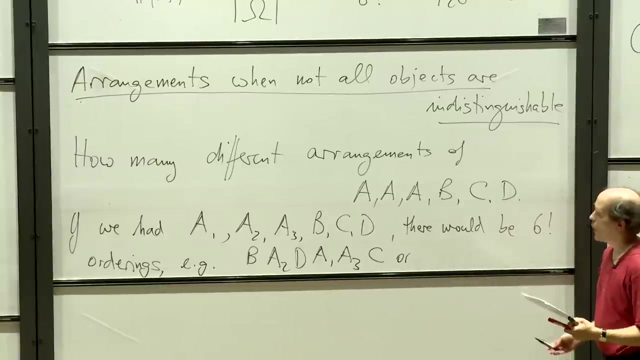 Well, we can kind of look at those. So let's look at some examples. For example, we can look at B, A2, D, A1, A3, C, or we could say, yes, but that's not the only way in which we can have B? A. 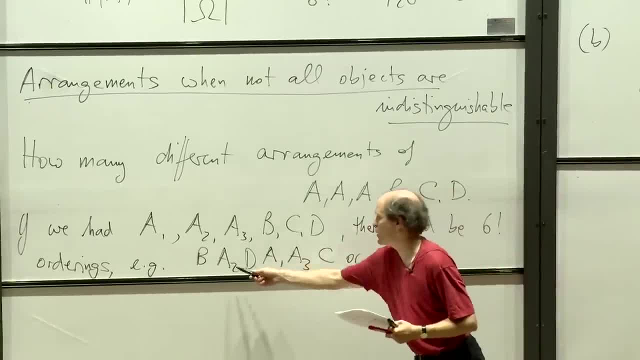 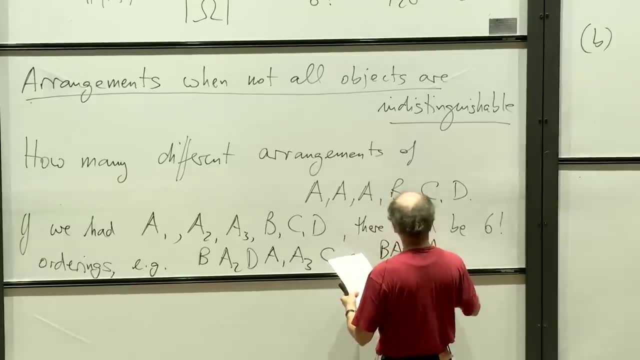 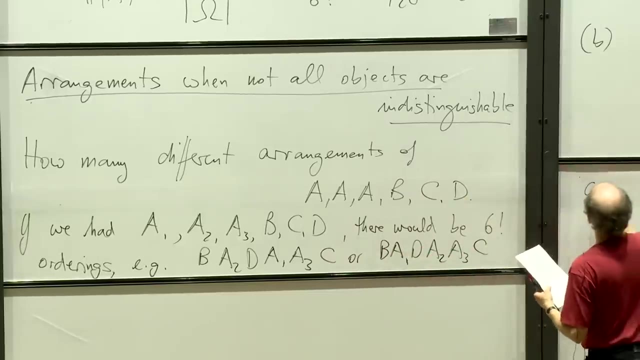 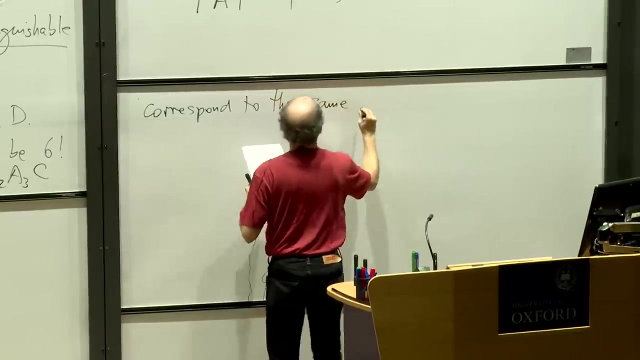 D, A, A, C. we can kind of have different indices to the A's, and another example is B, A1, D, A2, A3, C, right, So they correspond to the same: A1, D, A2, A3, A4, A5, A6, A7. 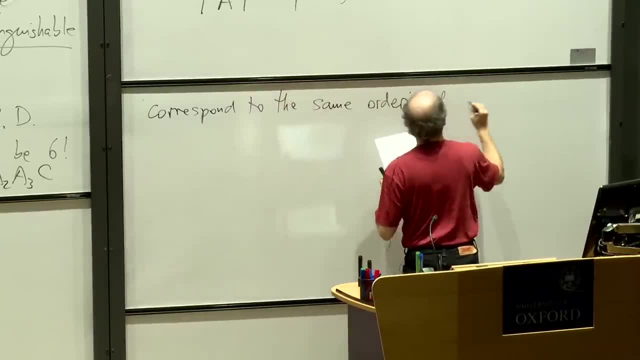 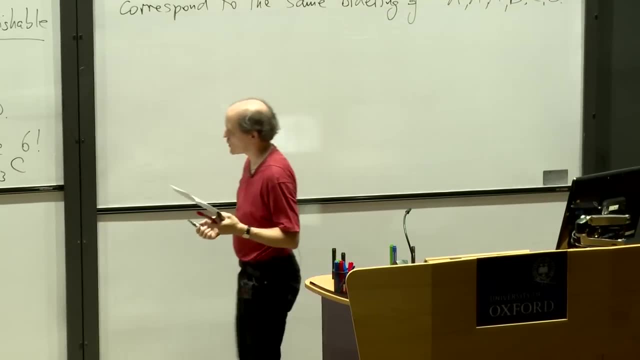 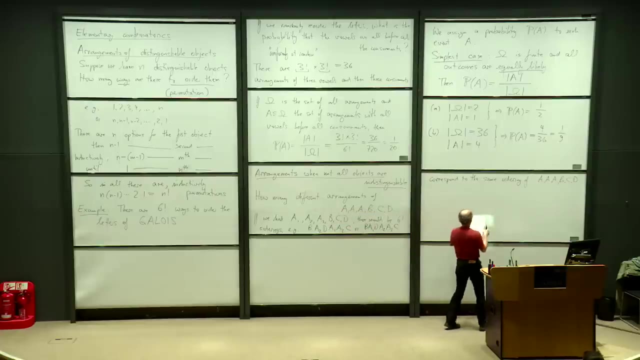 A8, A9, A10, A11, A12, A13, A14, A15, A16, A17, A18, A19, A20, A22, A23, A24, A25, A26, A27, A28, A29, A30, A31, A32, A33, A34. 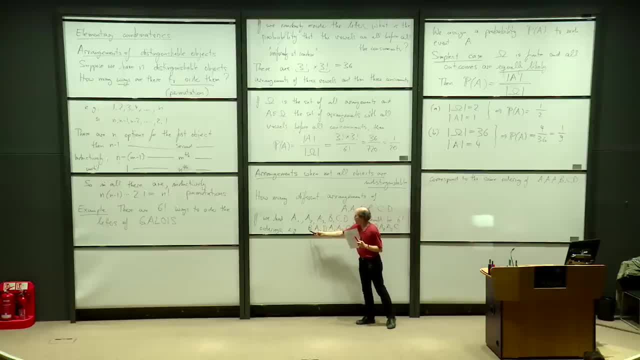 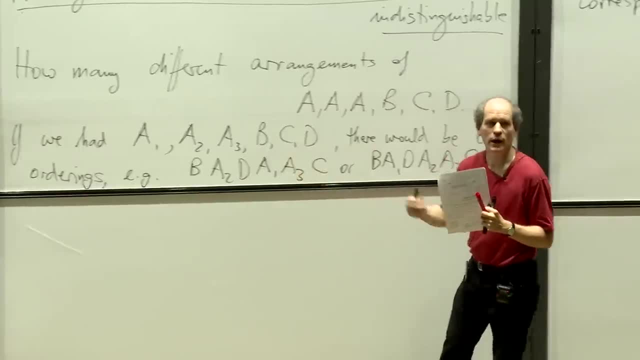 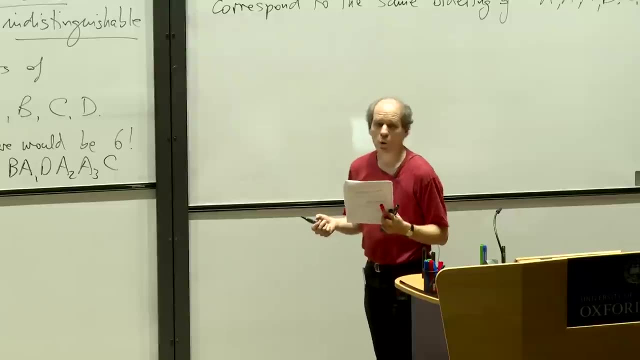 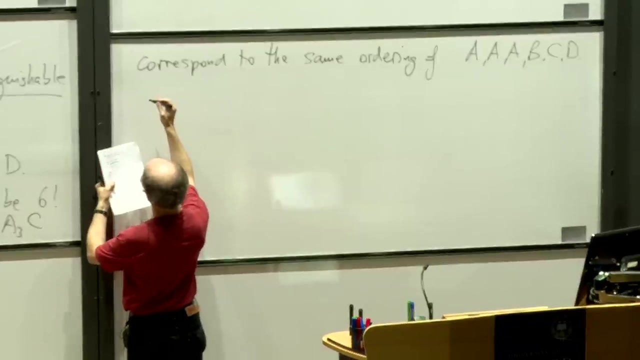 A36, A37, A40, A41, A42, A43, A45, A46, A47, A48, A49, A50, A51, A52, A53, A54, A56, A57, A18, A19, A19, A20, A21, A22, A23, A23. 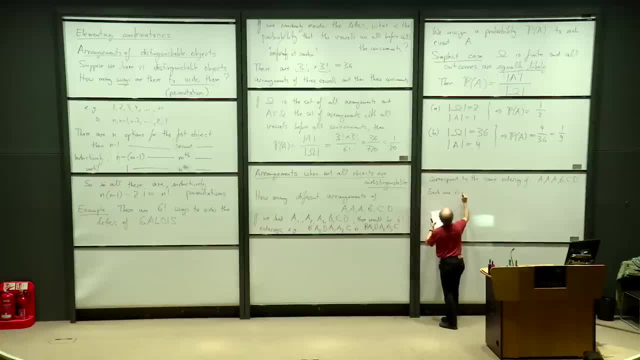 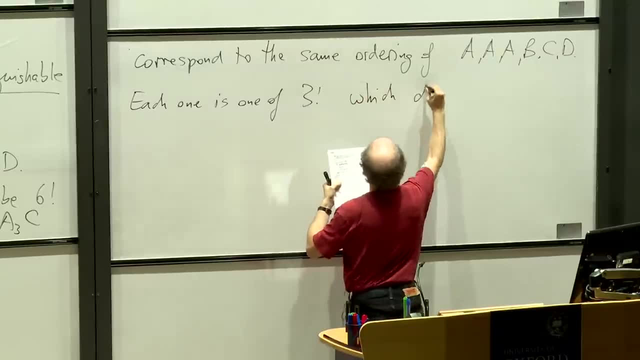 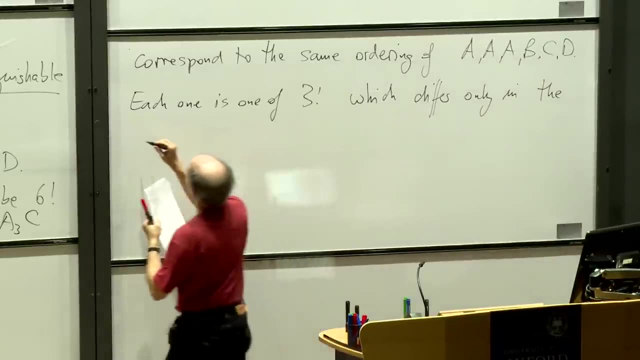 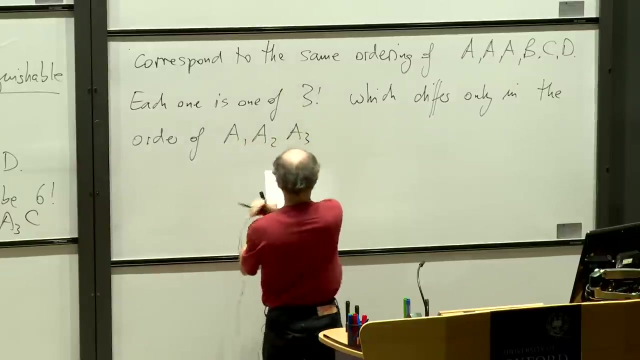 A24, A25, A26, A27, A28, A29, A30, A31, A32, A33, A34, A35, A36, A37, A38, A39, A40, A42, A43, A44, A45, A46, A47, A48, A49, A51. 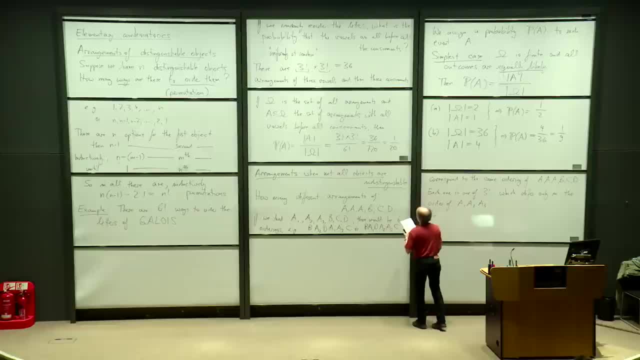 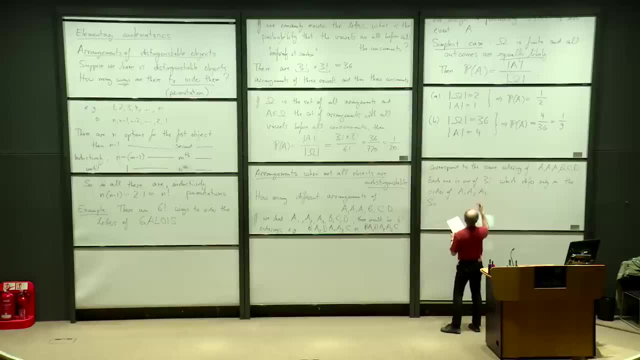 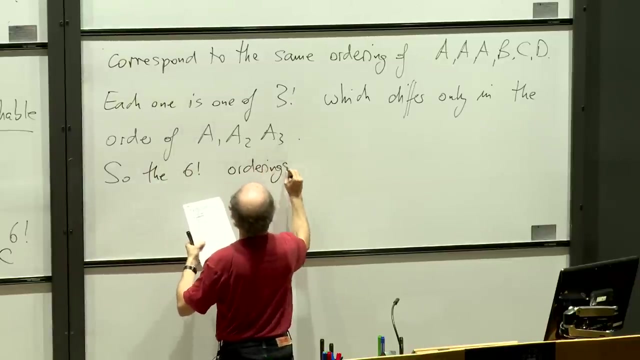 A52, A53, A54, A55, A56, A56, A57, A58, A59, A60, A61, A62, A63, A64, A65, A67, A68, A69, A70, A71, A72, A72, A73, A74, A74, A75. 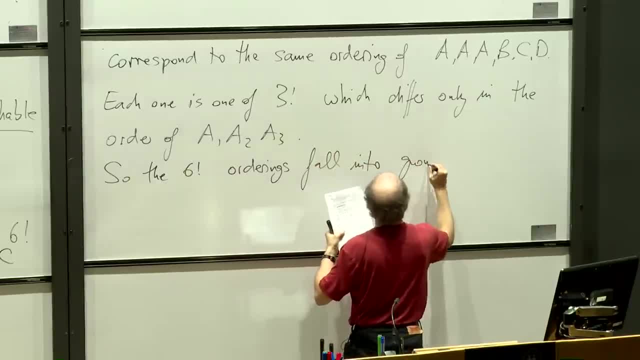 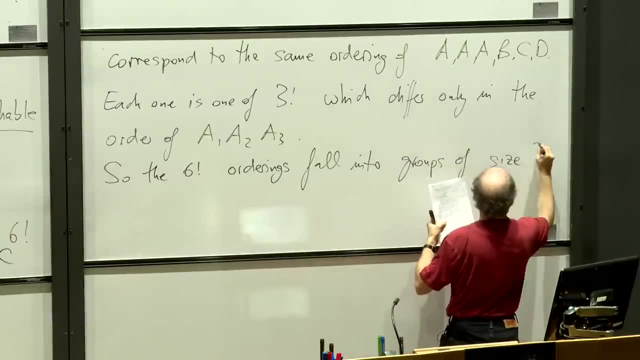 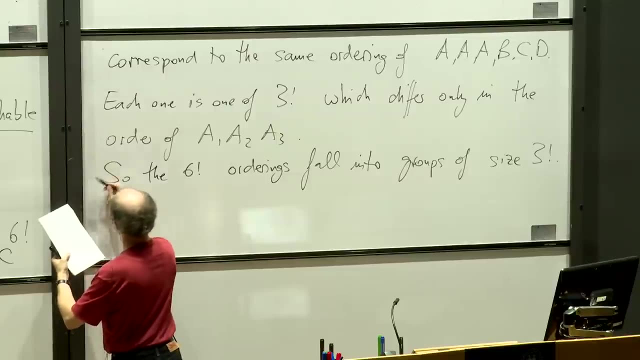 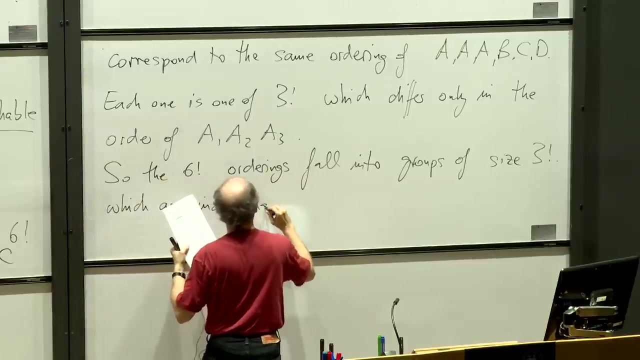 A78, A78, A19, A19, A21, A22, A23, A24, A24, A25, A26, A27, A28, A29, A31, A32, A33, A34, A36, A37, A38, A39, A41, A42, A43, A44. 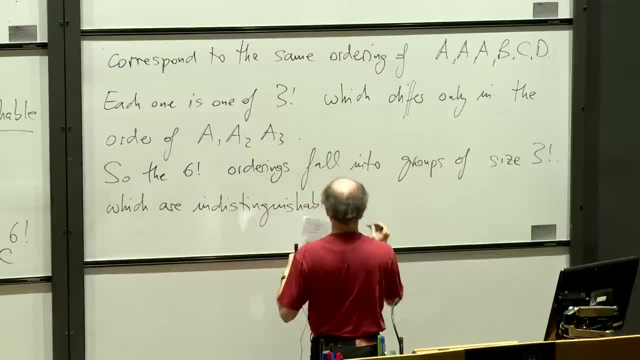 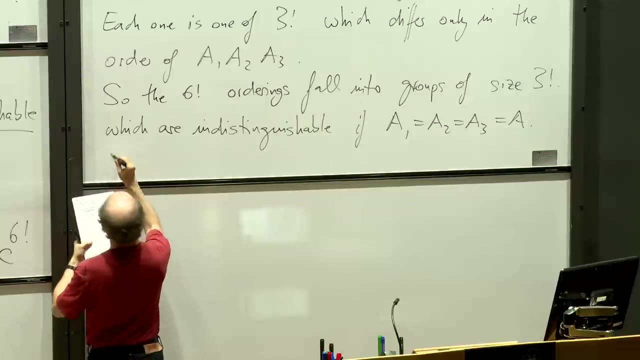 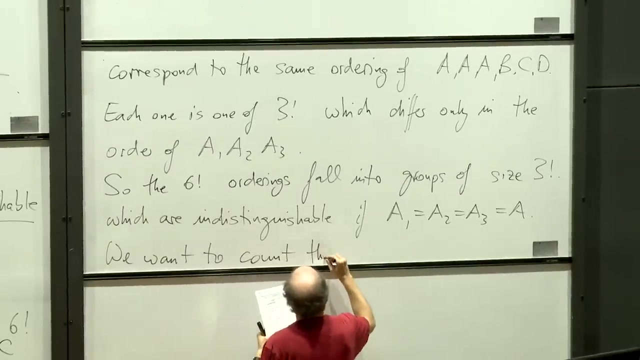 A45, A46, A47, A48, A49, A50, A51, A52, A53, A53, A54, A55, A56, A57, A58, A59, A60, A61, A62, A63, A64, A65, A67, A68, A69, A70. 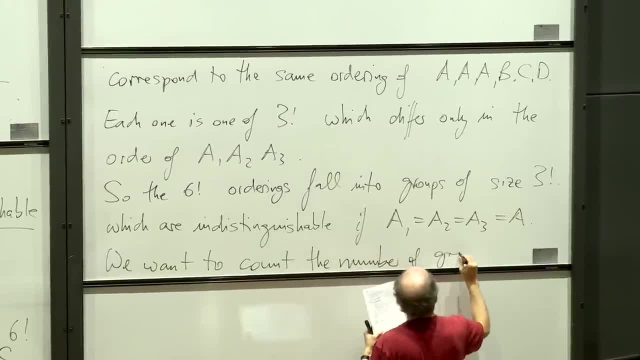 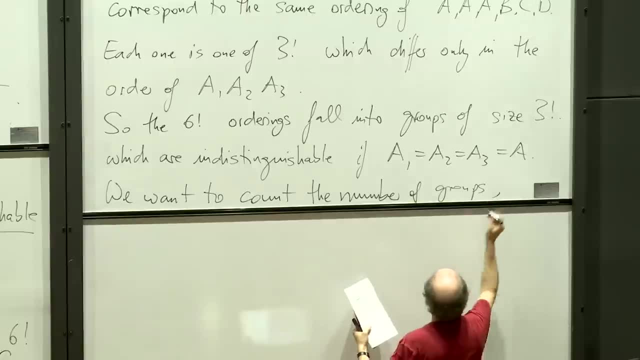 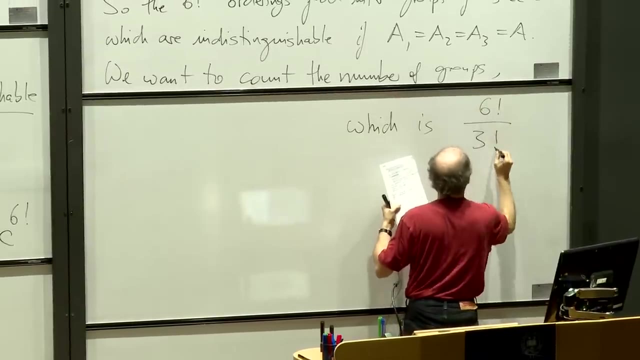 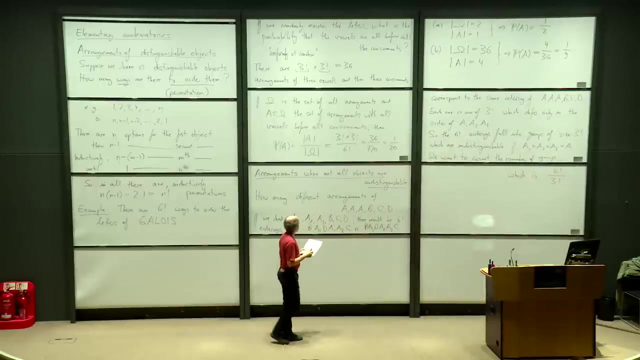 A71, A72, A72, A73, A73, A74, A74, A75, A78, A78, A78, A19, A19, A21, A22, A23, A24, A25, A26, A27, A28, A29, A30, A31, A32, A33. 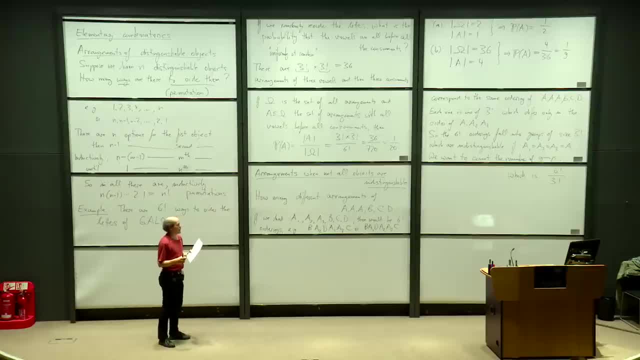 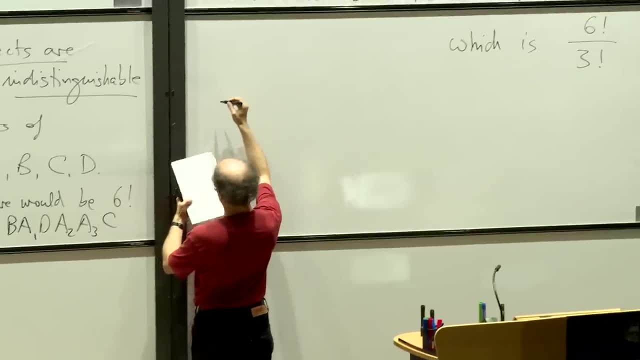 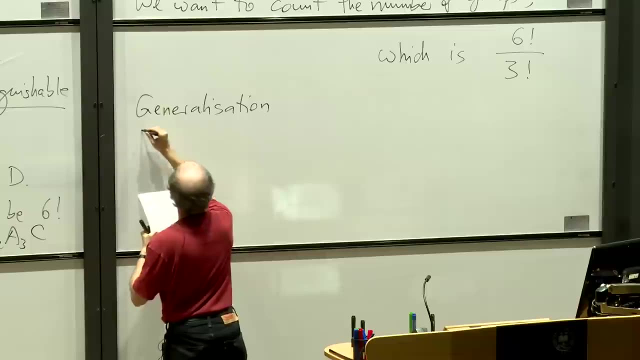 A33, A34, A35, A36, A36, A37, A38, A39, A40, A42, A43, A45, A46, A47, A48, A49, A50, A51, A52, A53, A53, A54, A55, A56, A57, A58. A59, A60, A61, A62, A63, A64, A65, A67, A68, A68, A69, A70, A71, A72, A71, A72, A72, A73, A73, A74, A74, A75, A78, A78, A71, A72. A72, A73, A78, A72, A73, A74, A78, A78, A71, A71, A72, A72, A72, A73, A74, A74, A75, A78, A78, A78, A78, A19, A19, A20, A21, A22. 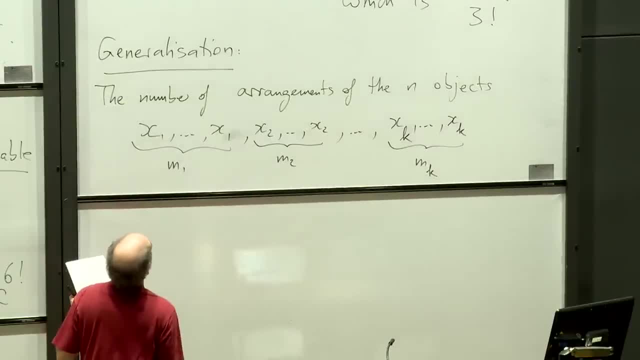 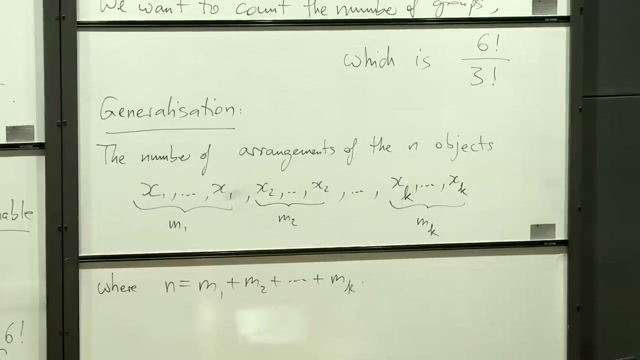 A23, A24, A25, A26, A27, A28, A29, A30, A31, A32, A33, A34, A35, A36, A37, A38, A39, A41, A42, A43, A44, A45, A46, A47, A48, A49. A51, A52, A52, A53, A54, A55, A56, A57, A58, A59, A60, A61, A62, A63, A64, A65, A67, A68, A69, A70, A71, A72, A72, A73, A74, A74. 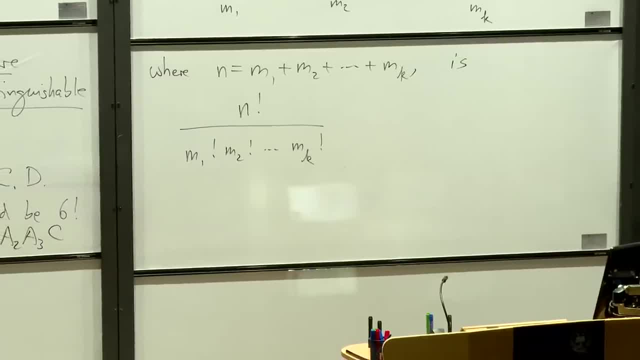 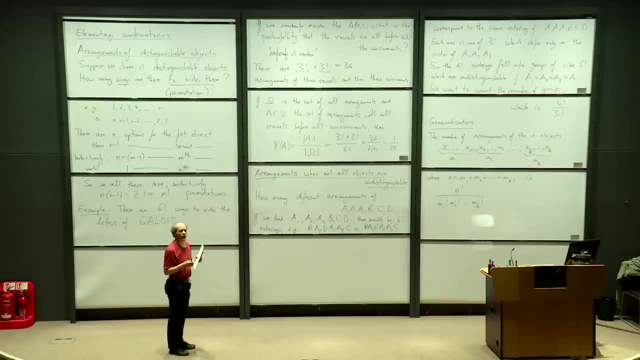 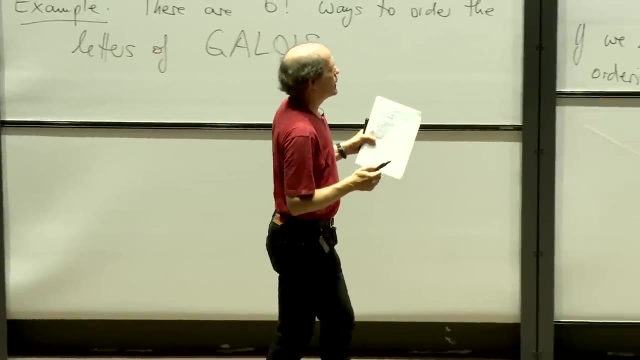 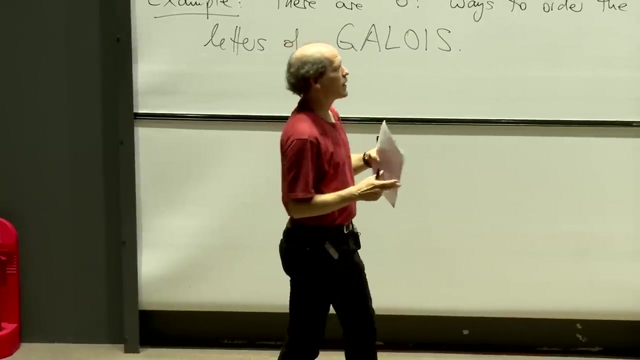 A75, A76, A78, A79, A79, A80, A80, A90, A21, A22, A23, A24, A25, A26, A27, A28, A29, A31, A32, A33, A34, A35, A36, A37, A38, A39. 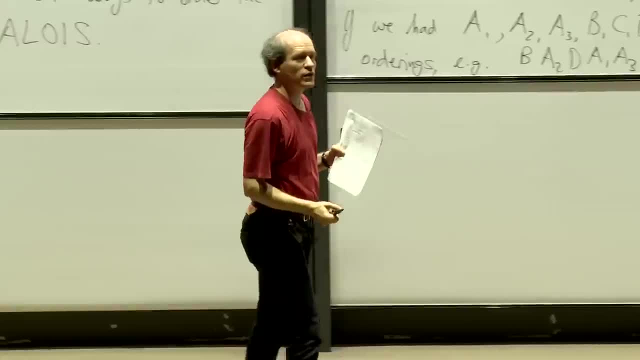 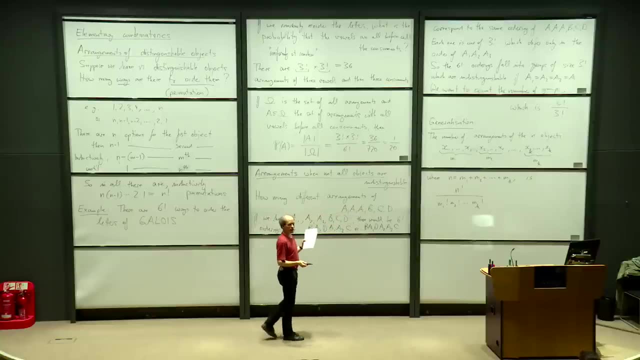 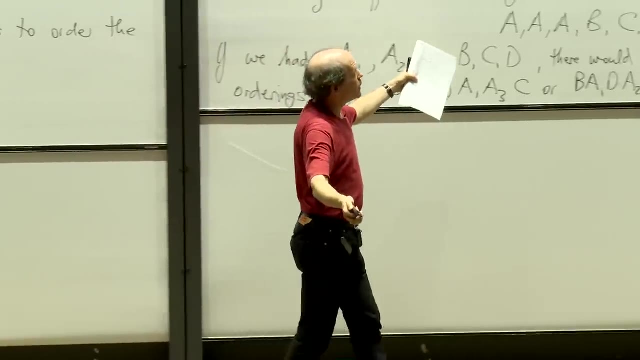 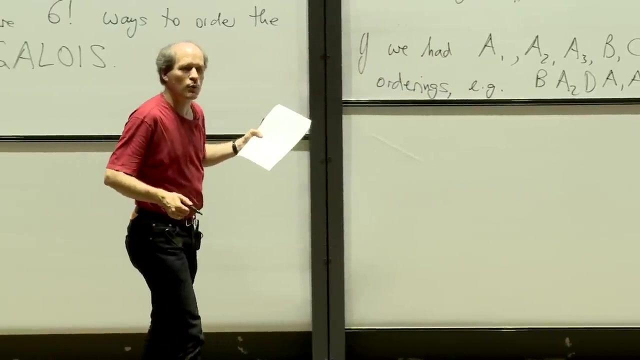 A40, A41, A42, A43, A44, A45, A46, A47, A48, A49, A50, A51, A52, A53, A54, A55, A56, A57, A58, A59, A60, A61, A62, A63, A63, A64. 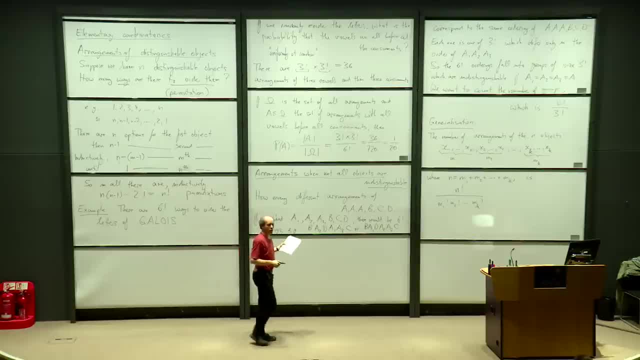 A65, A67, A68, A69, A70, A71, A72, A72, A73, A73, A74, A74, A75, A75, A78, A78, A78, A79, A19, A20, A21, A22, A23, A24, A25, A26. 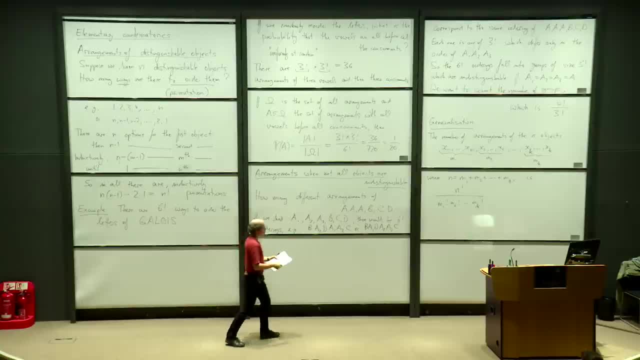 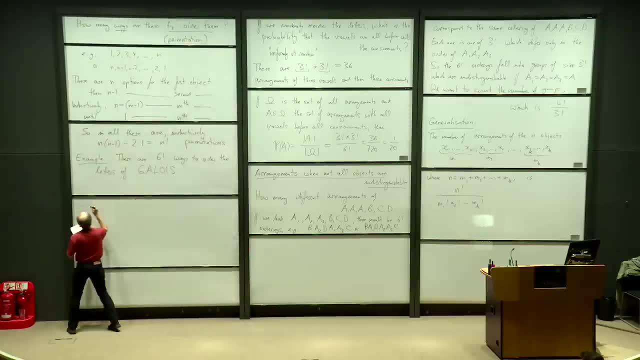 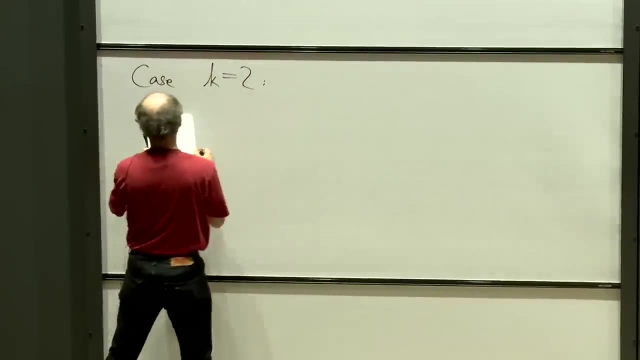 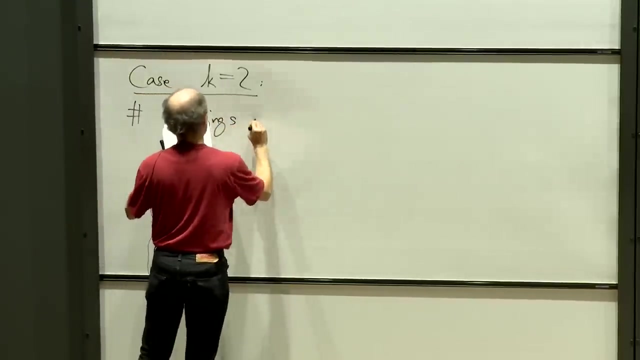 A27, A28, A29, A30, A31, A32, A33, A34, A35, A36, A36, A37, A38, A39, A41, A42, A43, A43, A45, A46, A47, A47, A48, A49, A51, A52. A53, A54, A55, A56, A57, A58, A59, A60, A61, A62, A63, A64, A65, A67, A68, A69, A70, A71, A72, A72, A73, A73, A74, A74, A74, A75. A78, A78, A78, A79, A80, A72, A72, A73, A74, A72, A74, A75, A78, A78, A78, A79, A19, A20, A21, A22, A23, A24, A25, A26, A27, A27. 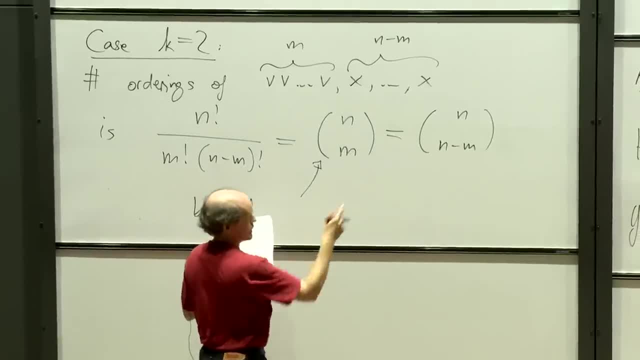 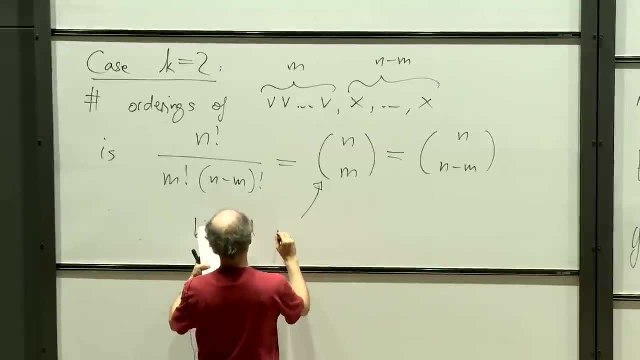 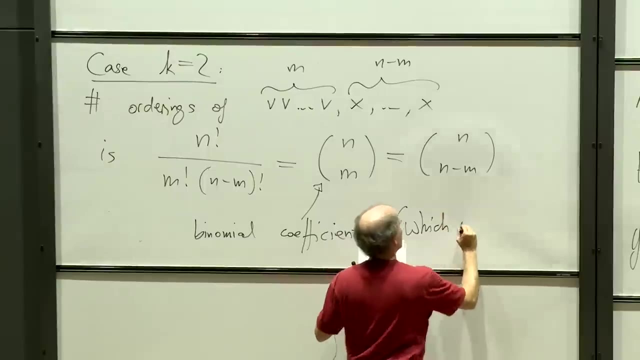 A27, A28, A29, A30, A31, A32, A33, A34, A35, A36, A37, A38, A39, A40, A41, A42, A43, A44, A45, A46, A47, A48, A49, A50, A51, A52. 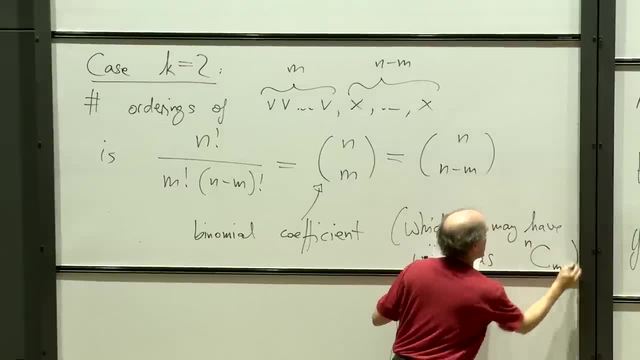 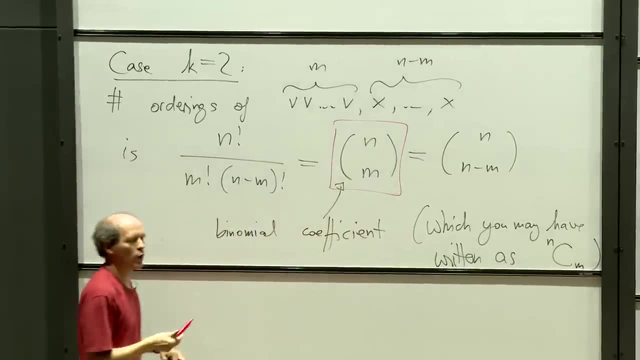 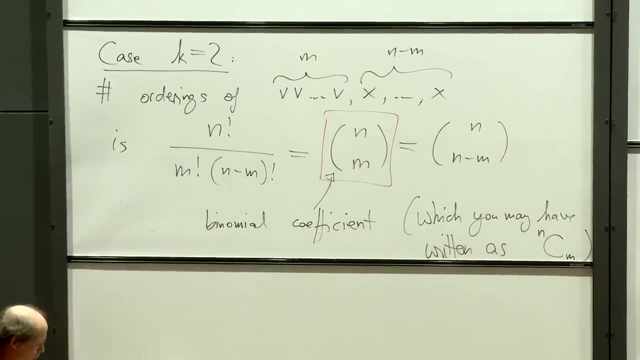 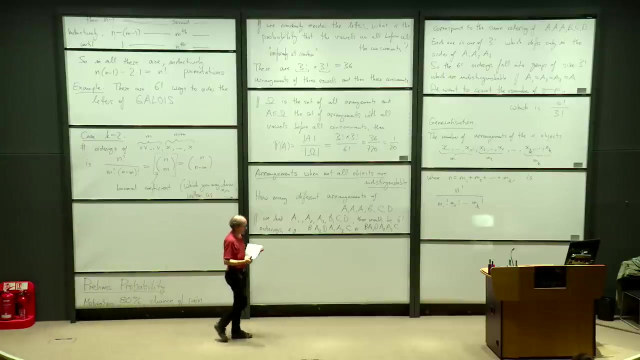 A53, A54, A55, A56, A57, A57, A58, A59, A30, A32, A33, A34, A35, A36, A37, A38, A39, A41, A42, A43, A43, A44, A45, A46, A47, A48.